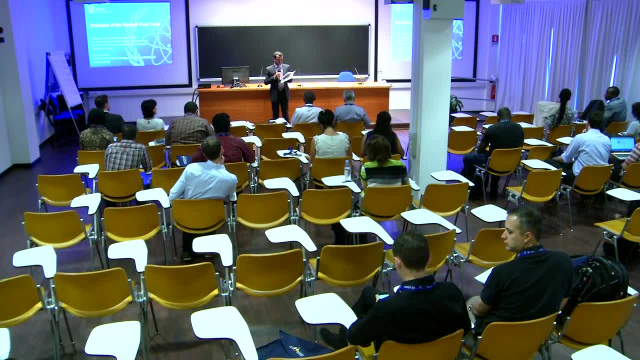 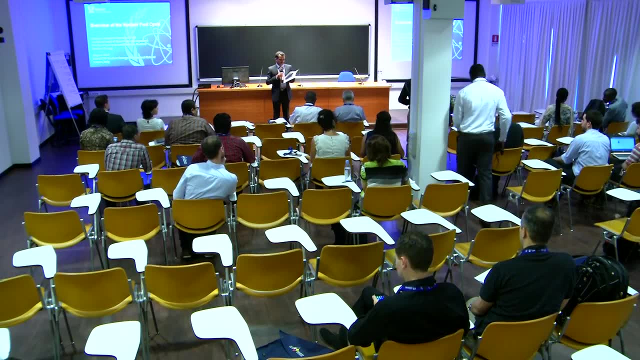 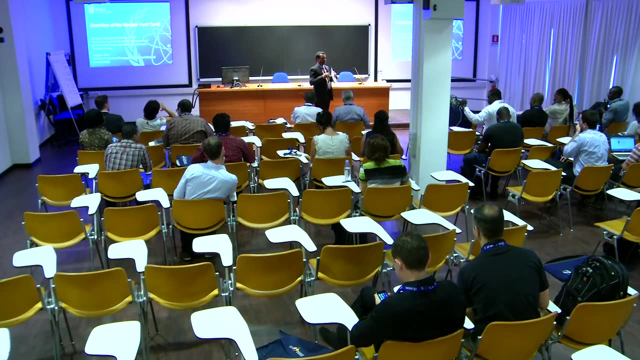 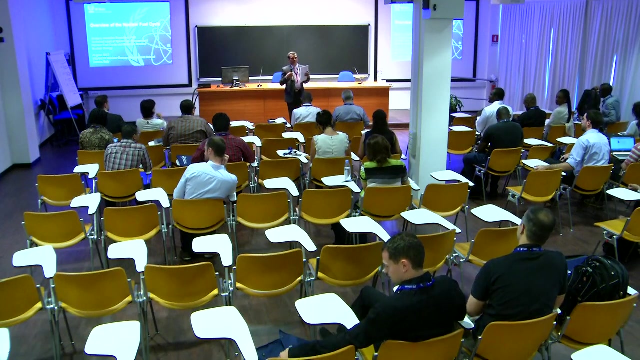 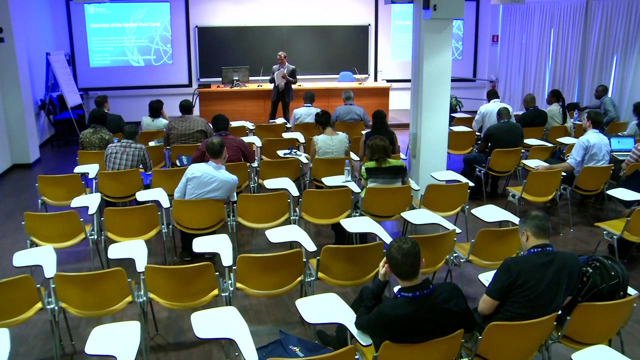 unique to an IAEA. It's a good location. He's doing a lot of helps. We do talk as good as any very interesting sessions with Sean in the afternoon. the morning sessions will be from Amparo, so I will hand over to Sean to take over the today's. 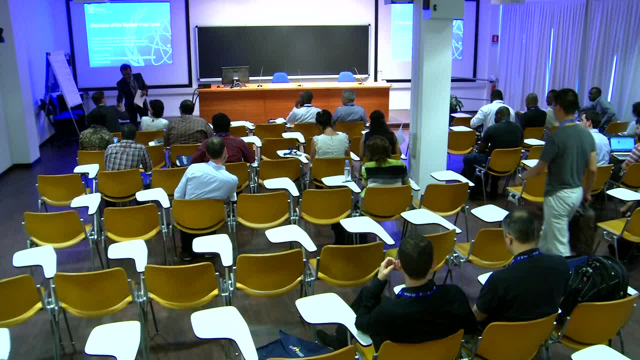 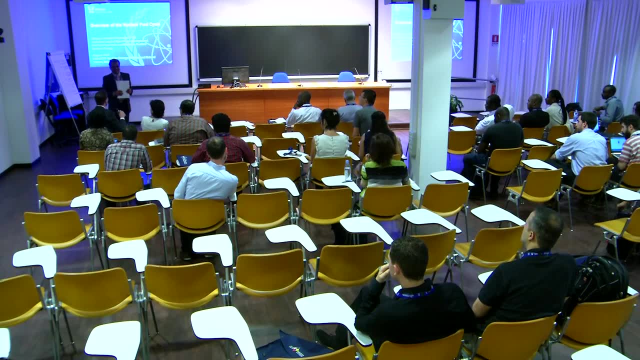 proceedings. Sean, please thanks. good morning everybody. I look forward to getting to know you a little bit better over the next couple days and, without further ado, I think I'll hand things over to Amparo. so good morning. I'm Amparo González Espartero. I'm the technical lead of the Spain fuel. 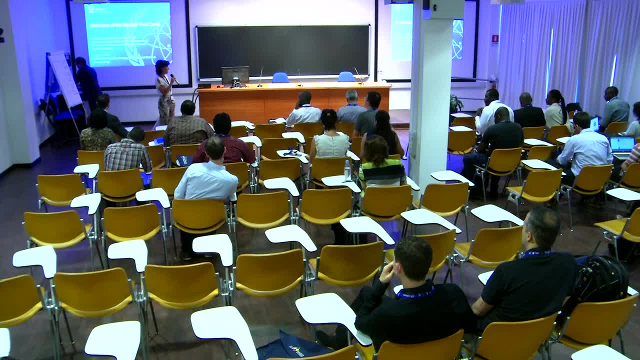 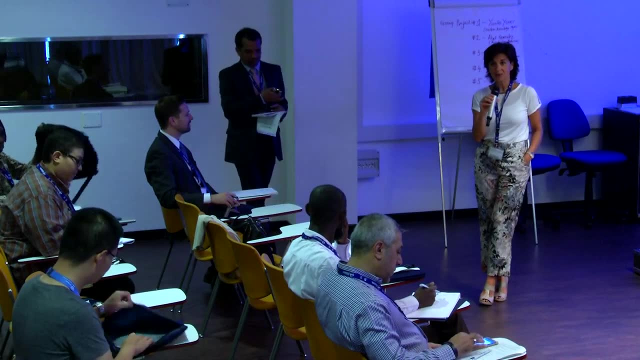 management in the nuclear fuel circular material section in the INC, and I joined the INC in 2015 and I was working previously for 24 years in the Spanish nuclear lab national lab, who, which supports EMRESA, who is the organization in charge of the radioactive waste management in Spain. 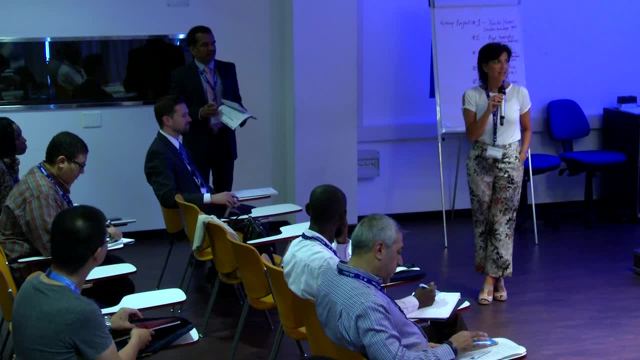 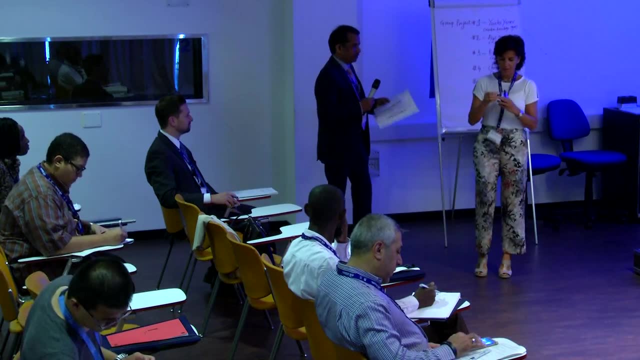 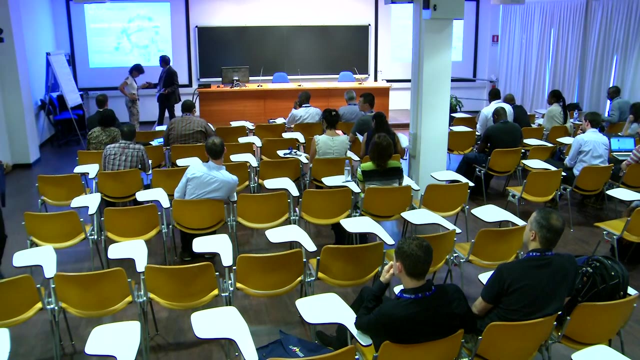 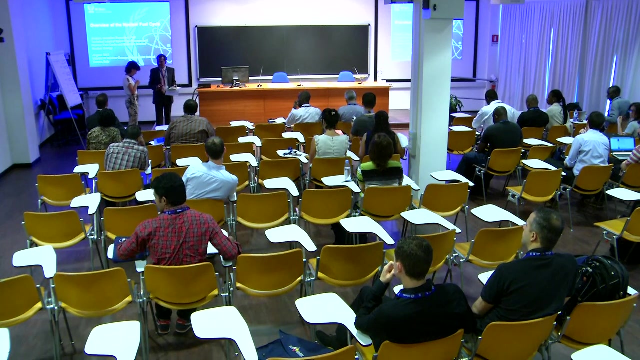 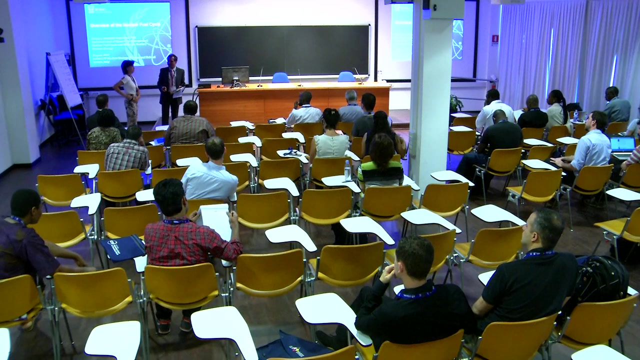 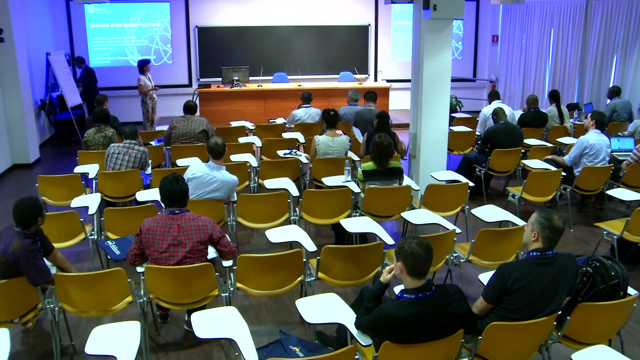 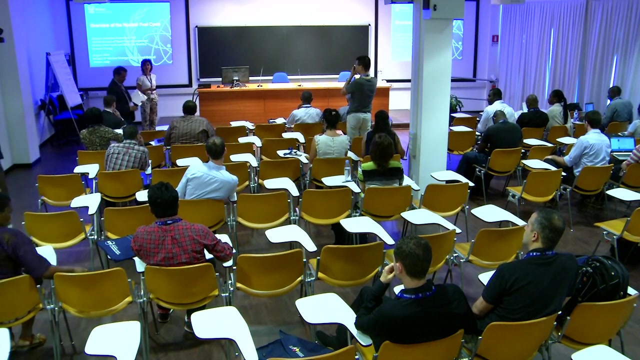 and also our regulatory body. so Should I? okay, I think you need to switch it on. Hello, so, as Ashok said, I was asked to give a presentation, an overview of the nuclear fuel cycle, and the second lecture I'm going to give is about radioactive waste management and the commissioning. 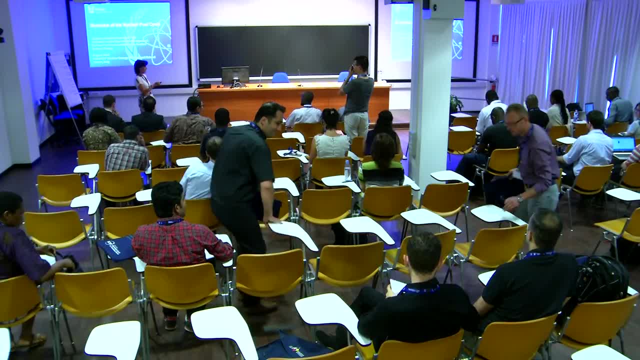 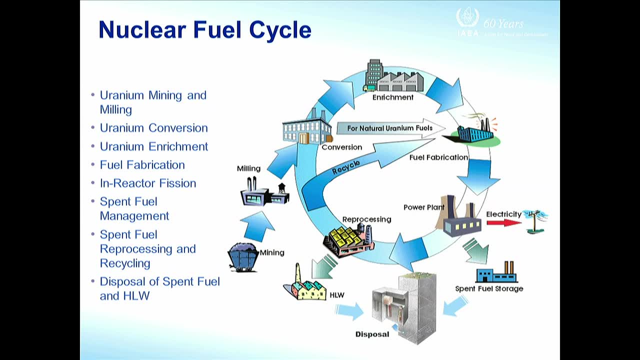 So this presentation I will try, I will try to give you an overview of the main stages of the nuclear fuel cycle and we can talk about, since we are going to talk about radioactive waste after the related waste produced in every stage. 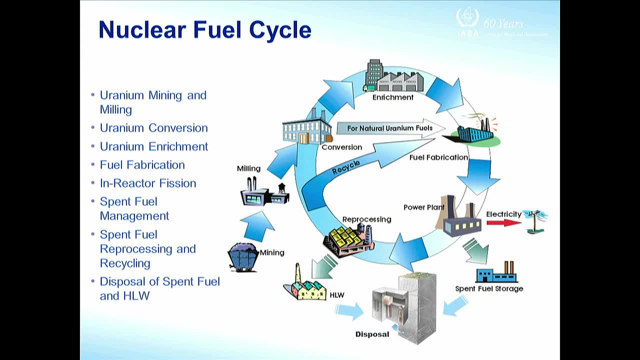 So I think that we can let the questions for the end of the presentation, because sometimes I'm going to address some issues in the course of the lecture. So the nuclear fuel cycle are the main industrial stages involved In the nuclear electricity production from nuclear power. 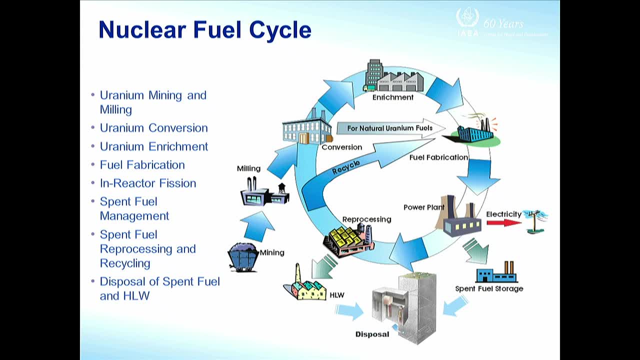 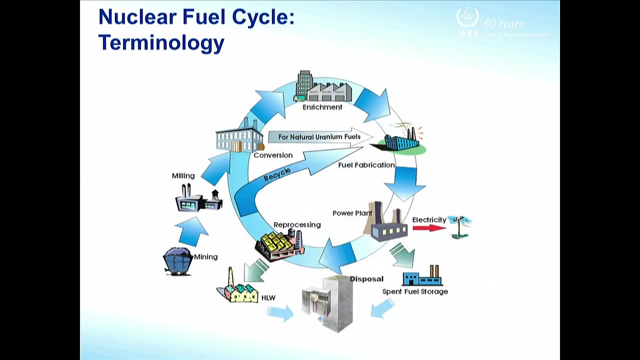 And it starts by the exploration of uranium mining and milling and ends with the eventual disposal of the waste produced, The nuclear fuel cycle terminology. There are the stages. This is covering mining, milling, the conversion of the uranium to put it in a right form to be used as fuel. 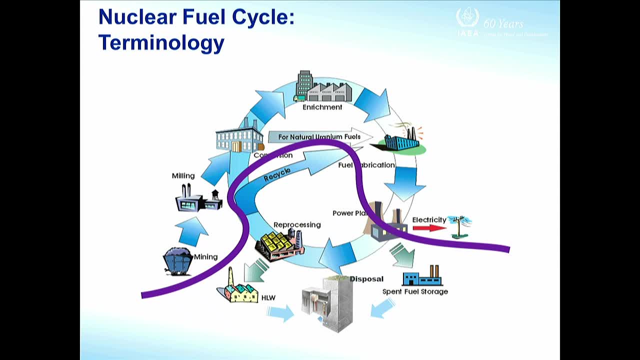 The enrichment for different types of reactors of uranium And the fuel fabrication are called the front end of the fuel cycle And then after the electricity production. I don't know if I have a list. Ah yeah, The fuel has to be discharged from the core after more or less three years in the core of the reactor. 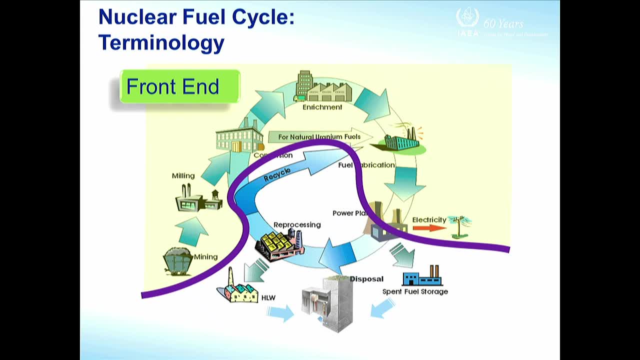 And has to be stored or reprocessed to recycling uranium and plutonium, But producing a high level waste stream that has to be managed with the same criteria as the spent fuel And has to be disposed in the deep geological repository. And these stages are called the back end of the fuel cycle. 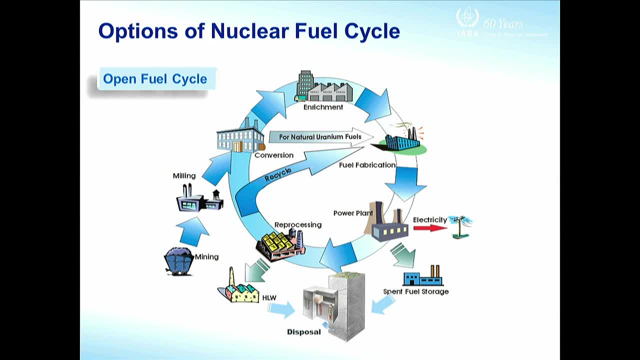 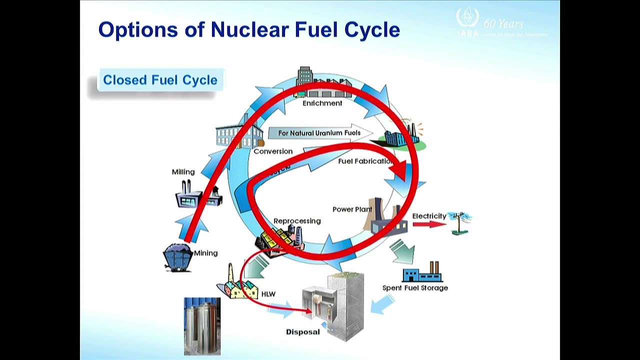 There are different options for the fuel cycles And so far there are two options commercially available. One is the fuel cycle, which consider the spent fuel as a waste, So after a period of storage has to be disposed in the geological repository. And the second option is the so called closed fuel cycle or one through cycle. 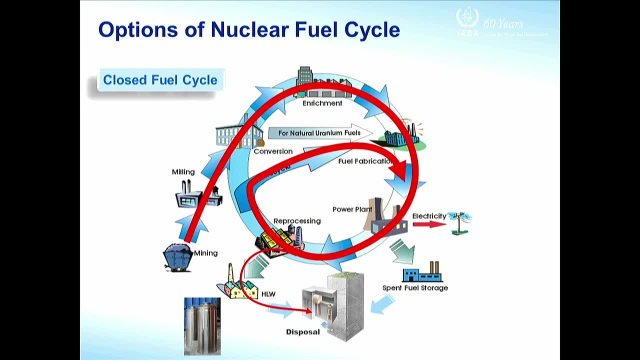 And is the mono recycling of plutonium. So so far, the spent fuel after a period of storage is reprocessed To recover uranium and plutonium, producing mux fuel. that is burned in reactors, But only one time, So once is discharged from the reactor is stored. 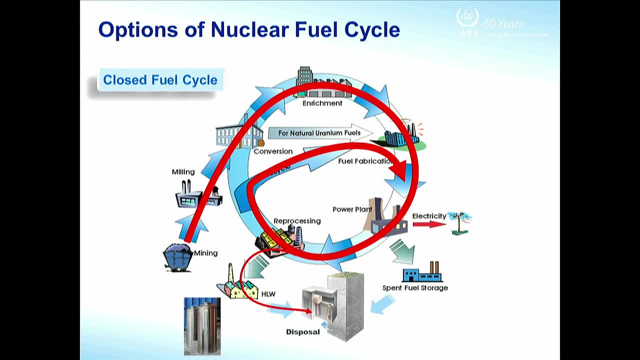 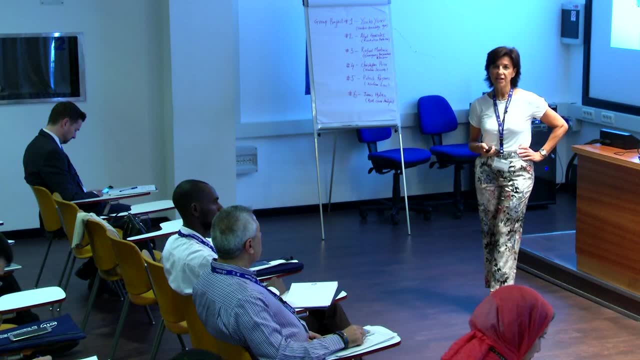 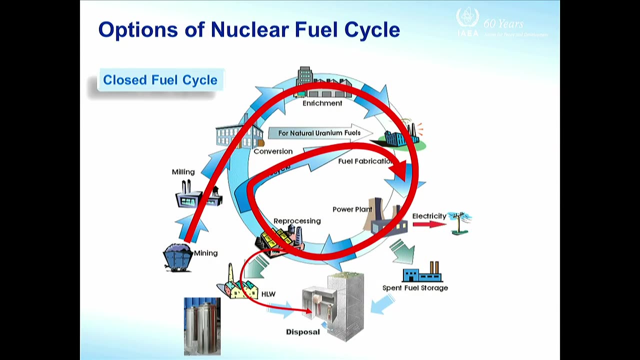 The mux fuel is stored for further use And so far is stored to be used in fast reactors. So France is the main country producing irradiated mux fuel And in this case is produced a high level waste stream That has is vitrified, arbitrified. 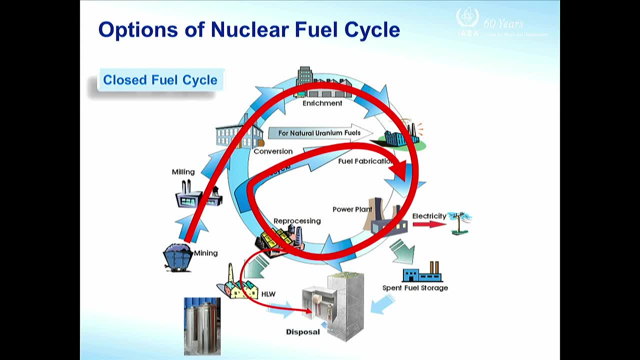 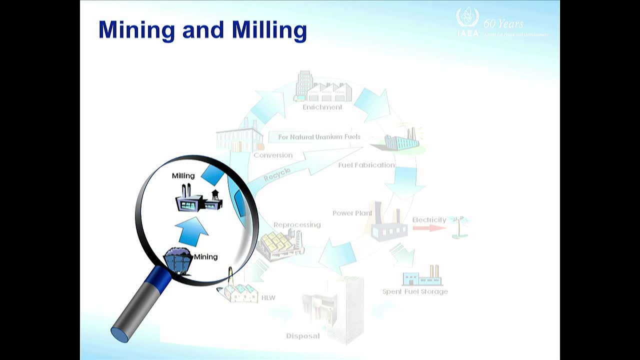 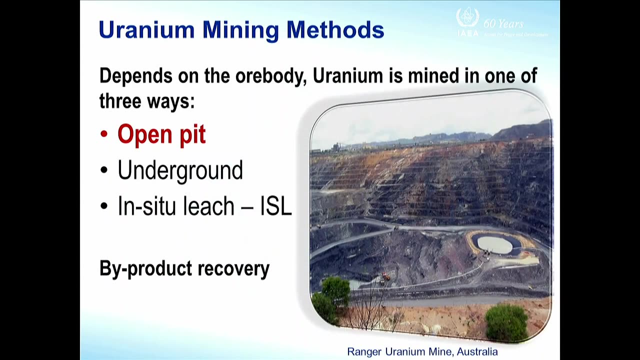 And then has to be stored also in the deep geological repository. So there are two main fuel cycle options. So if we start step by step, Let's talk about mining and milling. So it depends on where the ore body is. There are three options for to get uranium from the earth. 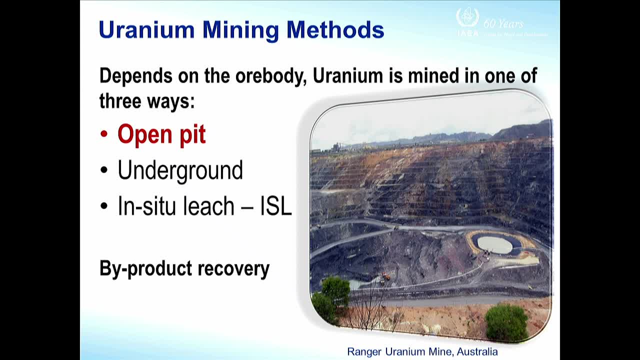 One is the open pit, underground or in situ leach, And also there is another option That consists to recover uranium from natural rocks as the fertilizers, And it's called byproduct recovery, So when the ore body is close to the surface. 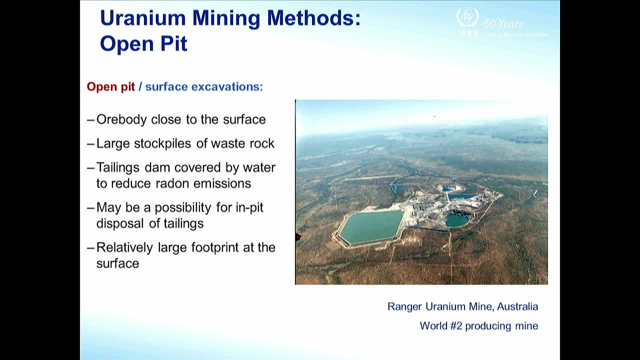 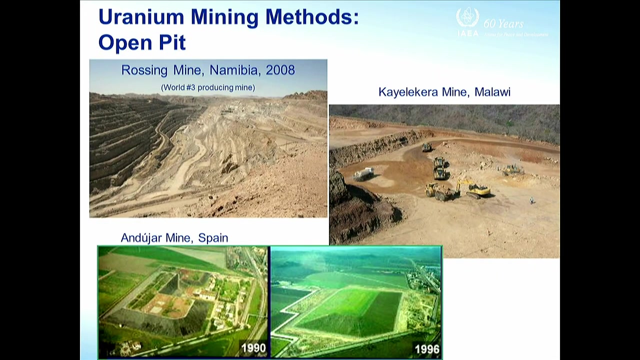 The open pit is the mining option And in this case it's produced a huge amount of barren rock And because the pit has to be big enough, Bigger than the ore, Because it's mined in a slope To prevent collapse. So, as you can see, there is a lot of surface disturbance. 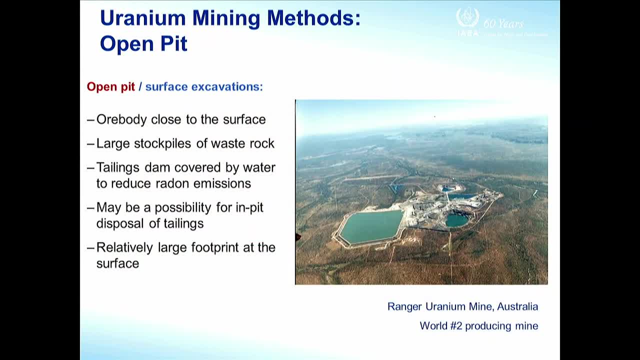 In this type of mining. So the rock produced, the barren rock, has to be put under water To prevent the natural radiation, Because, you know, the uranium is everywhere And the radon, the emissions of radon, are very common, And to prevent these emissions, 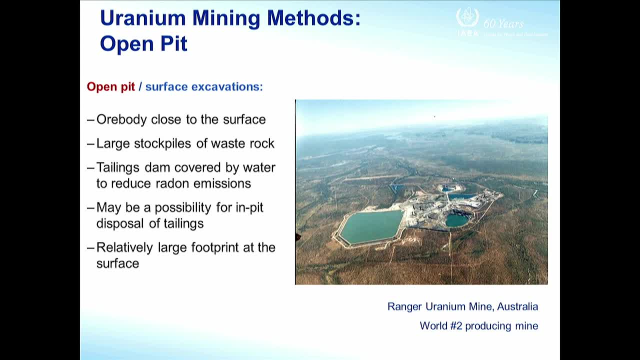 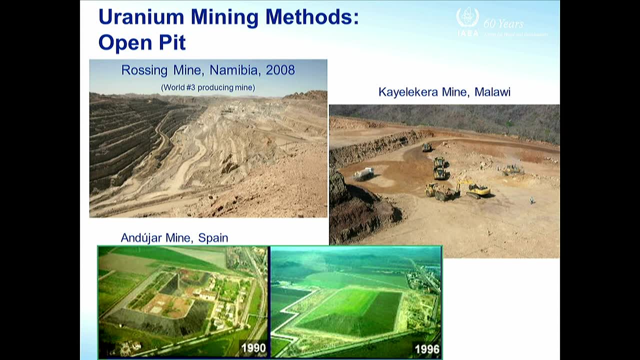 The barren rock is put under water And these tails are used after the mining lifetime And at the time of the commissioning, And this is the example of one of the Spanish mine in Andujar. So it was during the remediation and the commissioning. 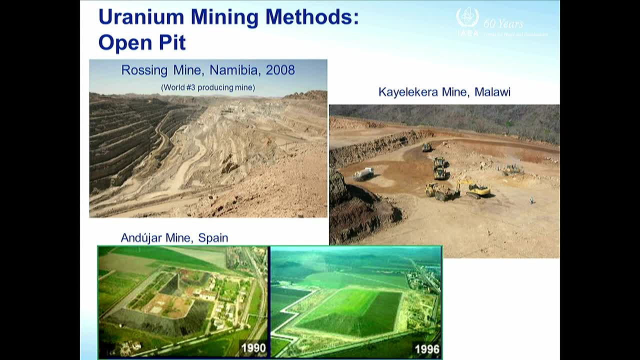 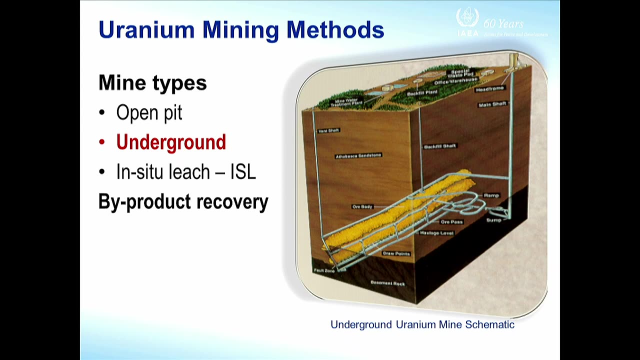 The barren rock was used to fill the pit And then this is the final situation of the mining And it was remediated. the surface. The second option is the underground And it's used when the ore body is underground And deep under the surface of the earth. 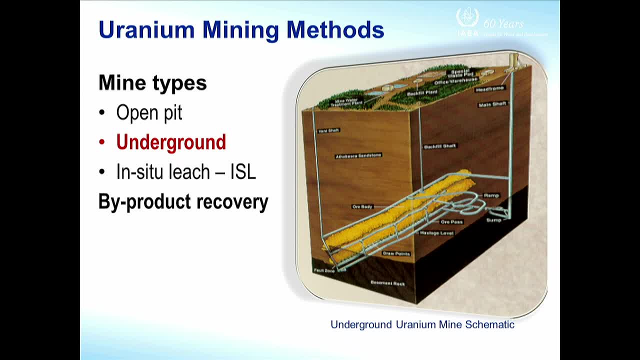 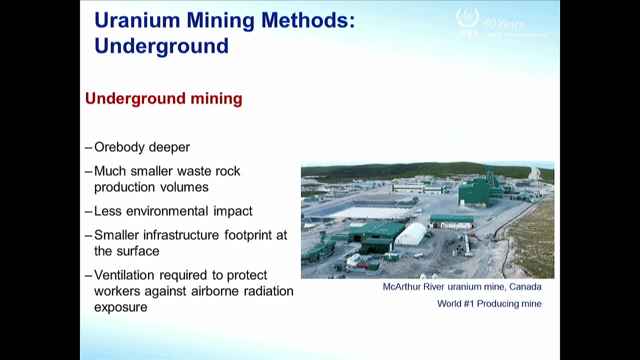 So in this case it's needed to build tunnels, And the disturbance in the surface is much less. So much smaller waste rock is produced, With a less environmental impact, And in this case ventilation is required for workers to be protected Against the airborne radiation. 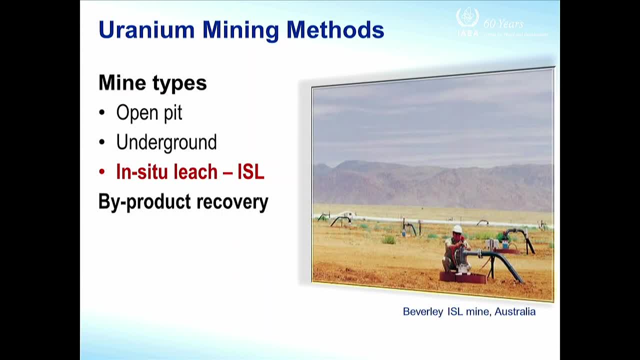 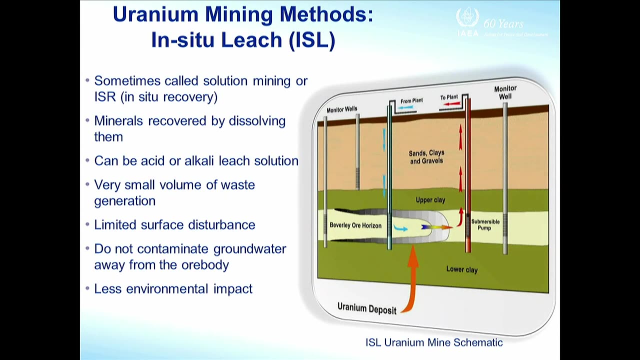 And the third option is in situ leach. So in this case the ore body remains where it is. So this is a picture of the surface, And so the ore body has to be permeable to solution, Because the uranium is dissolved using acid or alkaline solutions. 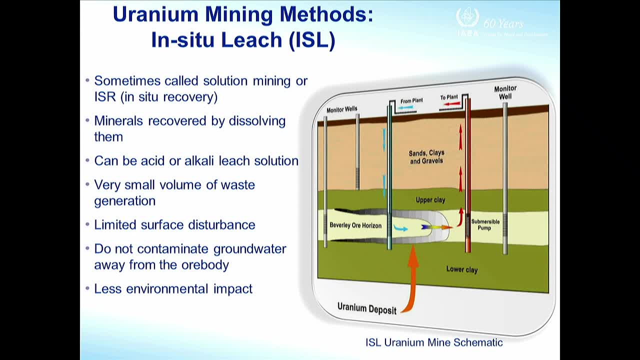 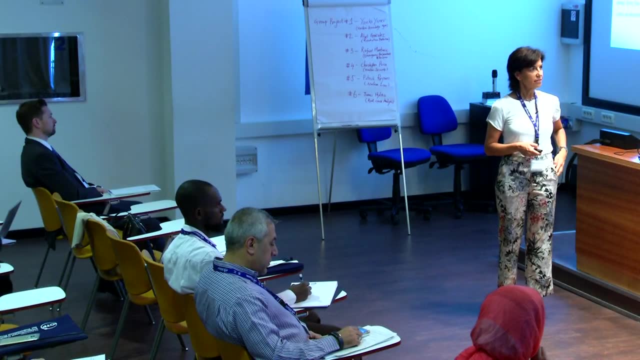 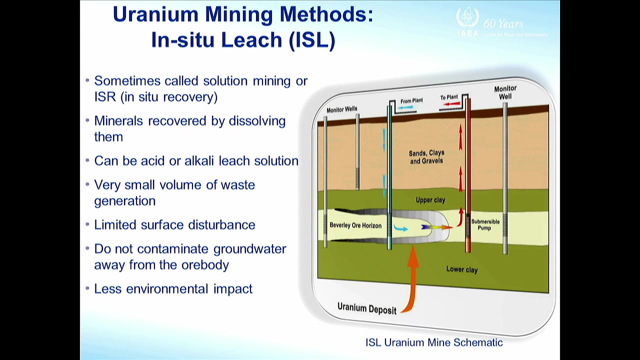 And then the liquid is pumped up to be recovered, And in this case the uranium is recovered from the leach solution By solvent-solvent extraction or ion exchange, And then it's purified and obtained the uranium oxide. So in this case, the most important thing is to prevent 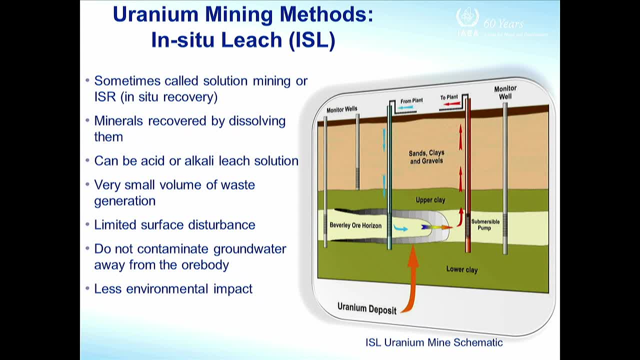 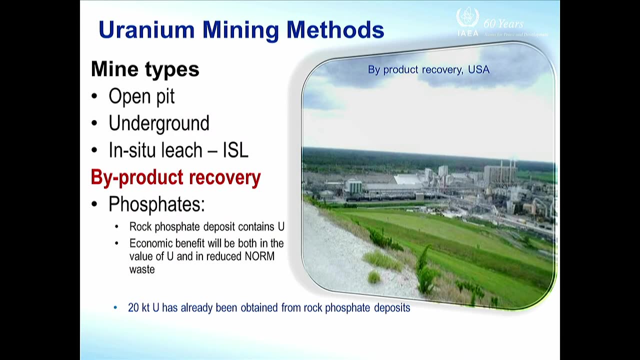 Not contaminate the groundwater away from the ore body situation And, if it's done well, has less environmental impact. Uranium also can be recovered from phosphate rocks, And so far, 20,000 tons of uranium has already been obtained from phosphate rocks. 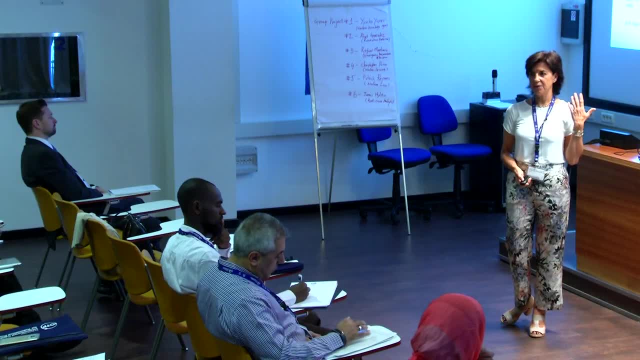 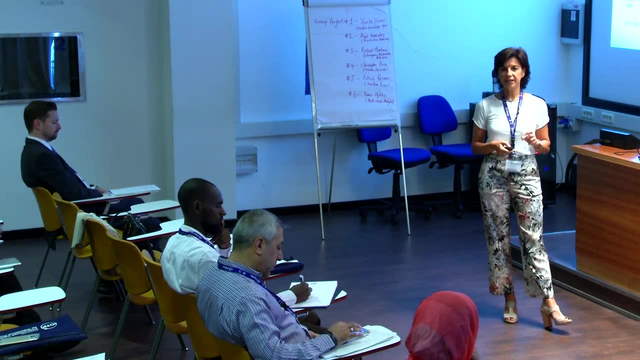 In this case, there are two benefits. In one hand, we recover uranium, But in the other hand, We reduce the amount of norm waste in the phosphate productions. I don't know if you've heard about it, But when phosphates are produced, 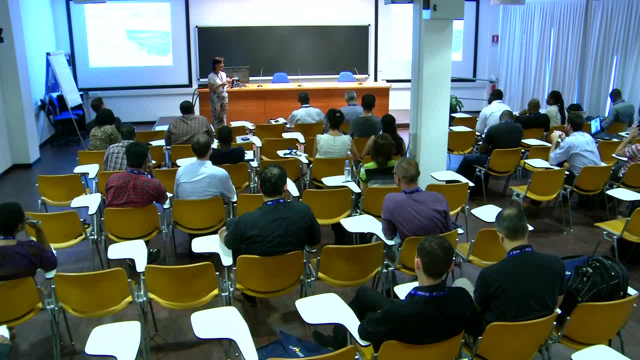 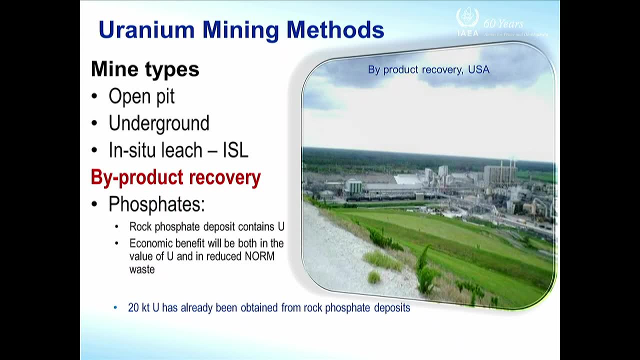 It creates a stockpile of natural. Its norm is natural occurrence radioactive material And it's a big problem because they are natural. This uranium is in the air, But it has to be controlled Under the radioactive requirements. So if we recover uranium from these deposits, 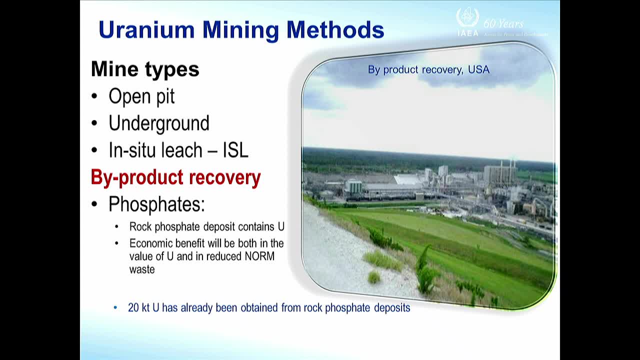 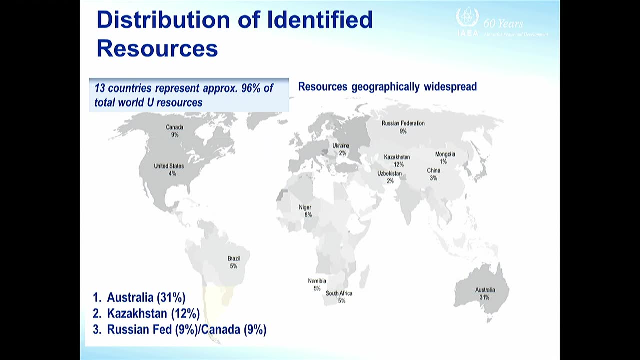 It's a benefit from these areas that produce phosphates for fertilizers. This is the map showing the distribution of resources So far of uranium. So there are 30 countries That represent approximately The 96% of the total uranium resources. 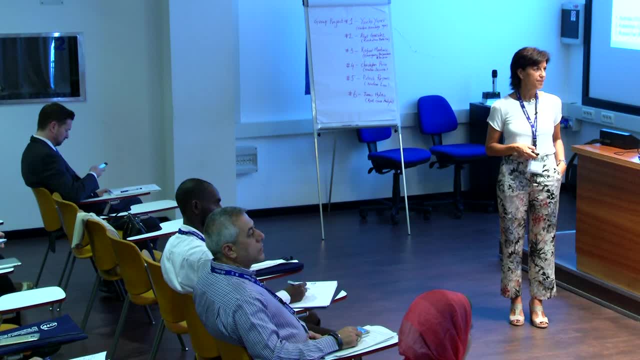 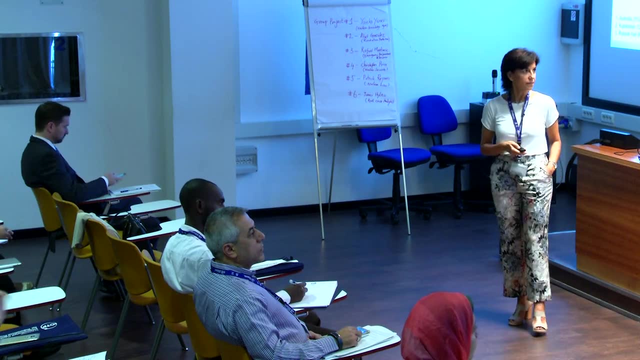 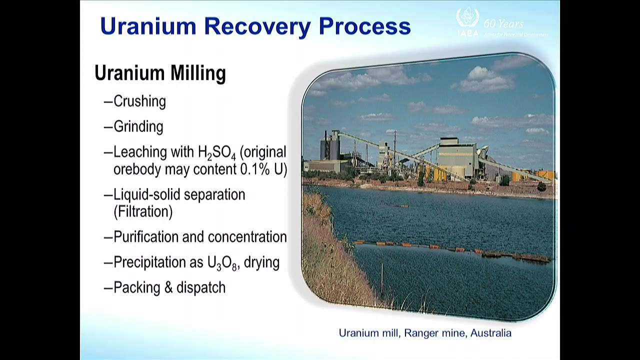 And the main sources are in Australia And second in Kazakhstan And in the Russian Federation And Canada. So once uranium is explored, The sources and also mine. Close to every mine there is a milling Where the rock obtained is scratched And ground. 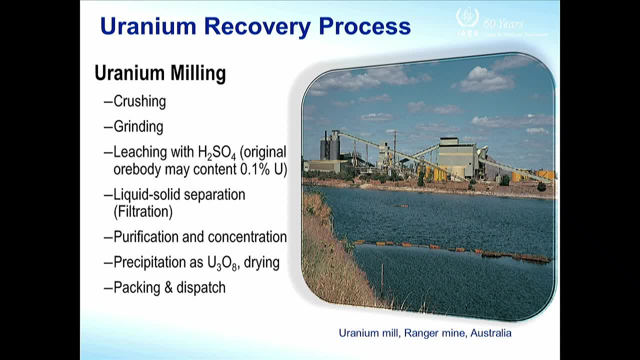 And uranium is leaching using acid solution, Because the content of uranium in the rock is very low: It's around 0.1%. So once we get the solution, Uranium is obtained. Well, first of all, we have to separate the barren rock from the liquid. 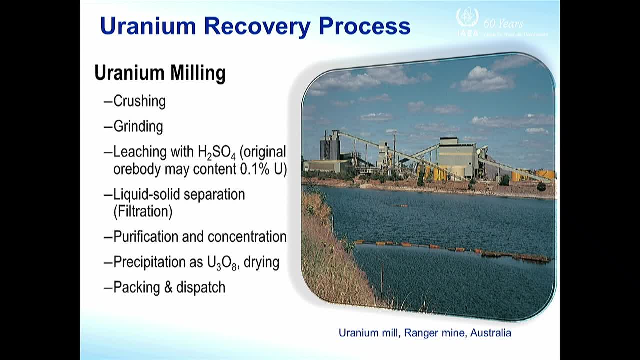 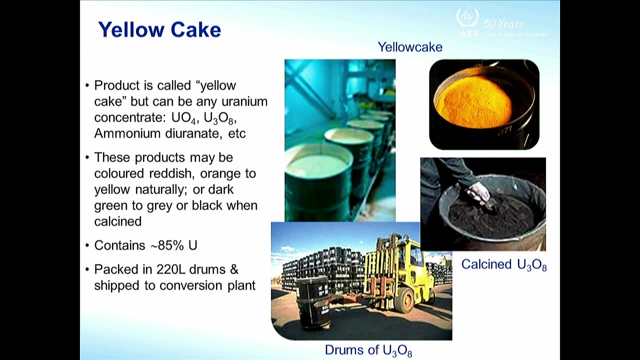 By filtration And, after the solution is purified And concentrate, Getting U308.. That is the way that uranium is packed and dispatched And this is the so called yellow cake. So the yellow cake Can be yellow, It's yellow, But when it's calcined, 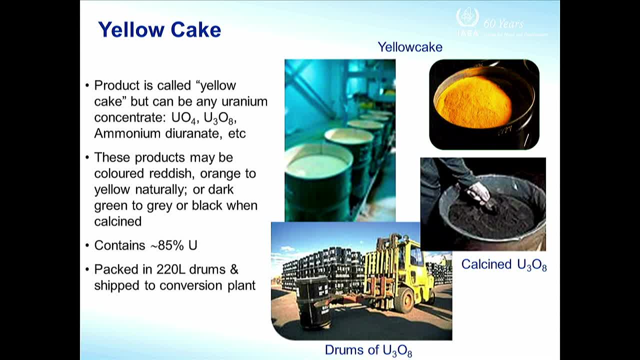 It's grayish, Dark, Very dark. So this is the way that uranium is dispatched And contains the Contains- around 85% of uranium- And is packed in 220 liters drums And it ships to the conversion plant. Why? 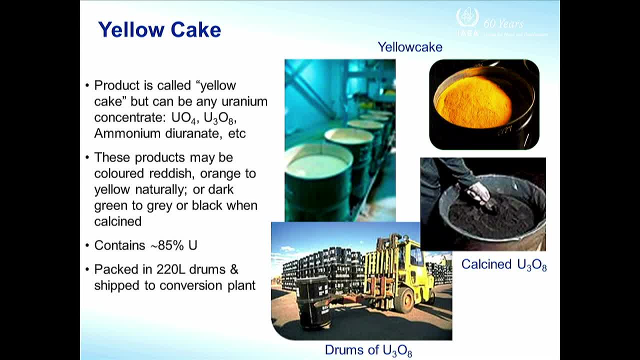 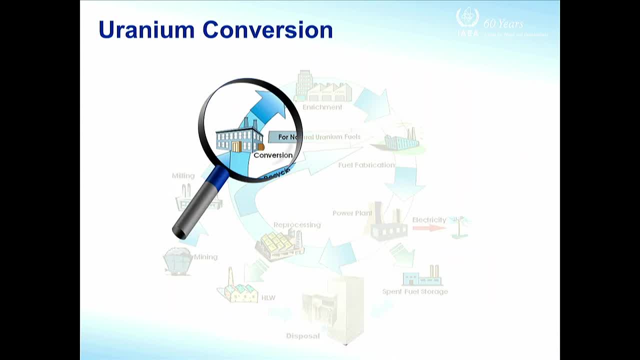 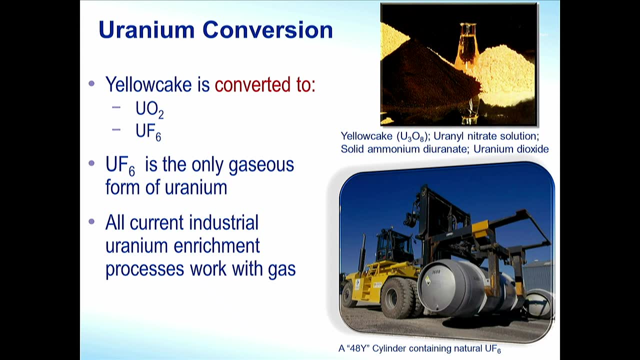 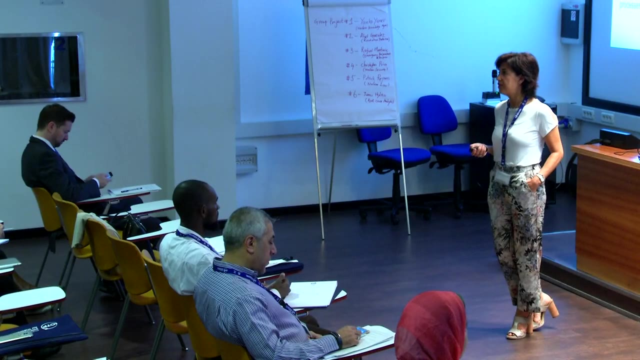 Because in this form Uranium is not suitable to be used in the reactors. So in the conversion plant The U308 is converted to uranium dioxide And in this case Can be used by the reactors that use natural uranium, That's the can do reactors of the heavy water pressurized reactors. 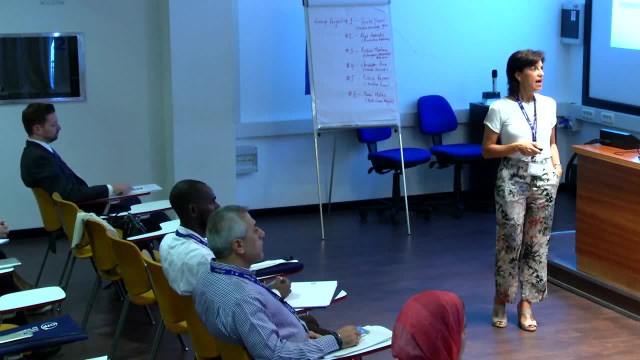 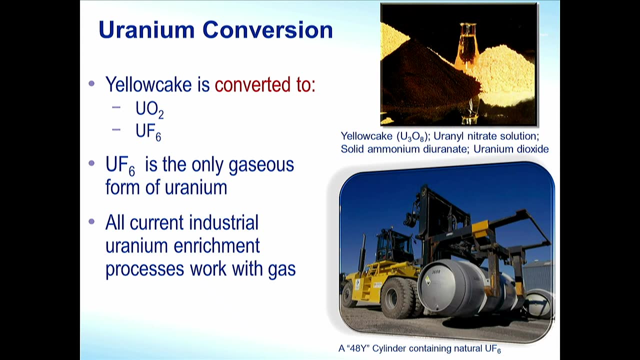 And in the case of those reactors- Light water reactors- We need to use uranium- enriched Uranium- The yellow cake- is transformed in hexafluoride uranium, Which is the only gaseous That can be used. This is the only gaseous compound of uranium. 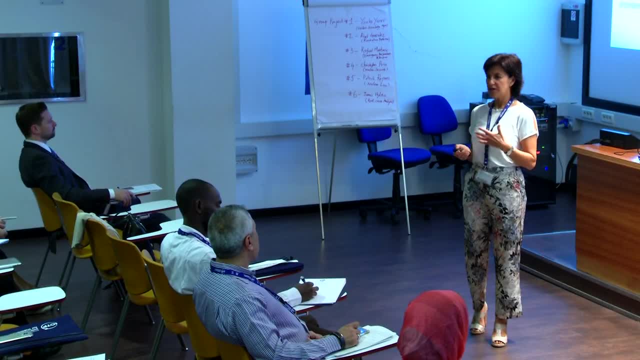 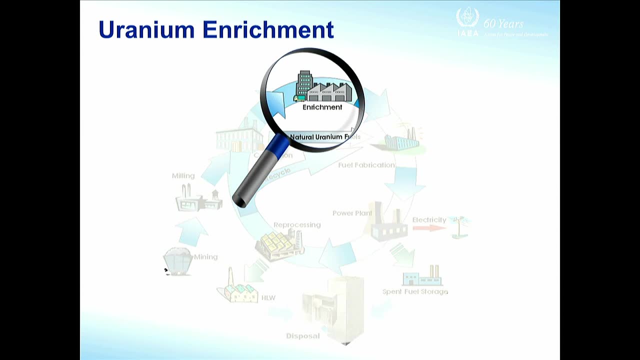 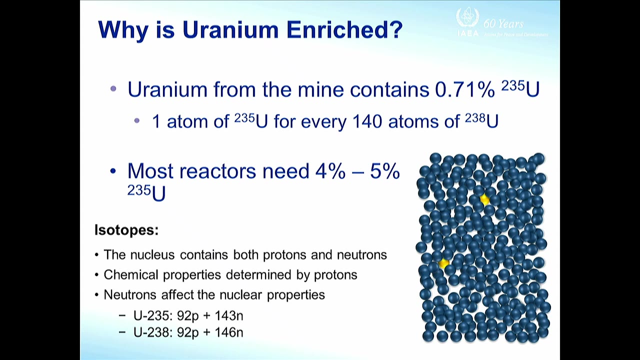 Because so far All enrichment process work in gaseous phase, So let's go to the enrichment step. So why we have to enrich? Because the natural uranium 5 concentration in uranium, The isotope composition, is 0.71% of uranium 5.. 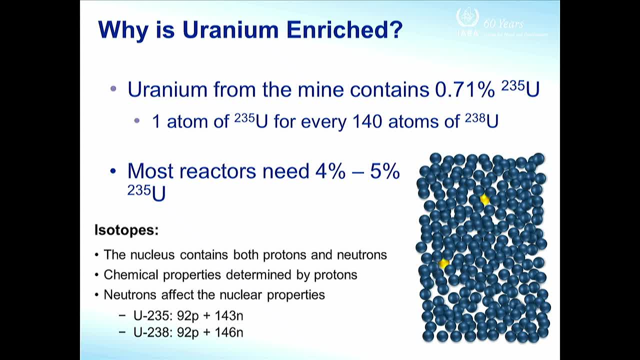 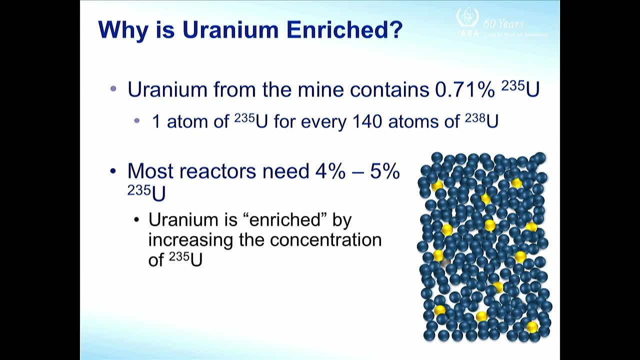 And most of the reactors- Light water reactors- work with 4%- 5% of uranium 5.. So the concentration of uranium 5 in the uranium Has to be increased. And how we can do that? Because it's very difficult to work with isotopes. 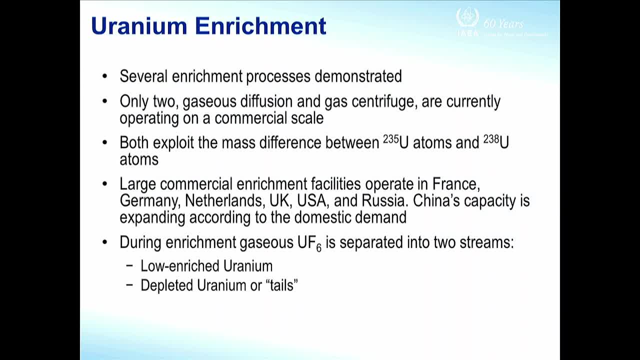 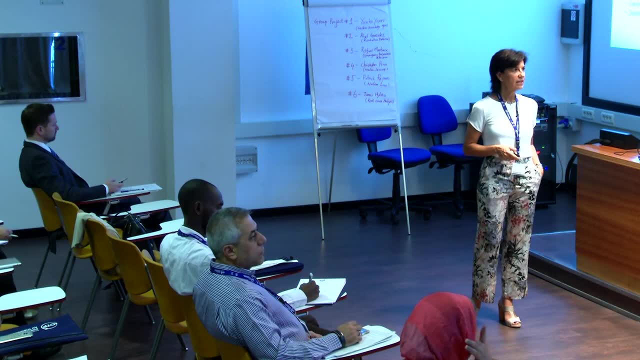 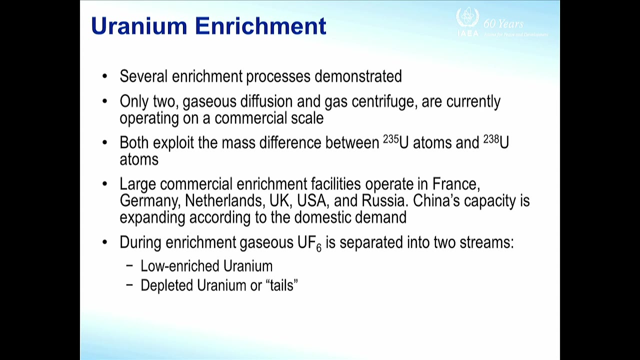 Of the same element. They have the same chemical properties. So there are so far some Several enrichment processes demonstrated, But only two are commercially available. Both expose the difference of mass Between the isotope 5 and 8. And there are large commercial enrichment plants. 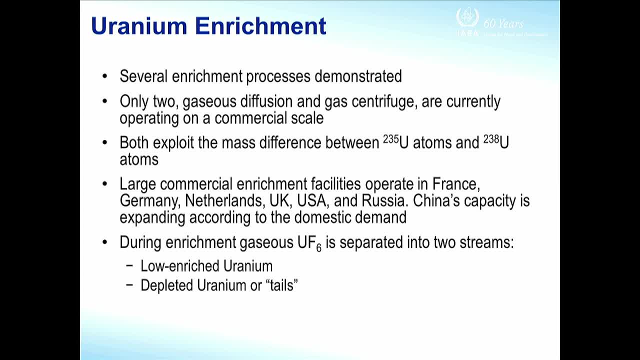 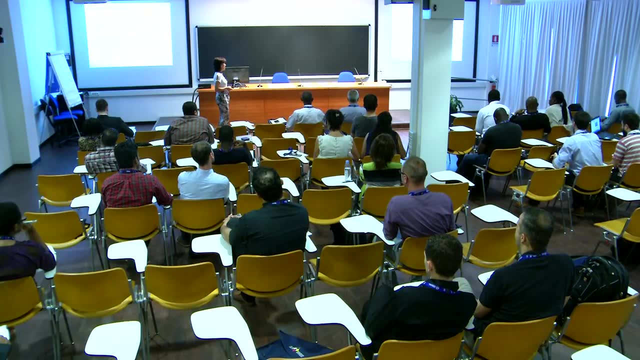 In countries such as France, Germany, Netherlands, UK, United States And Russian Federation And China is So it's now. It's currently increasing Their capacity, Their on demand is increasing. So during the enrichment We will see that we will get two streams. 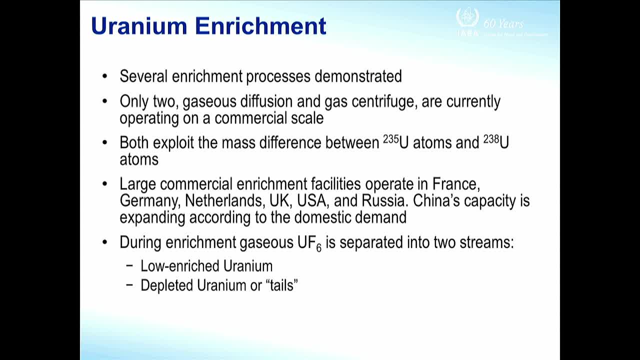 One stream is the so called low enriched uranium, Which will be 4, 5% enriched, And the other streams is called depleted uranium Or tails, So it's the uranium stream Containing less than 0.7% of uranium 5.. 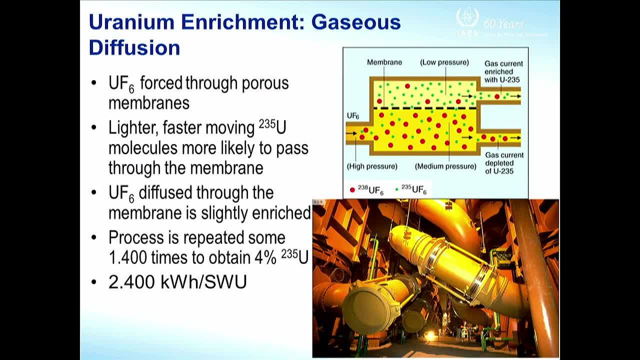 So the two options Is the gaseous diffusion- It was the first method used- And in this case The hexafluoride of uranium is forced To go through a membrane To a high pressure And then physically The lighter atoms. 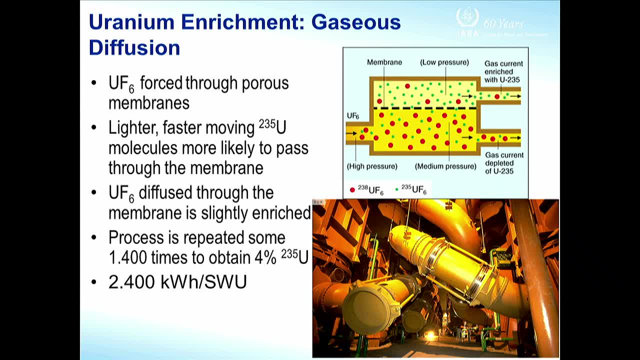 Pass through the pores of the membrane. Meanwhile the heavy, The heaviest One remain in the lower part. So this process is repeated, Repeated, many, many times, So to get around 4% of uranium 5.. It has to be repeated. 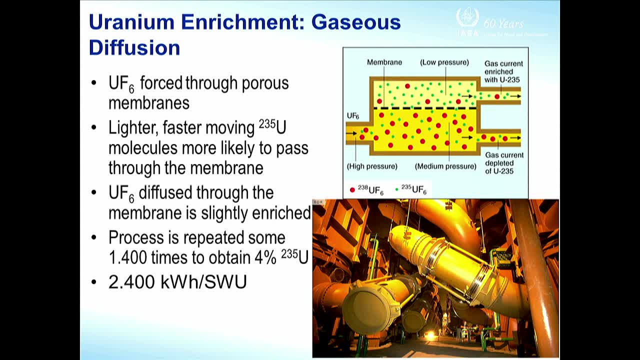 Around 1400 times. So this process is very, very energetic, Consumes a lot of energy, And the energy that it's consumed During the process Is measured In this separative working Units. We will see What does it mean. 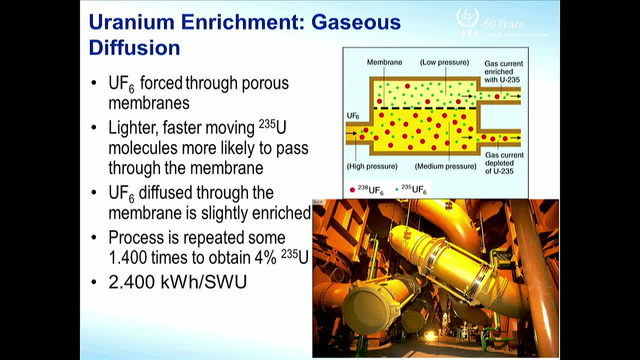 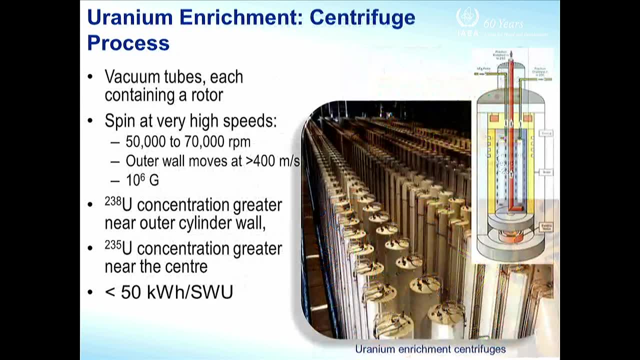 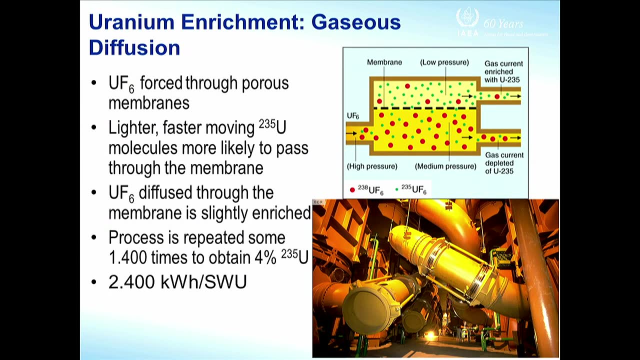 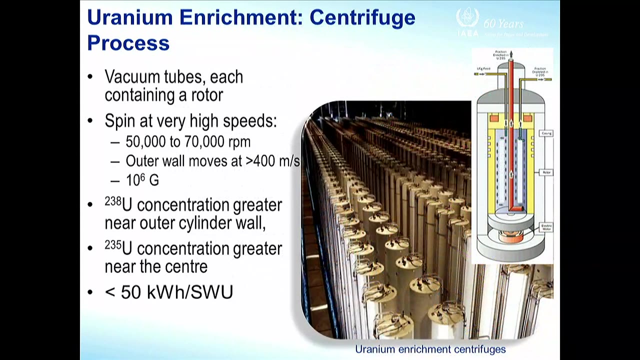 And it consumes around 2400 kilowatts per hour Per zoom. So the All facilities Dedicated to gaseous diffusion Are going to be dismantling And stop when they reach Their lifetime. Their lifetime And now. 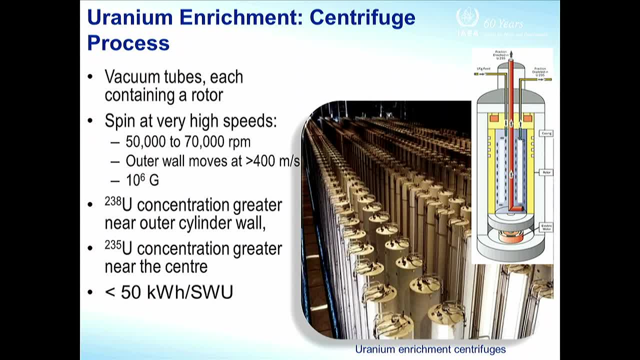 The more used. The more used Method Is the centrifuge Process That consists In Tubes, Vacuum tubes, With a rotor That speeds A very high Speeds, Around 50,000 to 70,000.. 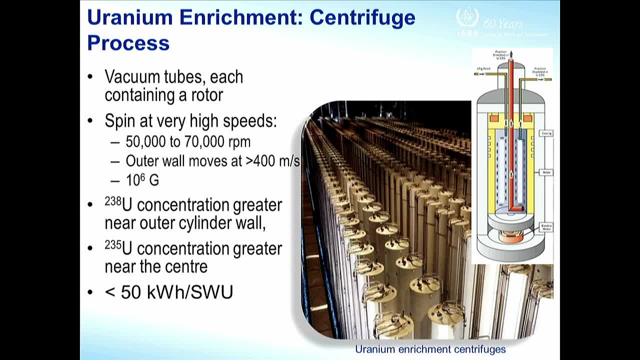 RPM, And in this case The heaviest Atoms are moved To the surface, To the walls Of the cylinder, And the Lighter remains In the middle. So, Repeating The process Several times, We get. 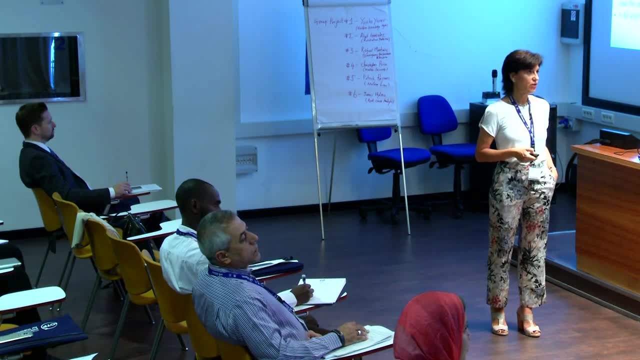 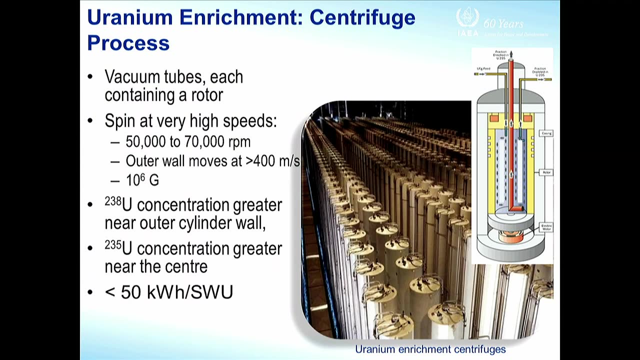 The separation And the Of the To increase The concentration Of uranium-5. In the final product, And in this case You can see, This process Consumes Much less Energy, So 50. Kilowatts per hour. 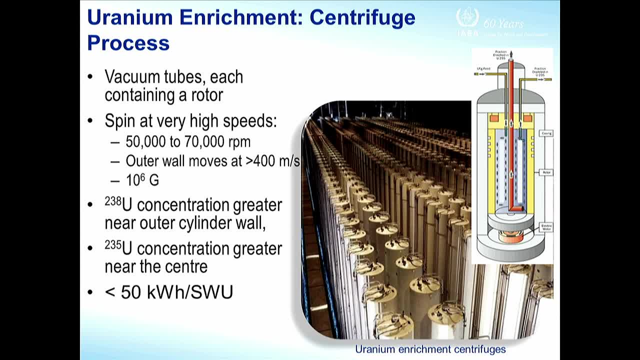 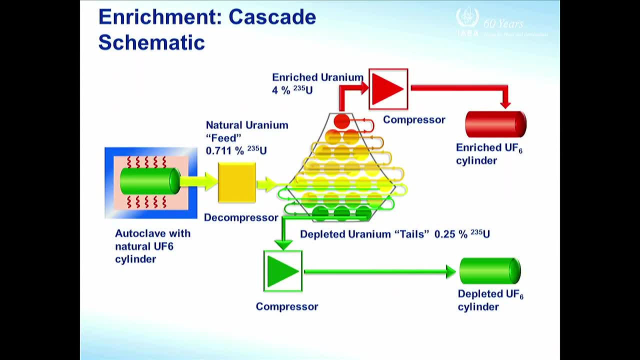 Per Zoom. So now Is the The most Used Process And Has to be done In cascade. That means That there are Many, many Tubes In series, And then, If we repeat The process, 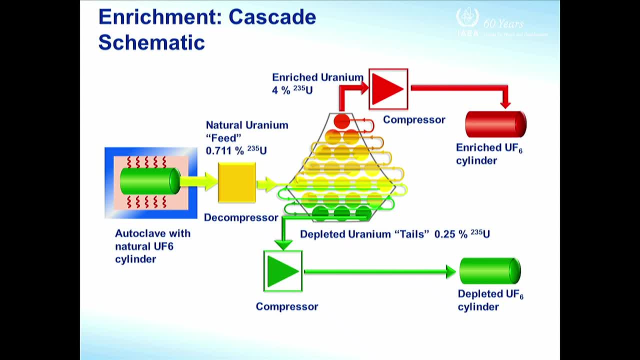 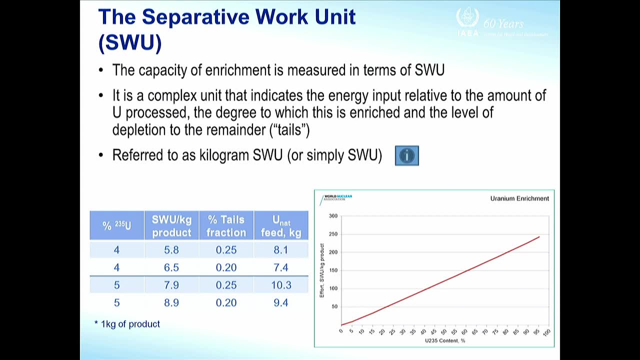 Several times We get At the end The rich Uranium And The depleted Stream. So What means Zoom? The Separative Work Unit Is a very complex Unit That Indicates The energy. 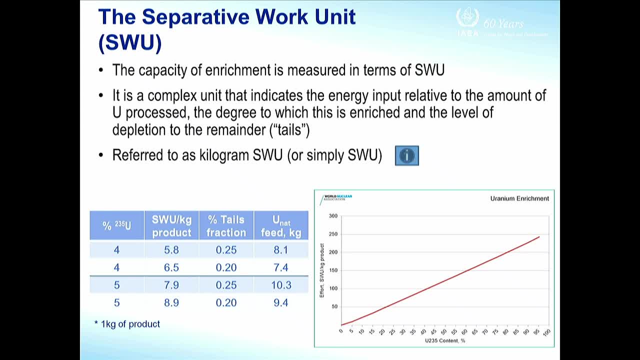 Input That Process, The degree Of Enrichment And the degree Of Depletion In the Tales, And Can Be Referred To A Kilogram Zoo Or Simply. 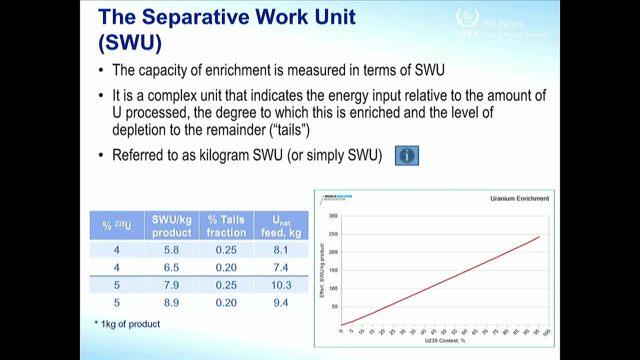 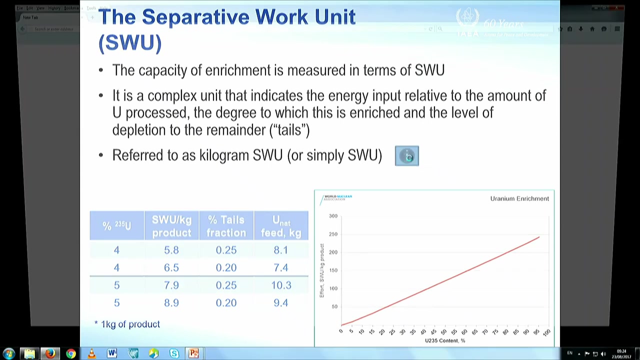 Zoom And, For Example, This Is The Evolution Of Zoo Depending On The Enrichment, So We Can Play If It Works. See, For Example, If 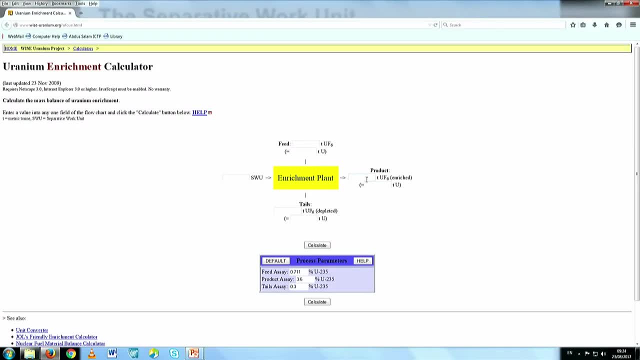 We Refer. Okay, So We Can Refer To One Ton Of Product And We Can See If We Like To Get Four Percent For Example Of 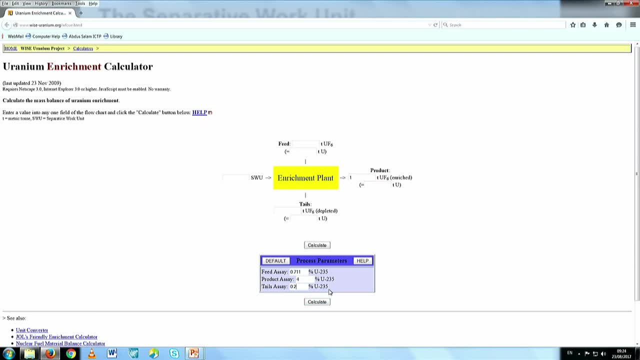 Enrichment, And We Like To Have A Tale Of 0.3.. Or Let's See 0.2. Of The Plate Of, Let's See He. 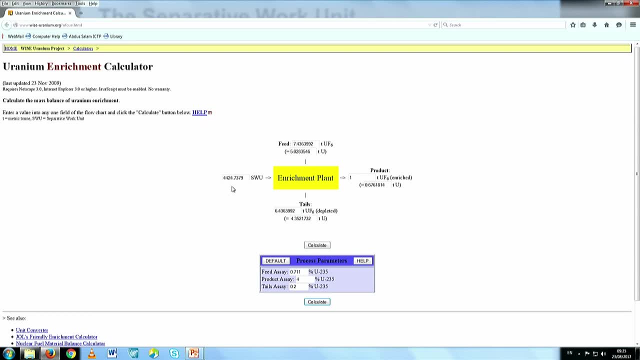 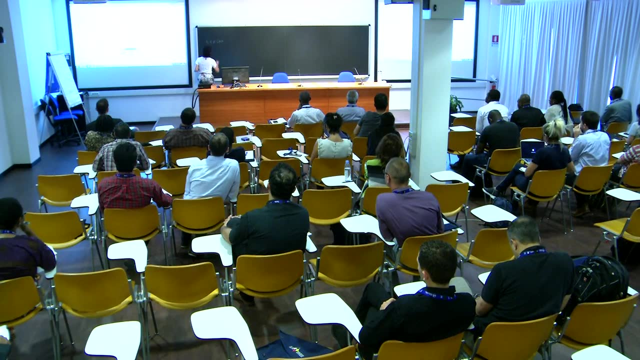 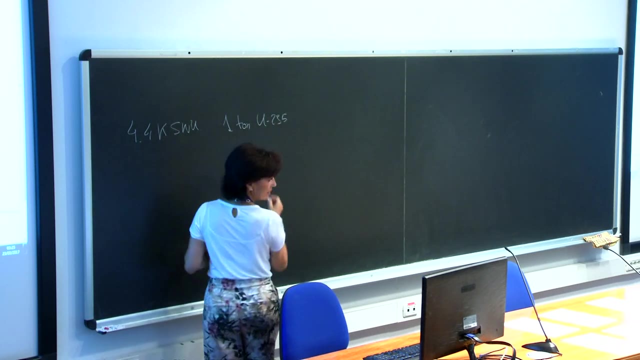 Knows You, But Per Kilograms Of, Per Ton Of Uranium Enriched. So We Have A Ton Of Uranium At. We Said At 4%. 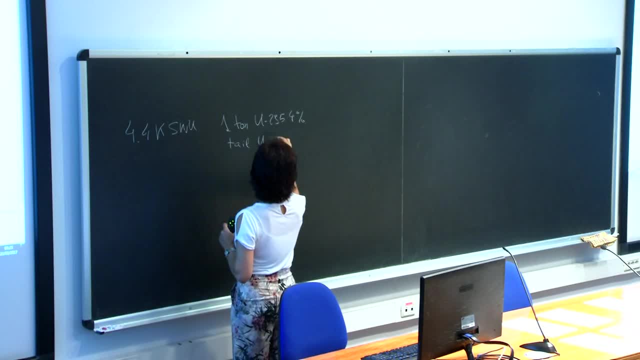 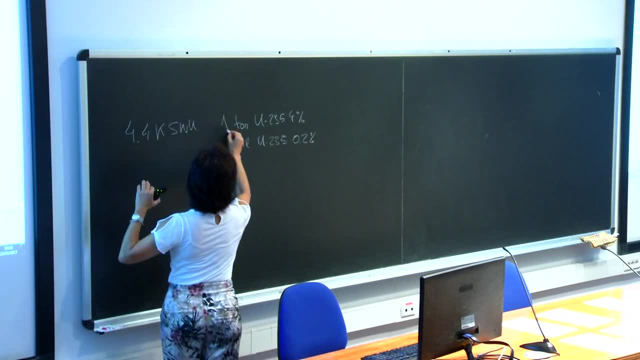 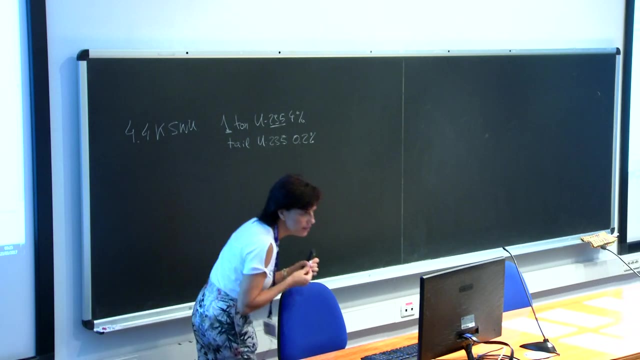 With A Tale Of Uranium, We Said 0.4.. But For The Same Tone Of Uranium To 35.. 4%. And We We Need. 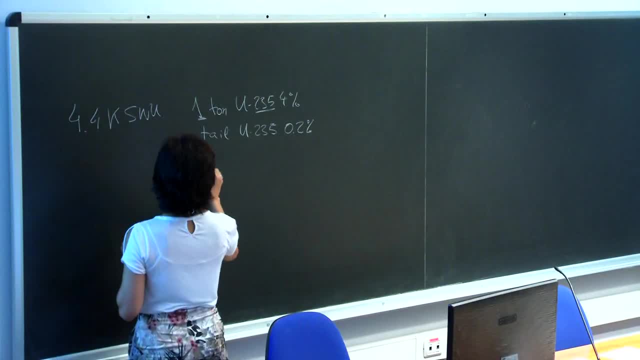 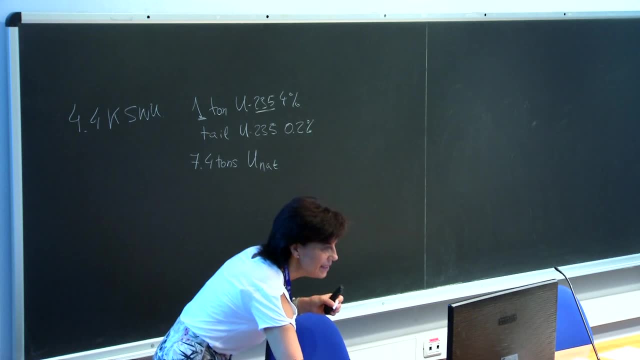 To Feed The System With Seven Tones Of Natural Uranium 7.5.. But We Have A Multiplated Tale And If We Keep The 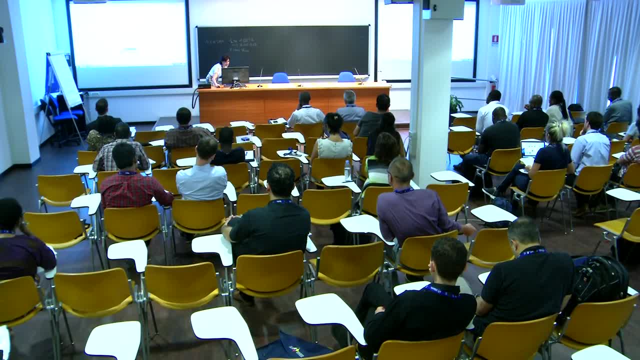 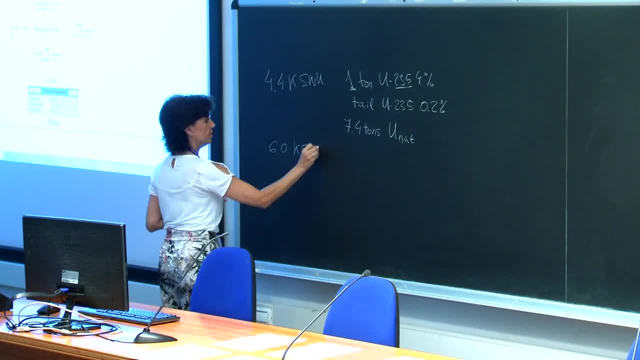 4%, We Keep Everything And Then We Will Consume More Energy. So 6. Kilo Su For The Same Uranium, We Will Consume 6.. 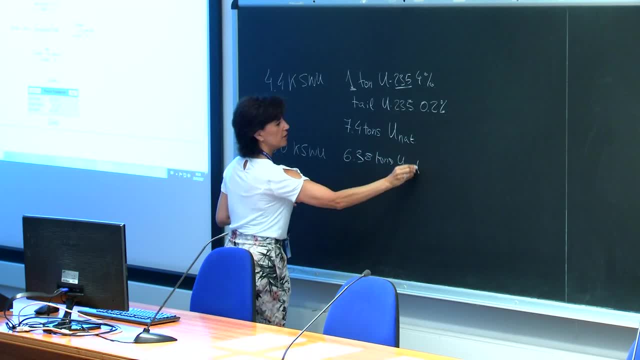 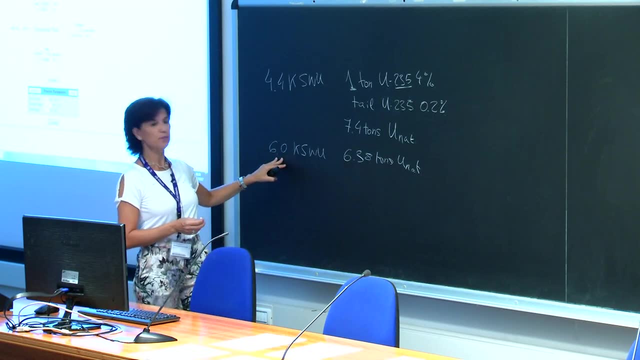 Point 38. Tons Of Uranium. So We Will Need Less Feed, Less Amount Of Uranium- Not Natural Uranium- But We Consume More Energy. 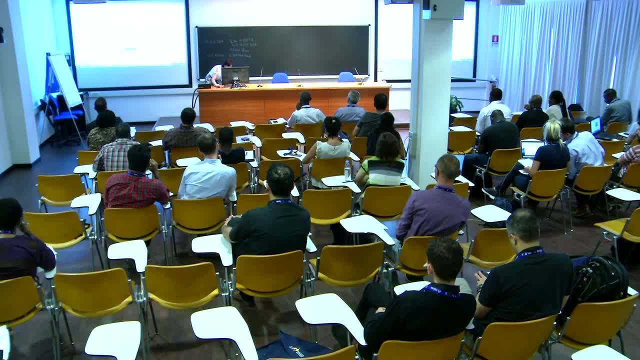 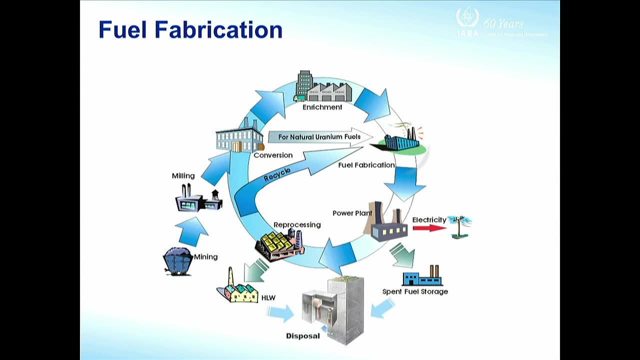 So We Will Keep Everything, Everything, We Will Consume Everything, We Will Consume Everything, We Will Consume Everything. So, Once We Have The Uranium, 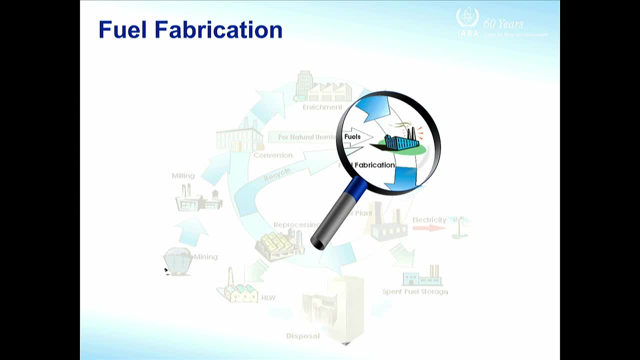 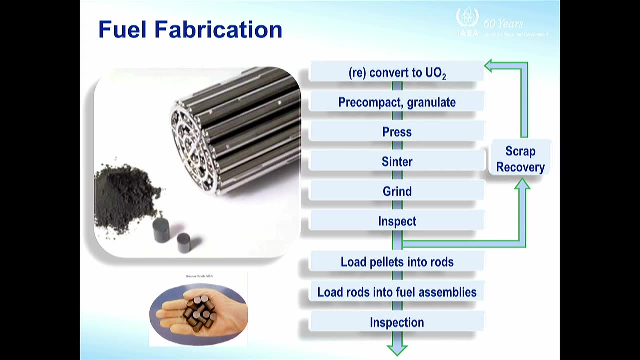 In Reach At The Amount Necessary To Enrich Uranium. We Have To Make The Pellets By A Process Called Sintering At High Temperature. 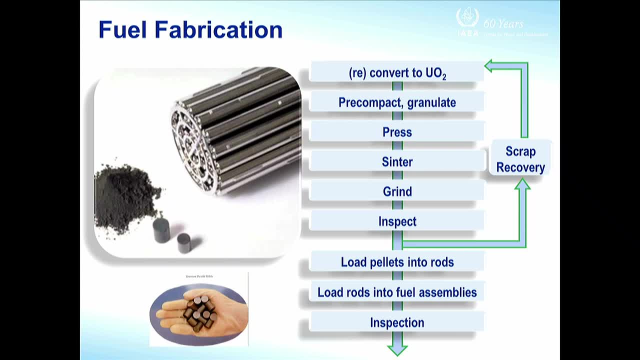 Around Nine Hundred Degrees And This Process Is To Make The Pellets By Uranium And This Process Has To Meet A Very Tight Quality As 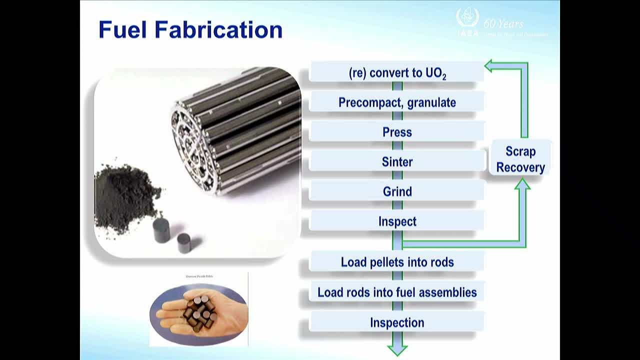 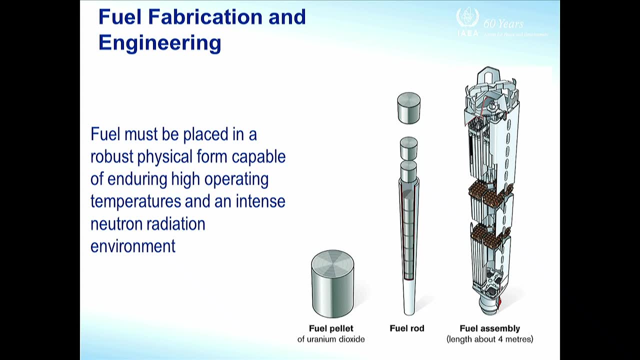 Specific, Specific. So The Size Of Pellets Is One Centimeter Per More Less One Centimeter, And These Pellets And The Roads With Containing 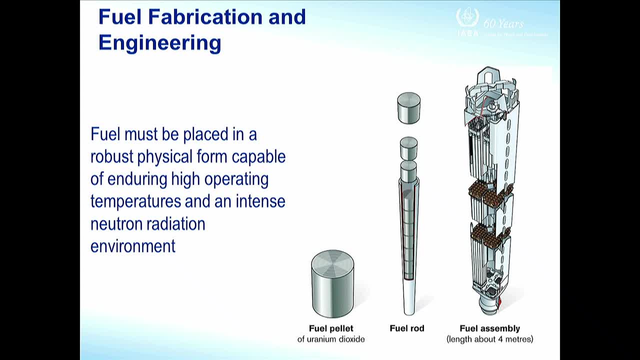 The Pellets Has To Be Placed In A Very Robust Structures That Are Called Bundles Or Fuel Assemblies, And These Structures Has To 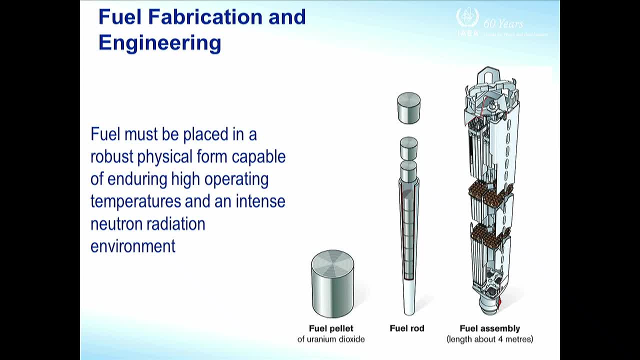 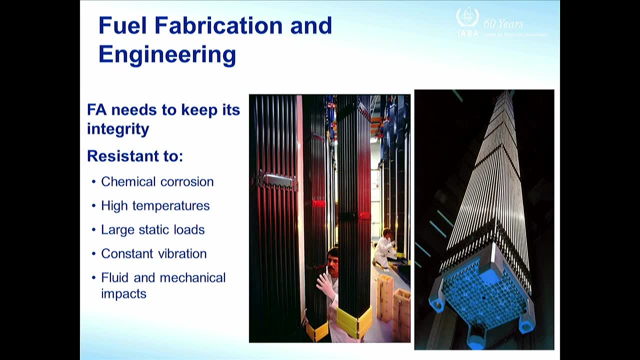 Be Resistant Against The Chemical Corrosion Because The Water Is In The Core Of The Reactor, The High Temperatures And Also The Static 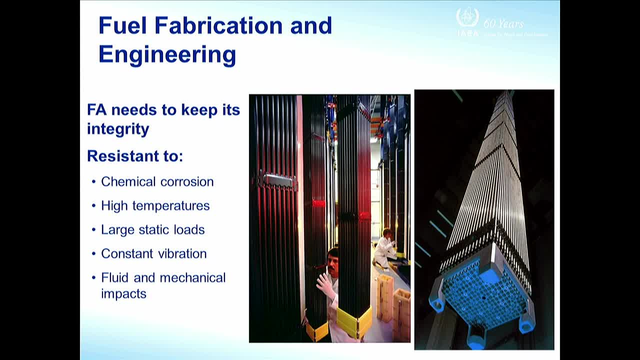 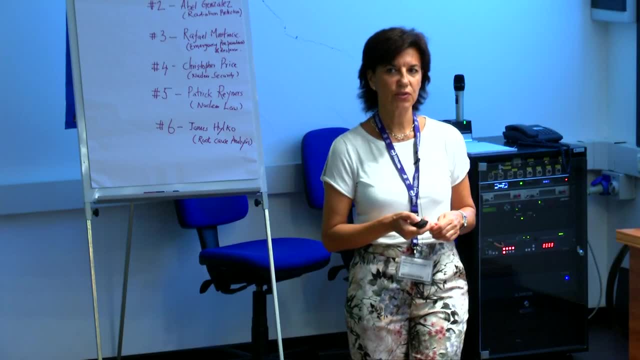 Loads And The Vibrations And The Fluid Impacts Not Only In The Core Of The Reactor But Also During The Storage And All The 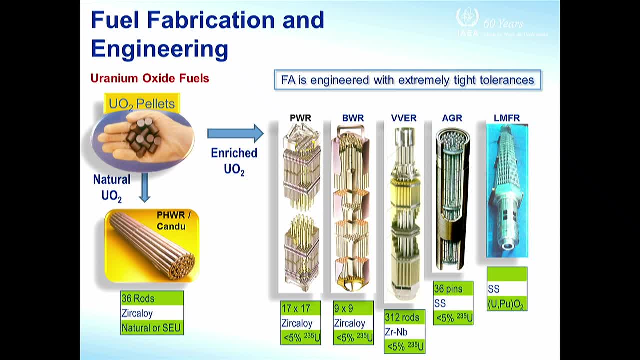 Handling Steps That The Fuel Assemblies Has To To Undergo. There Are Different Roads, Assemblies In Circular And The P W R Is The 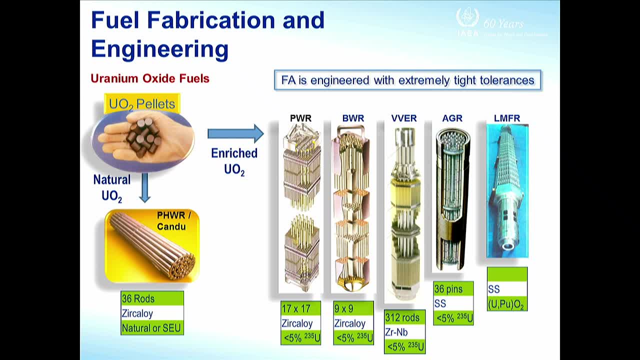 Biggest Fuel Assemblies With 17.. But 17. Versus 17. Pins In Circular The B W R 9. Is Use 30. 300. 12.. 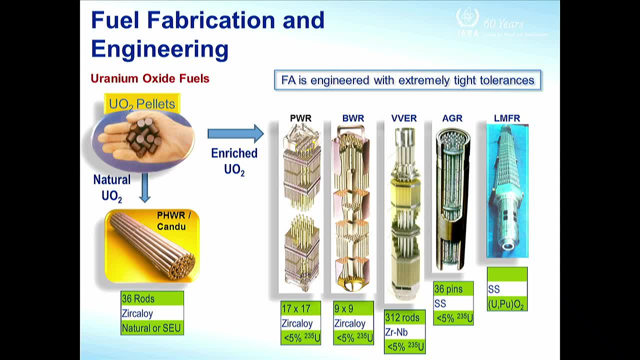 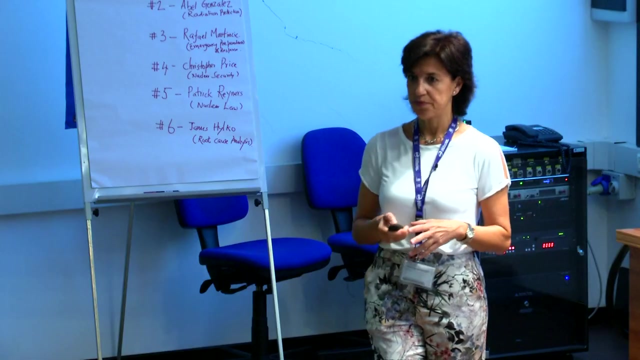 Roads In Circular And The Advanced Gas Reactors Use The Pins, And The Pins Are Covered By Graphite And We Will See When We Will. 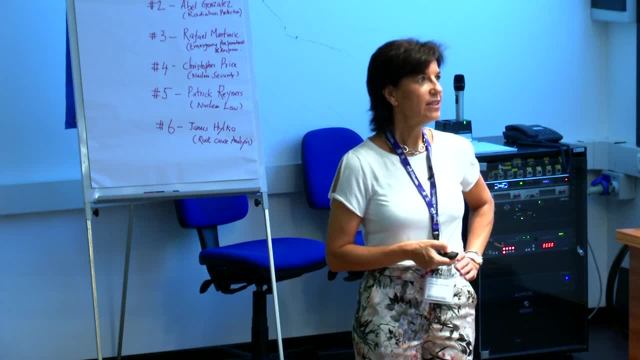 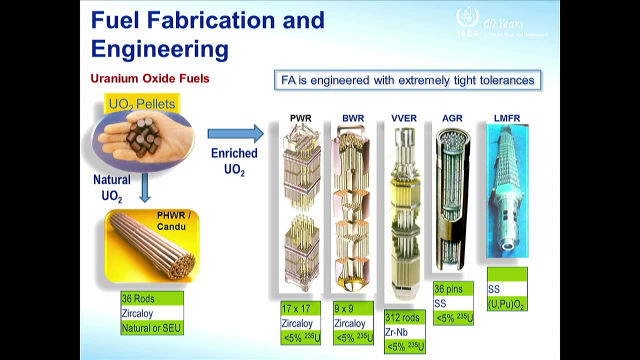 See What's Happening During The Commissioning. And Also, This Is The Assembly, The Fuel Assembly For The Fast Reactor, The Sodium Fast Reactors. 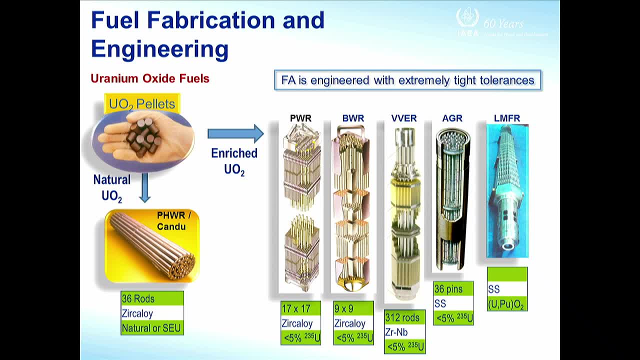 Sorry, The Roads. Yes, The Number Is Four Meters Tall And It's- I Don't Know What Is The Size. That's The Seventeen, Seventeen. 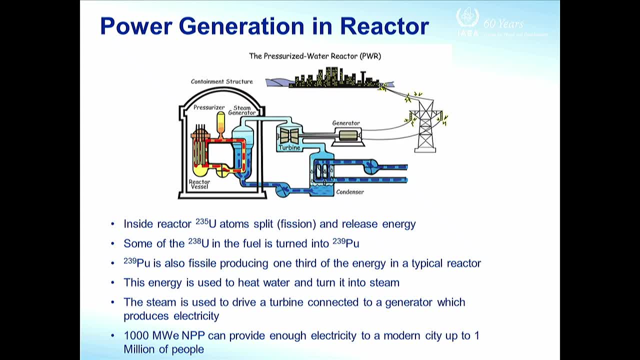 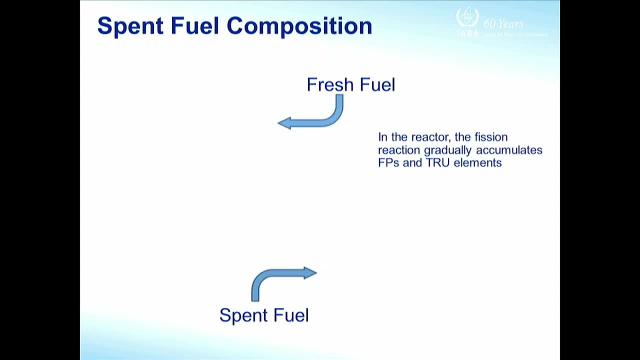 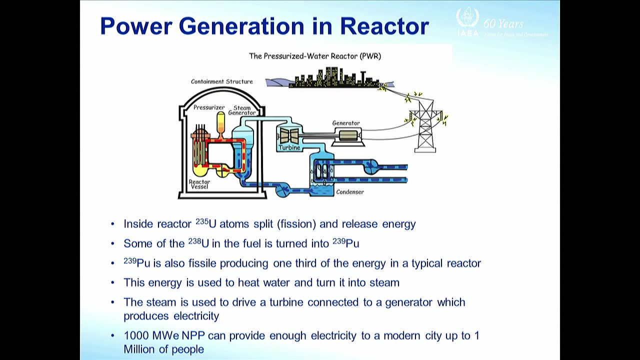 Roads, And Seven, Seventeen. So Once There We Have The Fuel Assemblies Placed In A Placement. So The Last Is The Energy Of The 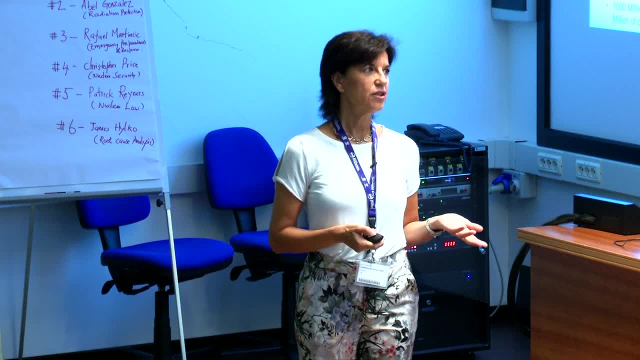 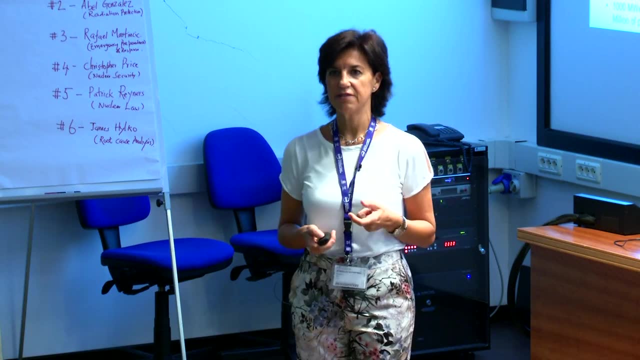 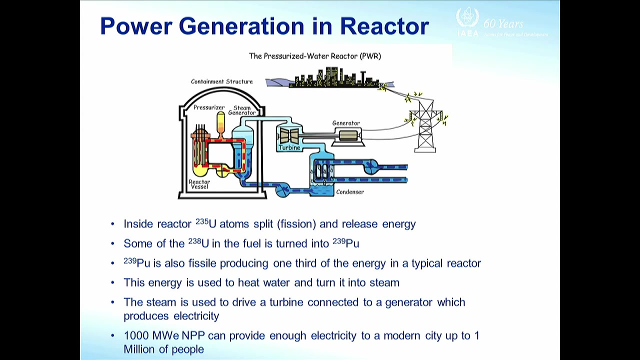 Water, So The, The Energy Is Sustained, So The Energy Is The Front Of The Energy, Of The. So, once the fuel stays in the core, for around three years more or less, 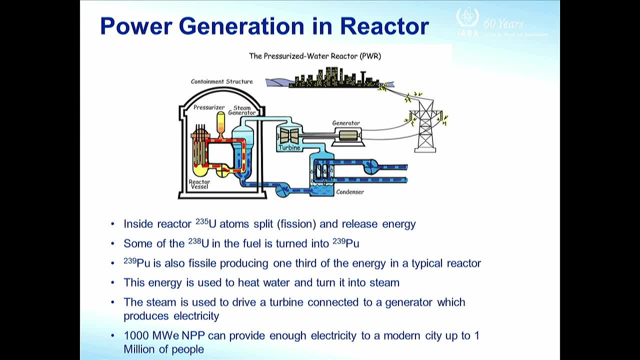 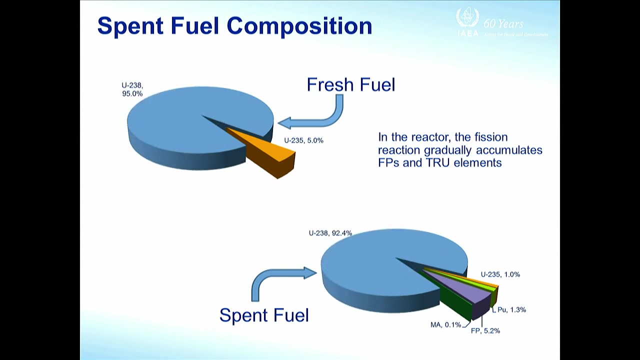 it doesn't meet the safety requirements so far because it became to be more absorbed. neutrons And also the metallic parts can be embrittled. So it's decided to consider the fuel spent. after three years in the core And the composition of the fuel has changed from 95% of uranium-8 to around 92%. 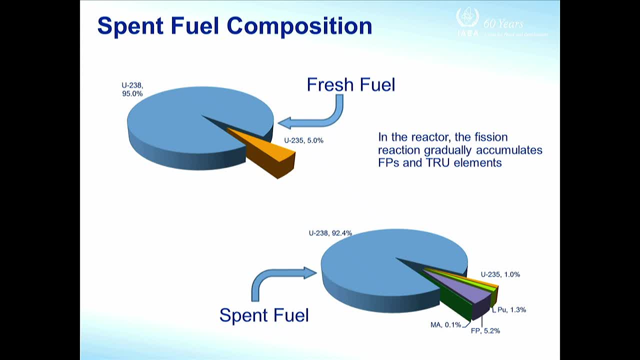 and from 5% of uranium-5 to 1% of uranium-5 remaining, And also we have now a new element that is plutonium in a concentration about. we have fission products and around a composition of 5% and also the so-called minor actinides. that are the actinides. 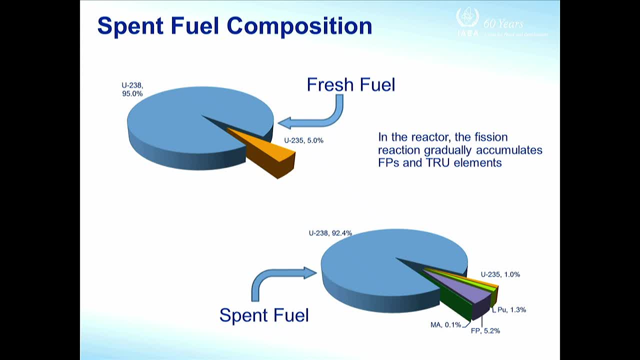 that are not uranium and plutonium. so neptunium, americium, curium, californium, becquerelium, and they are called minor actinides because they are in a very lower concentration compared to uranium and plutonium. 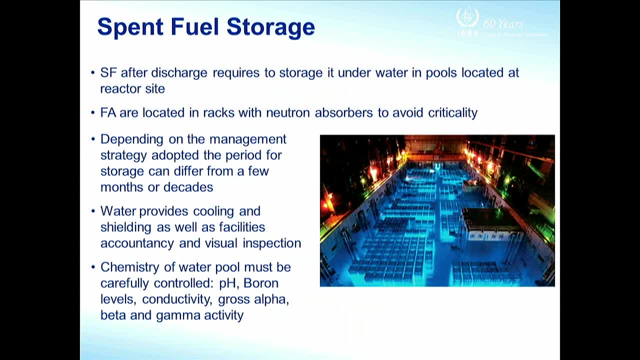 So once the spent fuel is considered- the fuel is considered spent, It should be- it has to be stored underwater due to its characteristics, because it's very the heat production, the decay heat, and because the water serves as biological shielding. 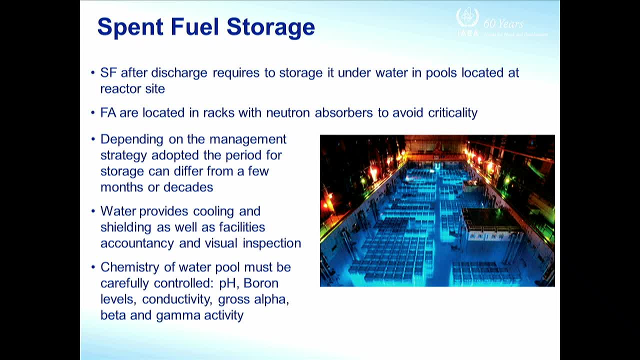 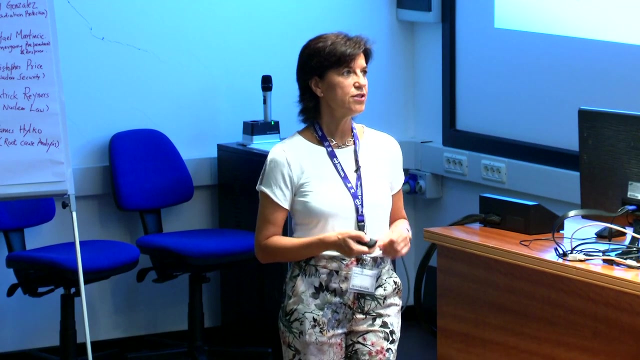 So the pools are located in the reactor building and the fuel assemblies are placed in racks. That has materials that absorb neutron to avoid criticality. So, depending on the strategy to manage spent fuel, the spent fuel can be stored in the pools for from decades or months. 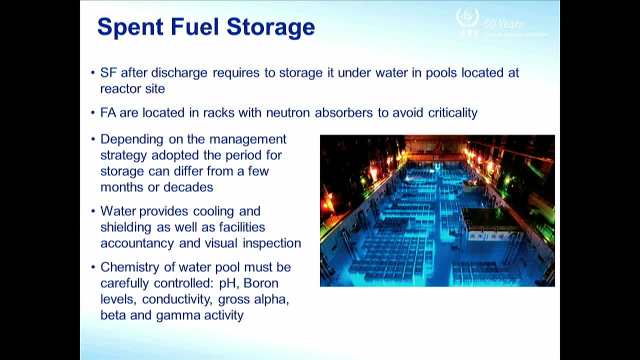 And the water not only provides shielding but also allows visual inspection of the fuel assemblies. And the chemistry of the water has to be strictly controlled. So, for example, the routine controls are to the measure of the pH, the boron levels, because the boron is used by 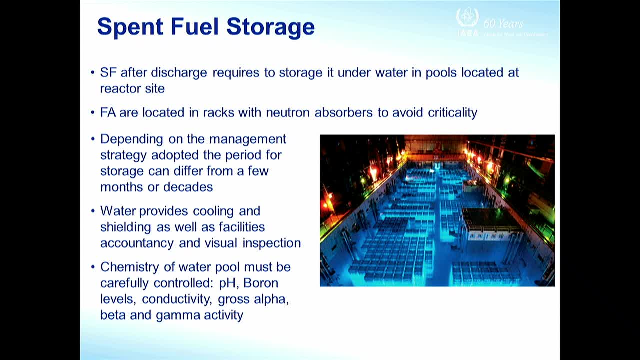 as a neutron absorber. the conductivity, because the conductivity gives us the idea of ions present in the water, and also the gross alpha, beta and gamma activity, because it indicates if there is release of radioactivity from the fuel assembly. that means that there are pinholes in the rods. 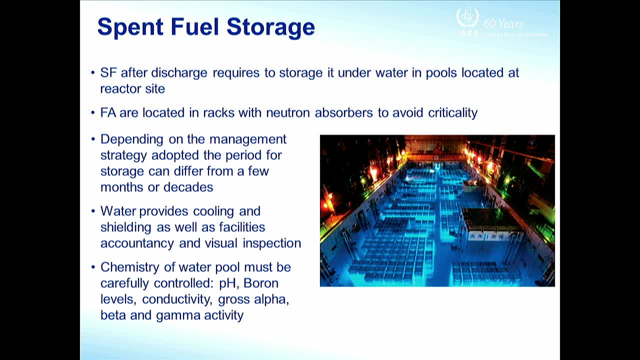 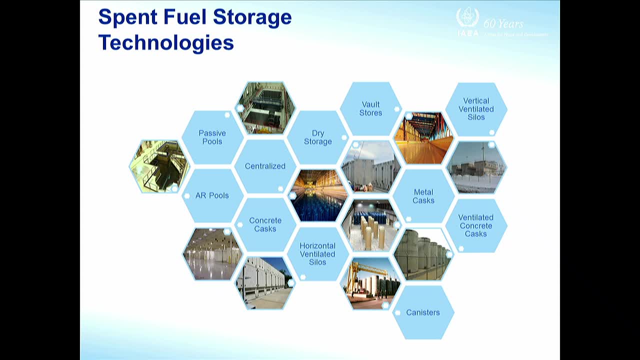 and give an idea. so a leakage of radioactivity. So there are different options and techniques to store the spent fuel and goes from wet at reactor or away from reactor, and also dry options. Once the spent fuel spends time in water, we can. 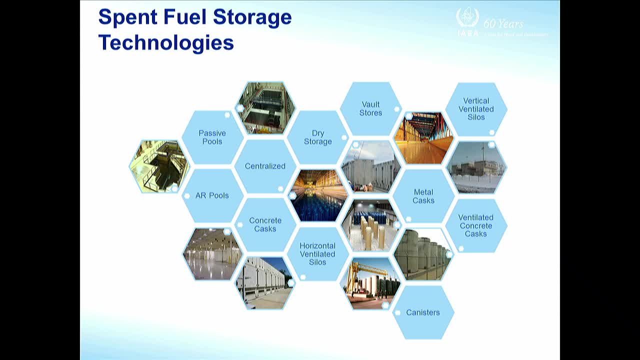 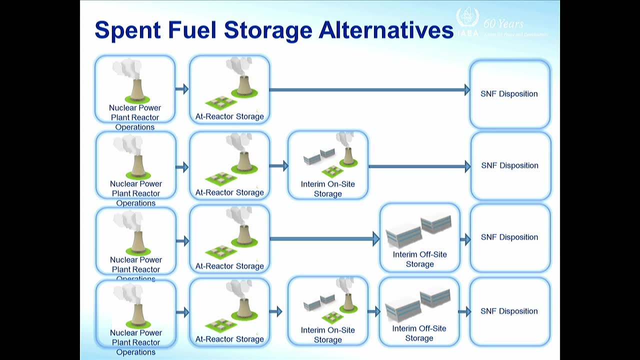 there are options to move the spent fuel to dry storage. So let's see, These are the options to store spent fuel, So it could be at reactor storage for a long period of time and then go to the final disposition, Or 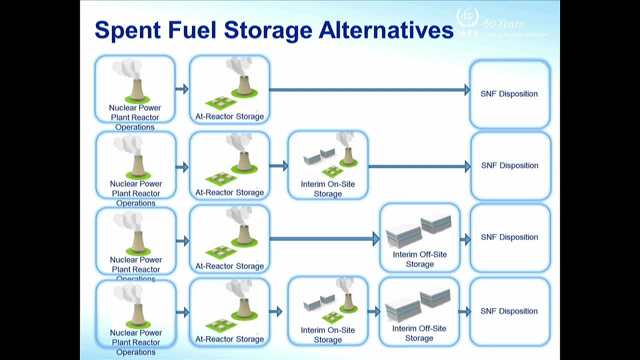 it could be in the at reactor storage facility in pool, and then the interim storage, usually in dry, could be on site and then to go to the final disposition. There are other options that after a period at reactor, if the spent fuel moves to an interim storage, 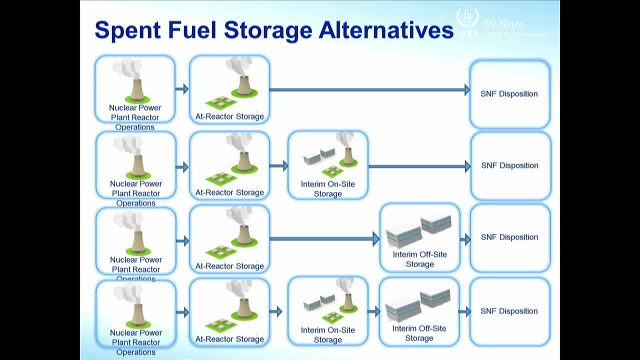 away from reactor- sometimes hundreds of kilometres far away before the final disposition, or could be stored at reactor and then to be moved to an interim storage on site and then to be moved to an interim storage off site and then go to final disposition. 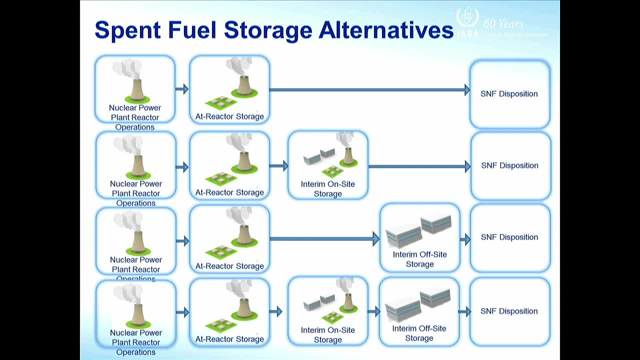 So these are the different options so far to storage the spent fuel. How many years in interim storage? Oh, There is no definition of interim storage. so far It's considered 60 years, around 60, and now it's considered longer. 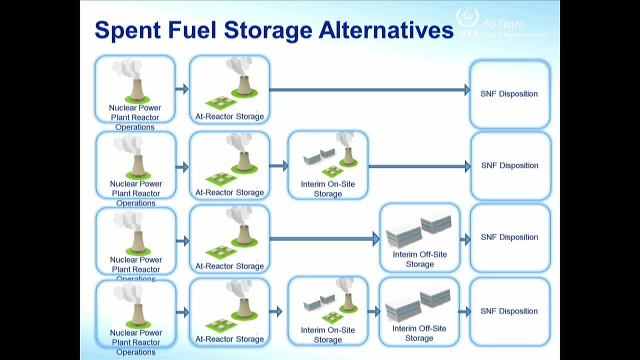 because only few countries have facing in a short term the final disposition. So many countries need a period of around 100 years to have a final disposition ready. So interim storage now. the facilities are licensed for 60 years more or less. 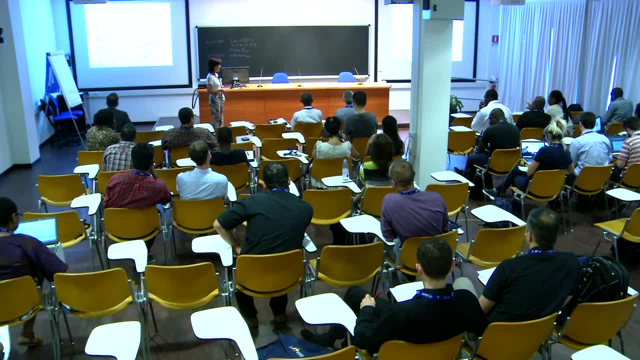 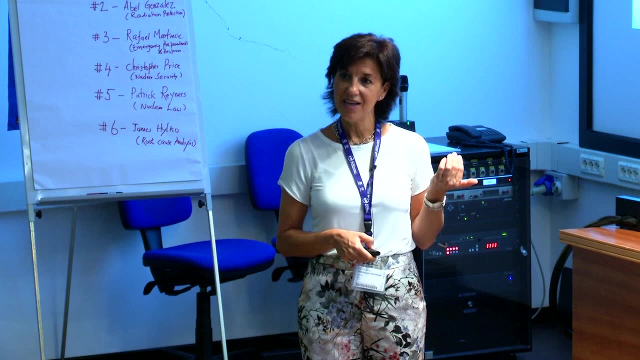 So on site? you mean on site or away? Ah, on site. On site it depends on first the lifetime. in principle is the lifetime of the nuclear power, because on site is in the pool of the reactor and it's around 40 years. 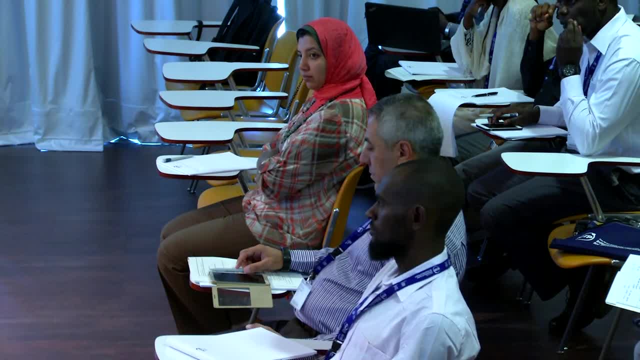 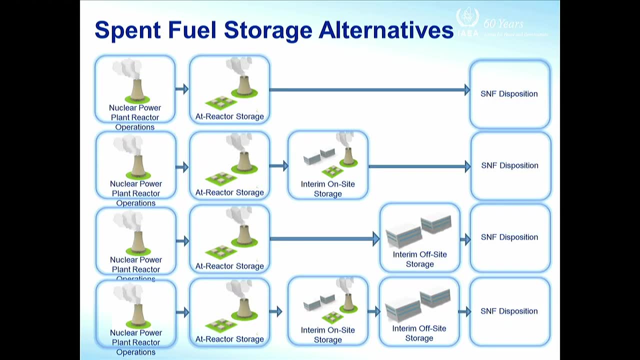 and now is the license period of the lifetime of the nuclear power, And we will see some examples of nuclear powers in the United States, for example, that after the nuclear power plant has been shut down, the pools has to be emptied and the spent fuel was moved. 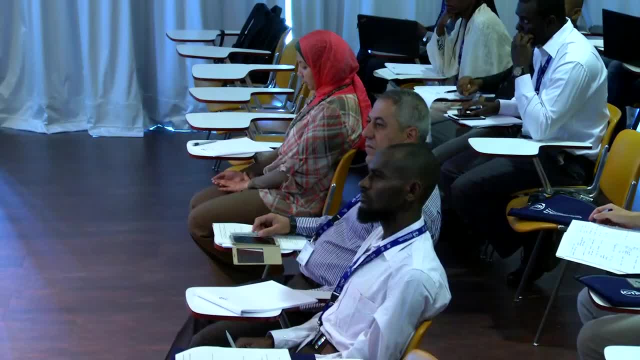 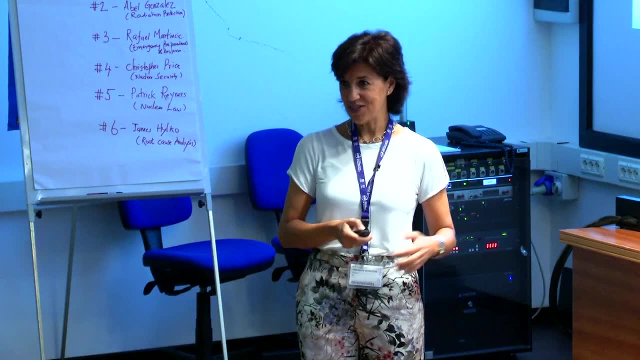 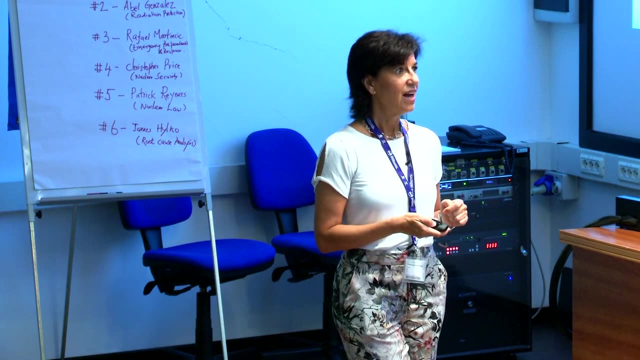 to an interim storage on site- dry storage- and we will see a picture of a power plant completely dismantling and the dry storage remain on site. So it happened now in the United States And it's a it's a problem. 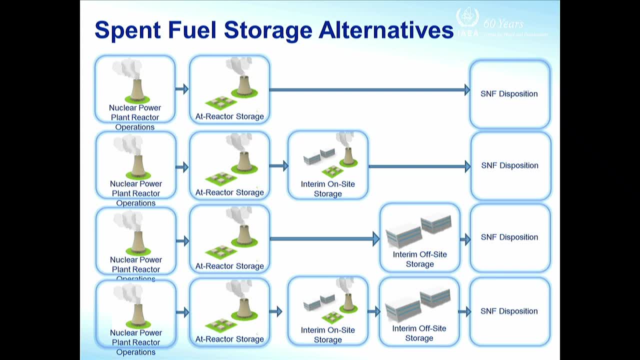 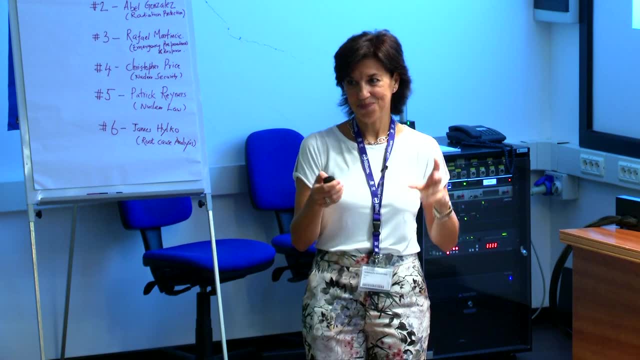 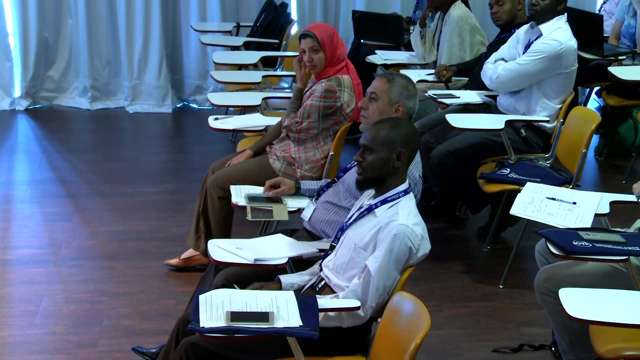 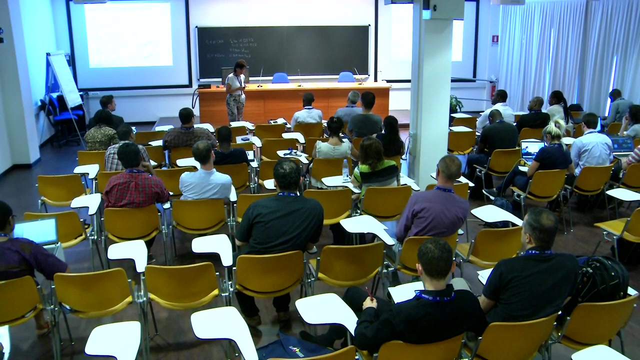 because at the end the country has different interim storage spread around the country, So it's an issue Sorry In the in the world. We will see at the end of the presentation what is the status. So 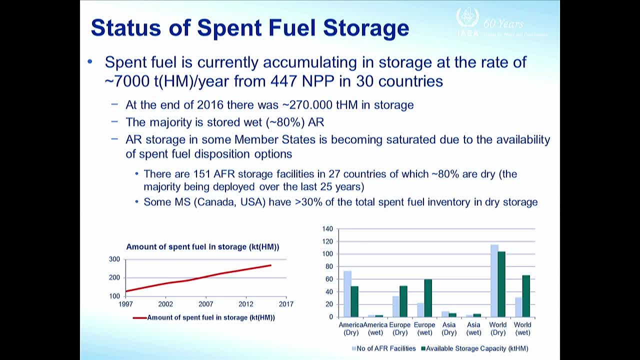 what is the current situation of storage in the world? So every year is around 7,000 tons of heavy metal discharged from reactors. that goes undergoes to storage from the 447 nuclear power plants in operation in 30 countries. So 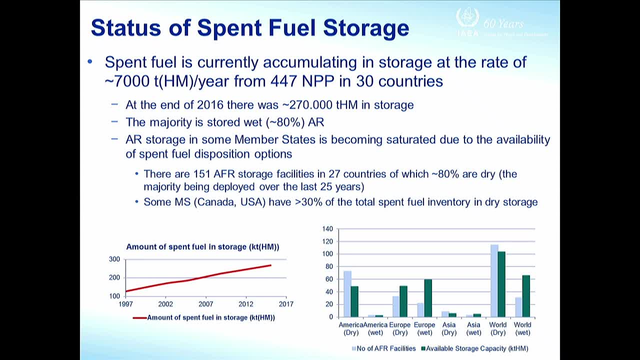 at the end of 2016,, there were 270,000 tons of heavy metal in the storage and the majority are on site at reactors- the 80% And. but what's happened? now most of the nuclear power plants are reaching the end of the lifetime. and most of the pools are full. So the nuclear power plants needs to to find a solution, and some countries have decided to start dry storage on site also. So there are so far 151 away from reactor storage facilities. 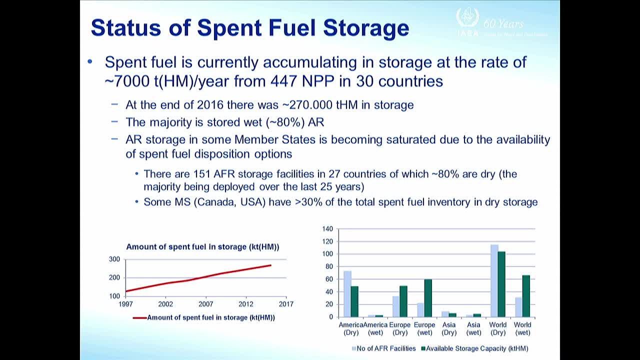 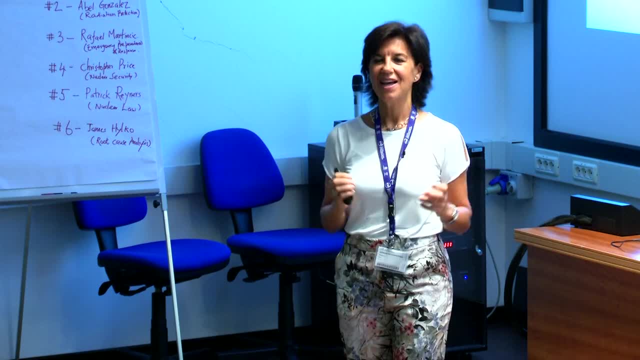 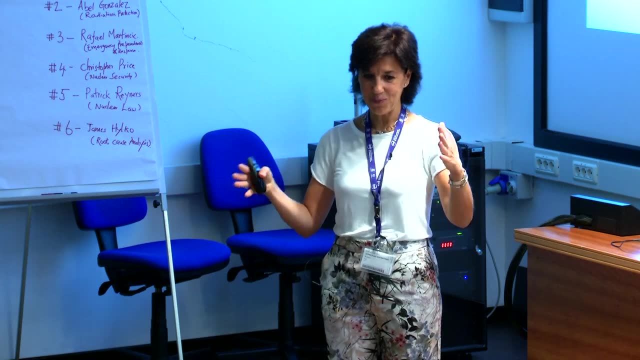 and this name is a little bit confusing because if we, if we speak properly, at reactor means in the building of the reactor. That's why I mean at reactor, So the pool is at reactor building. And away from reactor also mean on site. 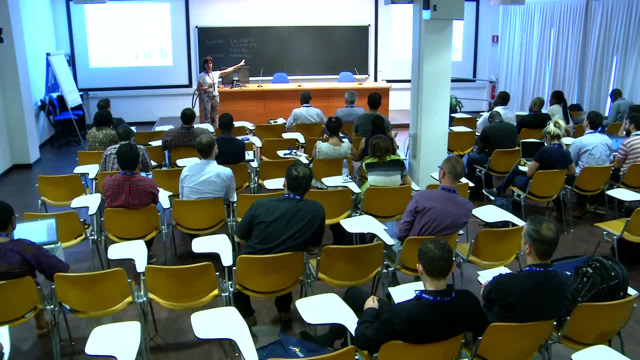 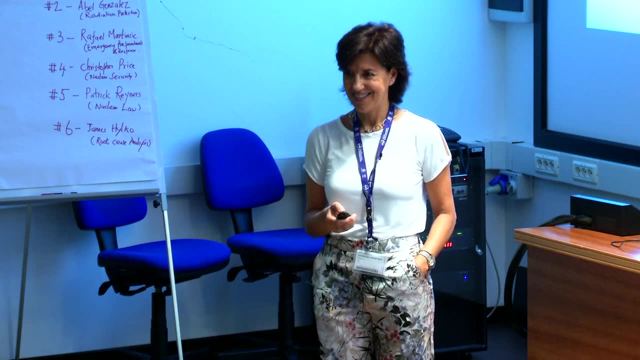 but not in the same building, And also mean away from reactor, far away. So away from reactor means could be on site and could be outside the containment, But could be on site, but also 100 kilometers far away, Yeah, So 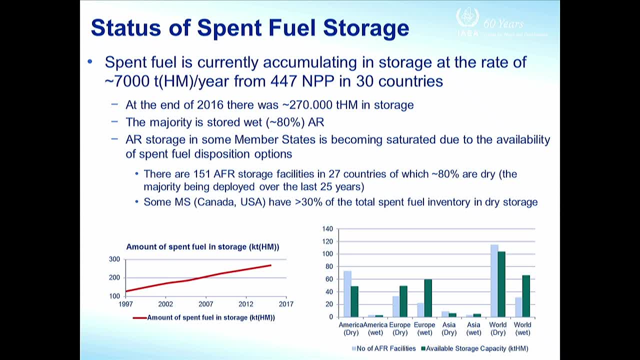 so the the new storage facilities. that doesn't mean the pool under inside the containment building. So now so far we have 151 away from reactor storage facilities in 27 countries, And 80% of these facilities are dry storage. 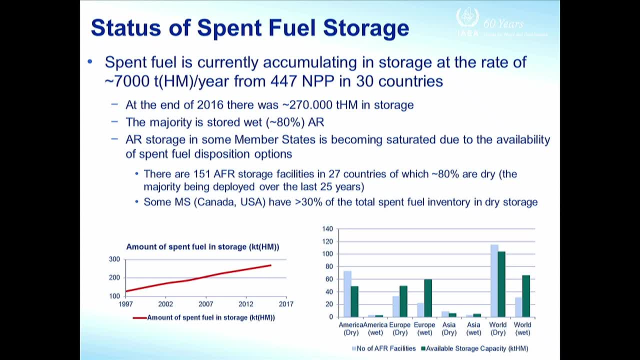 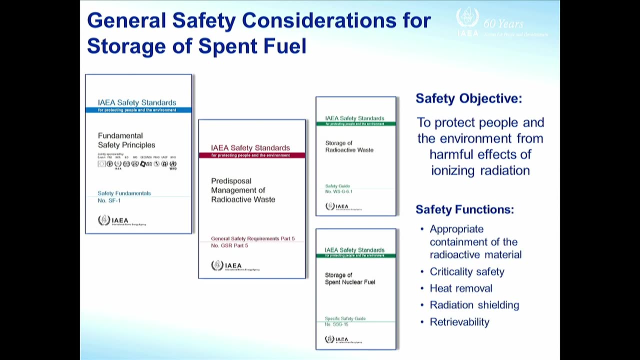 And most of them have been deployed for more than 25 years. So some member states, such as Canada, United States, have more than 30% of the total spent fuel inventory in dry storage. So there are. I think you have received. 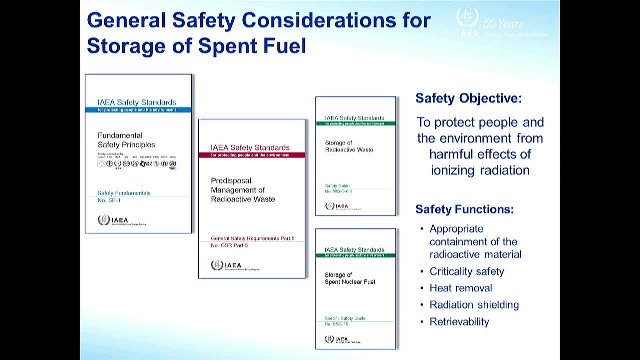 a lot of information about safety standards And all this. the storage facilities and storage activities has to meet the requirements, safety requirements- And there are two specific safety guides. One is safety guide WSG 6.1. It's the storage of radioactive waste. 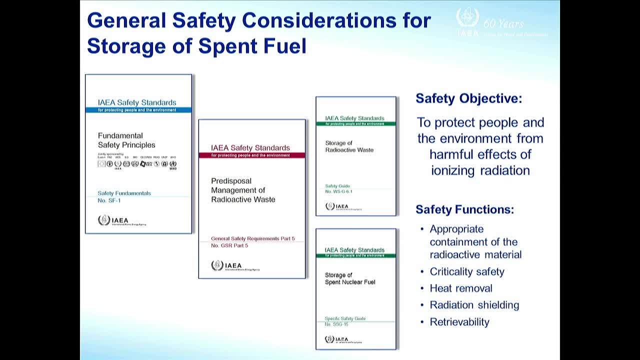 And the other is the specific safety guide 15. And it's main- and it's referred to the storage of spent nuclear fuel- And the main, the main objective of safety is to protect people, environment, from the harmful effects of the radiation. 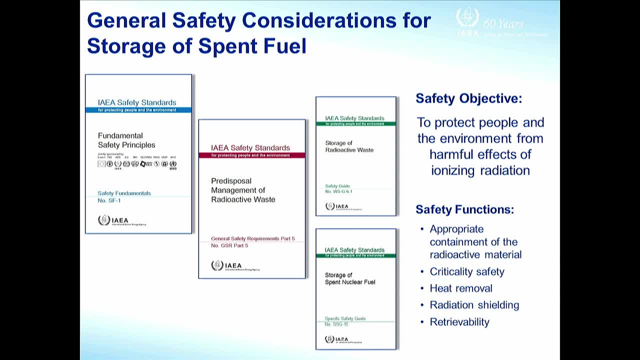 And the storage systems has to meet the safety functions. So they have to give appropriate containment of the radioactive material, And the first barrier is the pellet. The second barrier is the fuel assembly And then there is the also the canister. 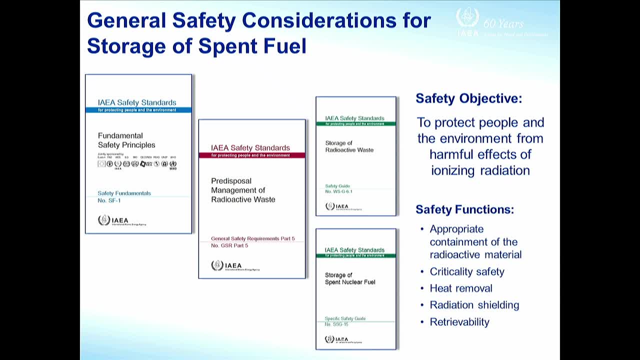 and the casks to to keep the radioactive under control. So the system has to be critical, safety against criticality, So it can never occur that it leads in a configuration that can be critical. It has to have effective heat. 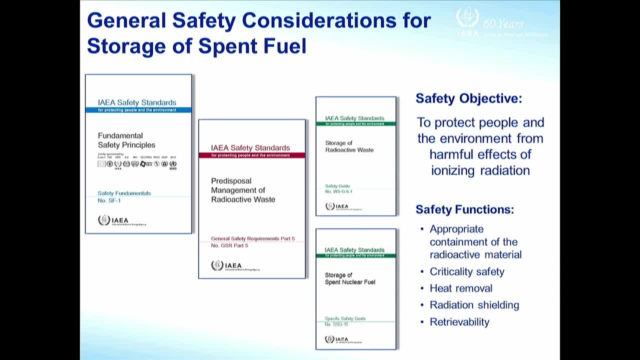 decay, heat removal And in the case of the pool, the water is the coolant And in the case of dry, is the natural convention convection. And it also has to ensure that the dose for workers and also for the public. 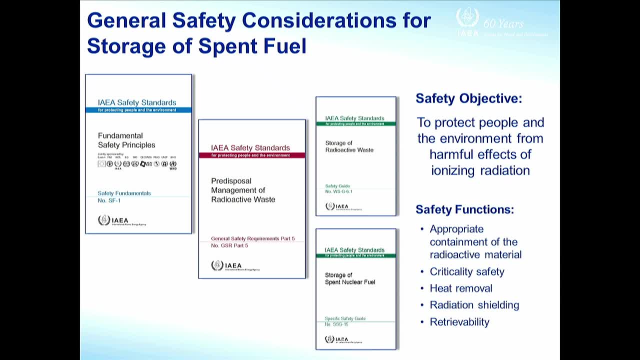 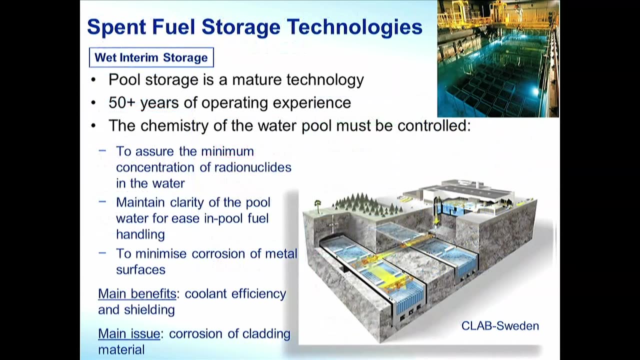 remains under the limits And also has to ensure that the of the spent fuel to undergo to the next steps of the spent fuel management. So we have talked about to store the spent fuel and the water. So the pool storage is a mature technology. 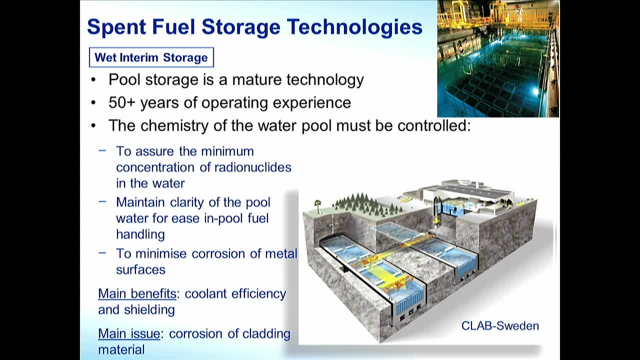 since it's been used from the beginning of the nuclear power generation And we have accumulated more than 50 years of operating experience. And, as we said, the chemistry of the water has to be strictly controlled to ensure the minimum concentration of radionuclides. 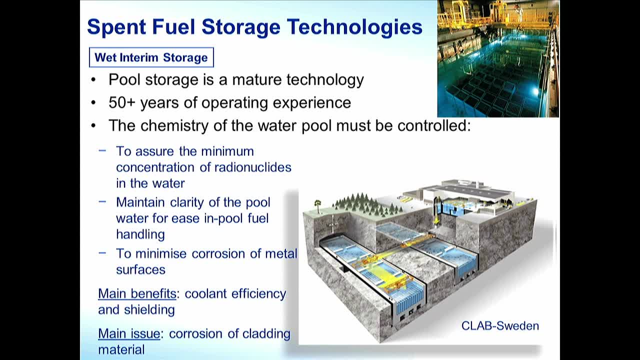 in the water to keep the clarity for inspection and to minimize the corrosion of the metal surfaces, the rods and the fuel assemblies. So the importance of water is because the water gives the coolant efficiency and shielding, the biological shielding And 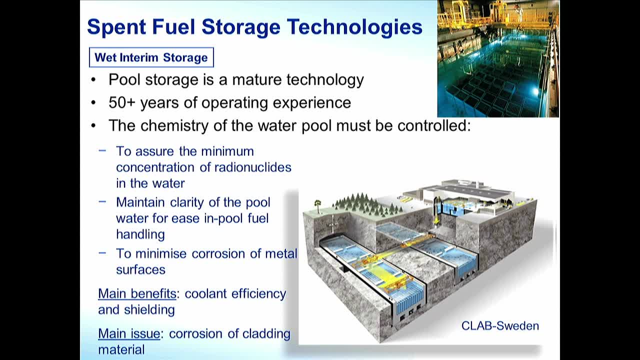 the main issue is: the water always provokes corrosion, So we have to keep the water under strict conditions to prevent the corrosion of the metal parts. And this is the CLAP concept in Sweden, because they decided to storage- the interim storage of water. 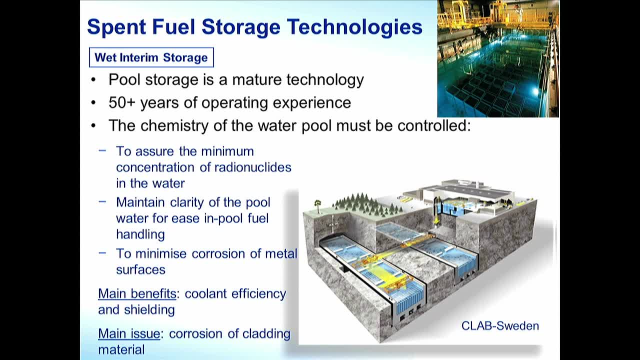 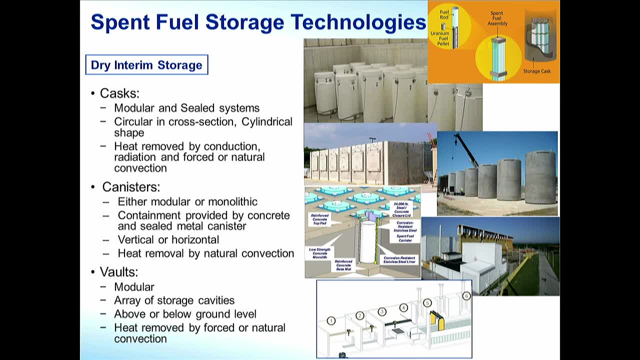 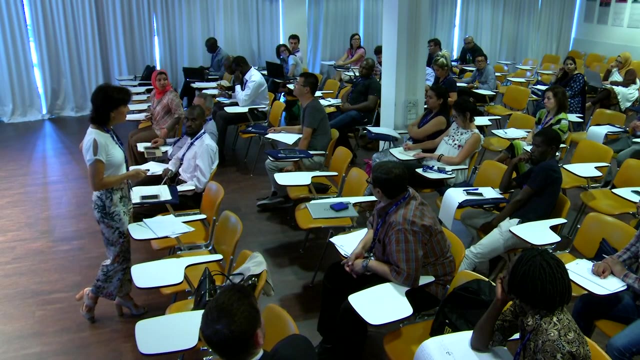 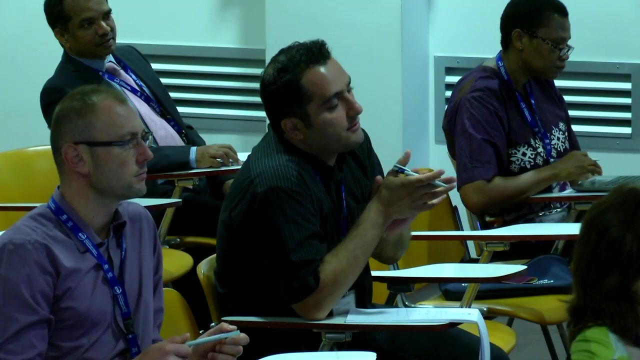 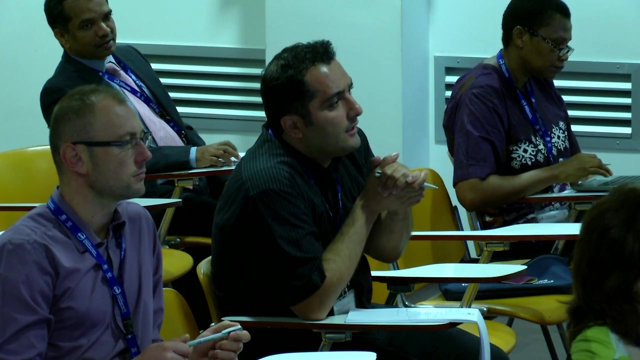 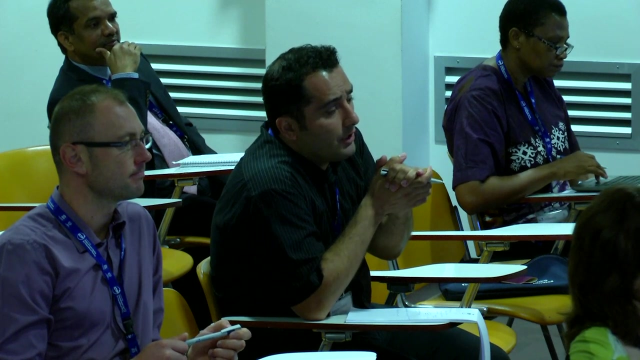 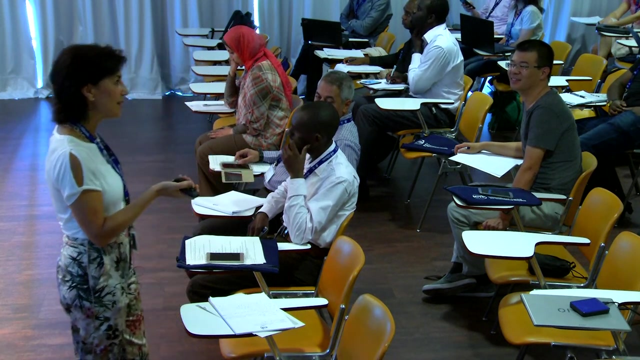 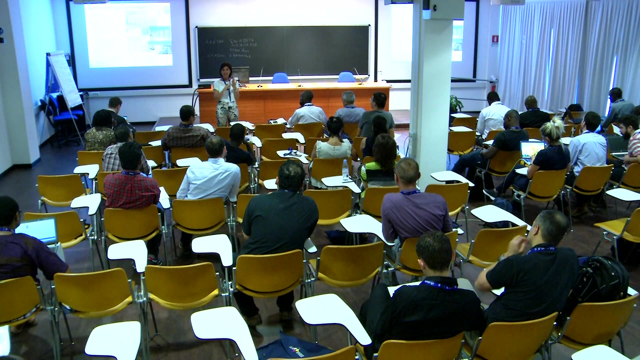 and it's away from the reactor. and instead of using dry storage, they use water storage. Sorry, Of course, because the water, if you put something in water, is corroded, So you have to. it's first of all, it's deionized water. because the presence of different ions can provide corrosion: Chlorine for example, and the ions we have in the normal water. So first the whole pool is full by deionized water to prevent the corrosion, And also you can. 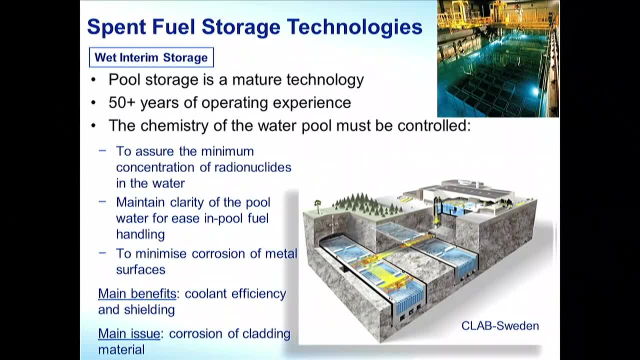 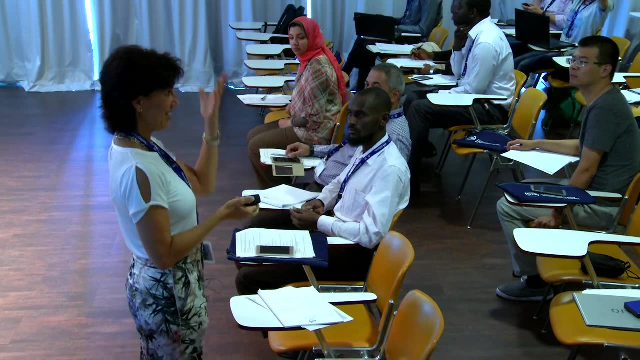 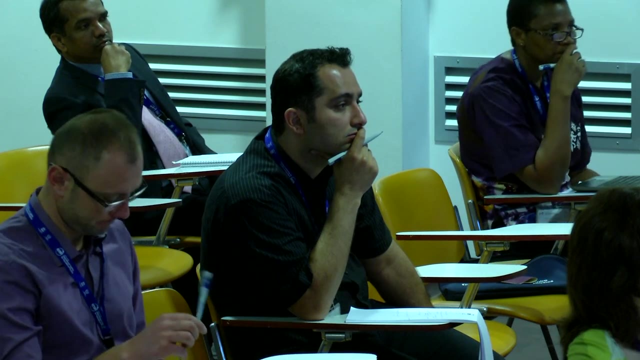 control. it's very if you see under control still water, you have bacteria very easily. So you cannot see. and it's not clear the water, so you cannot see. you cannot inspect visually what is the status of the fuel assemblies. So the bacteria 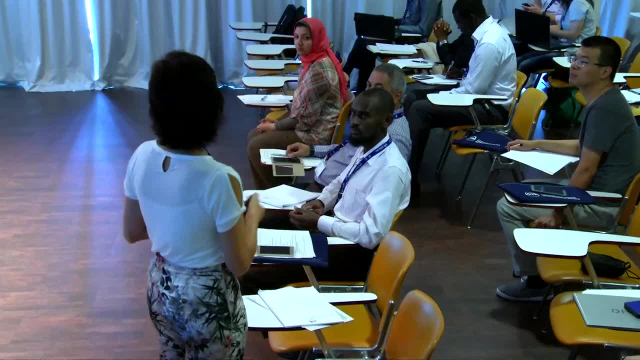 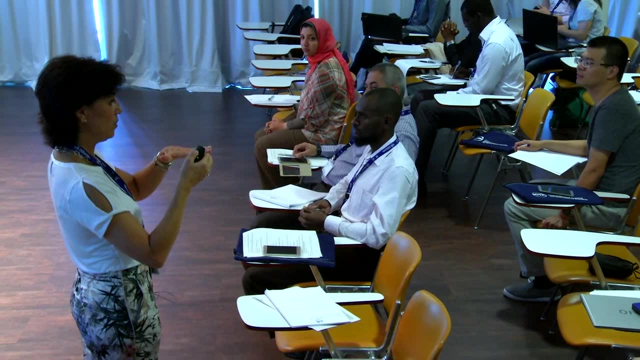 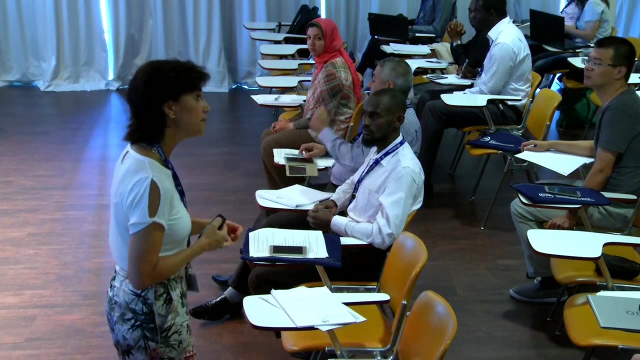 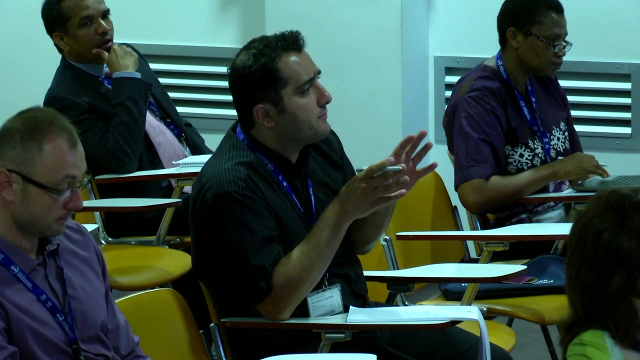 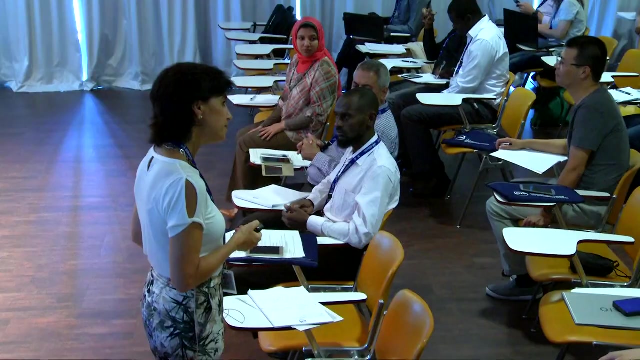 also the bacteria corrodes everything. So in one hand you have to prevent corrosion is the most important thing- and you have to also to prevent the levels of boron. for criticality controls for neutron absorbers: Yeah, the fuel assemblies is directed, you can see. 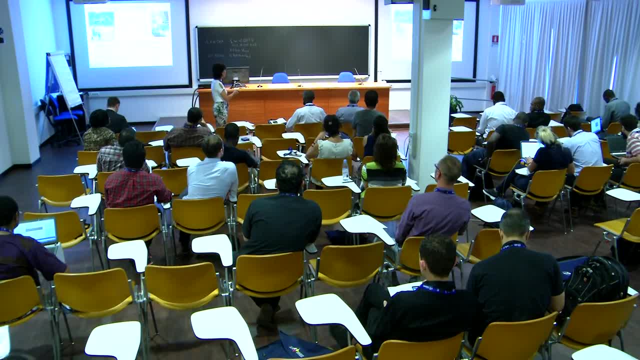 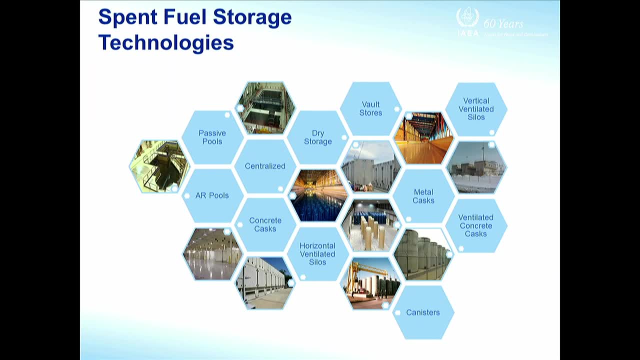 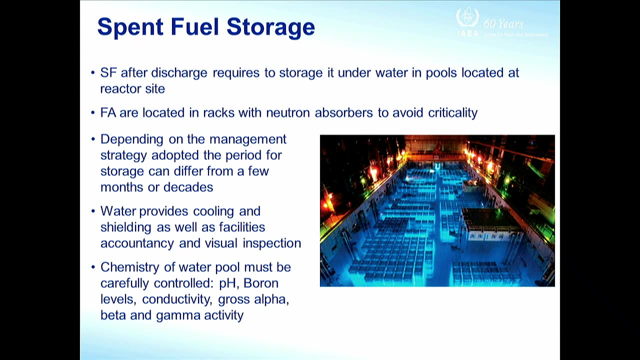 I think it's better seen in the other picture. Here You can see this is the fuel assemblies Only puts in how you call these, in racks. so it's not without any containment. So this is a rack and the fuel assembly is put like this. 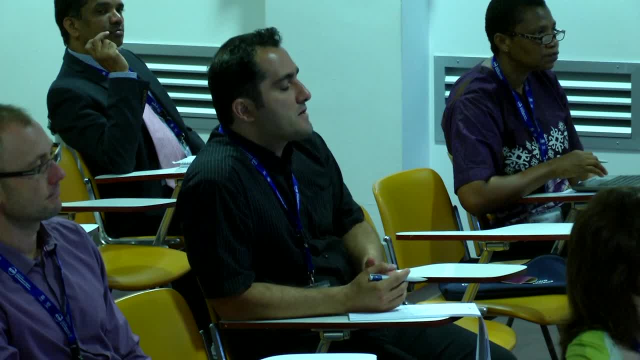 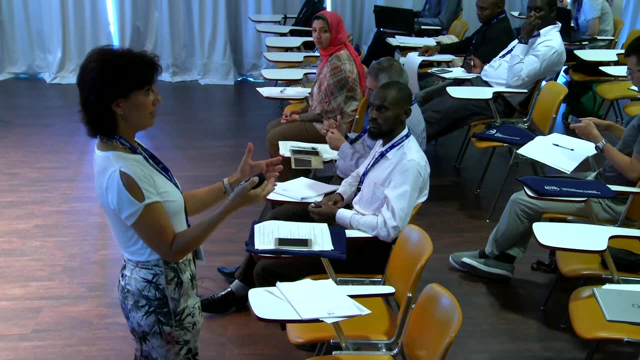 directly in the water. So that's why you have to prevent all corrosions and also it's a way to control the radioactivity in the water. So you cannot have a concentration of radioactivity in the water first for the workers and also. 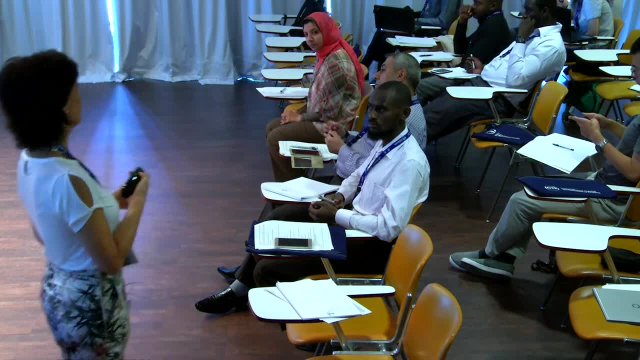 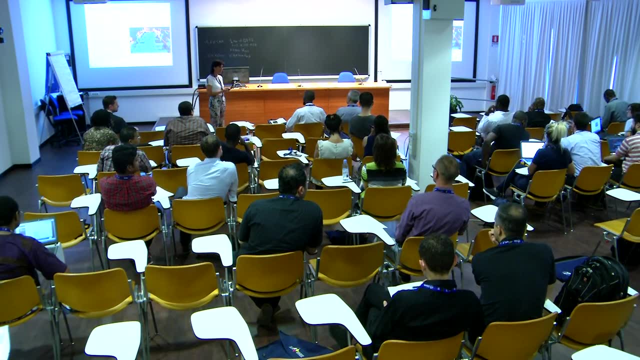 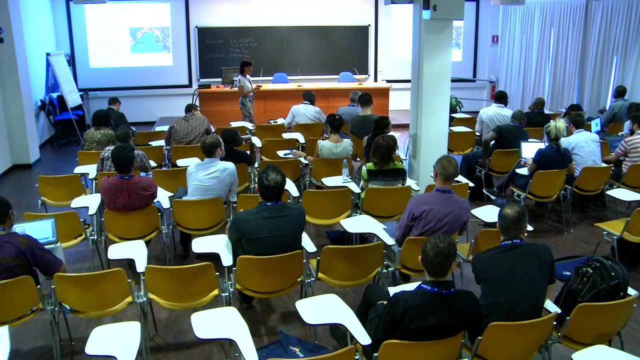 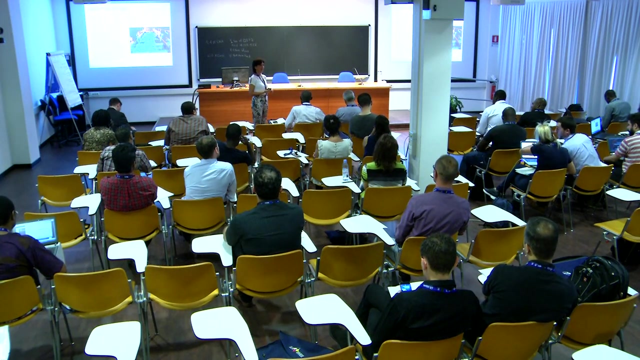 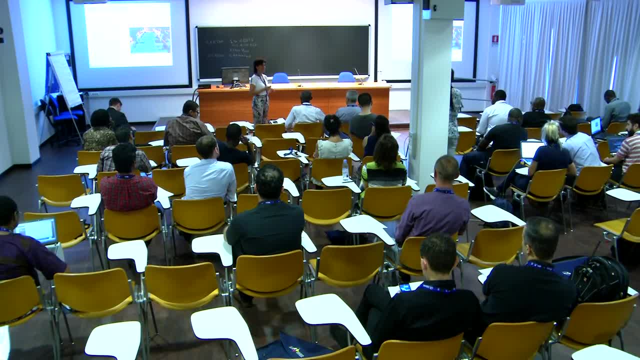 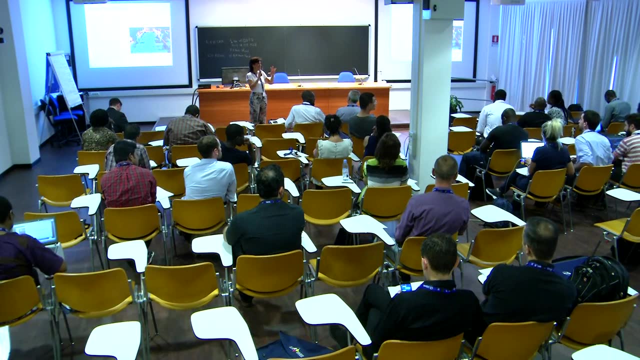 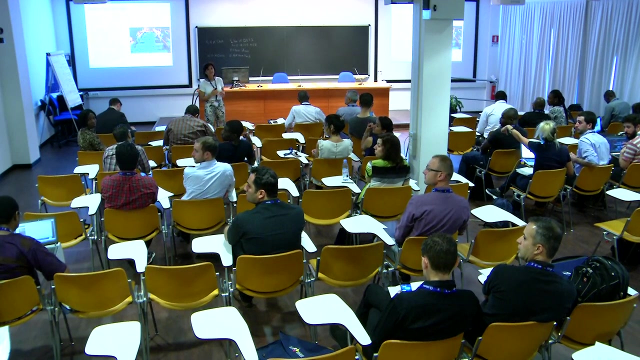 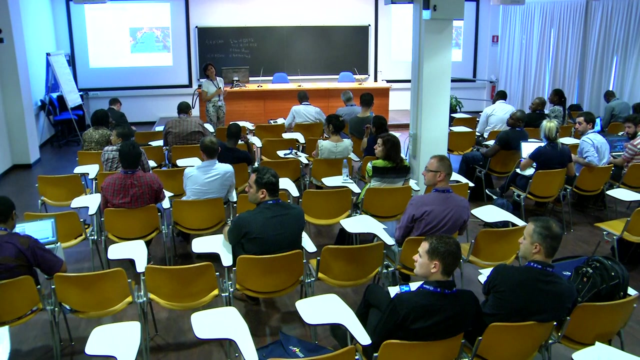 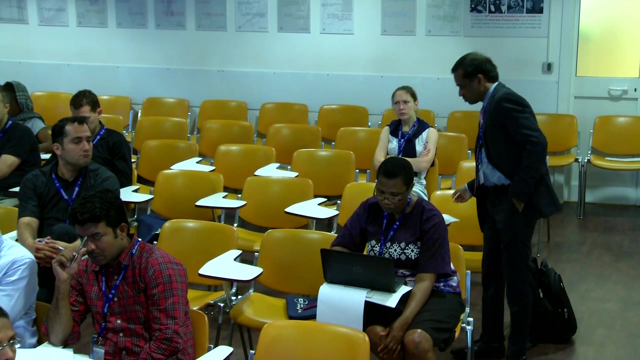 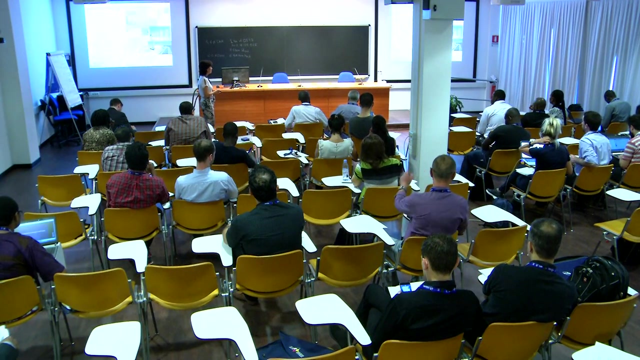 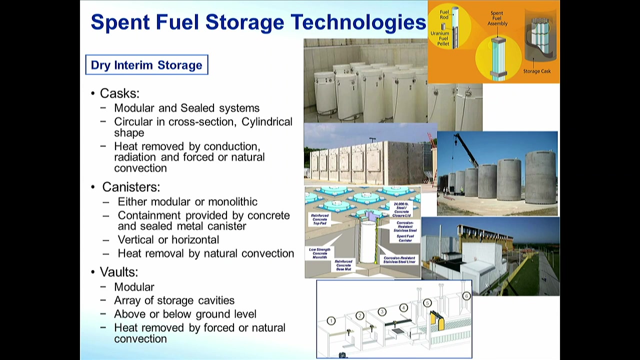 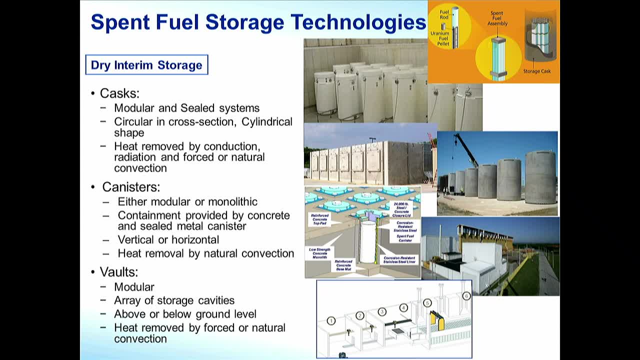 are modular and also can be monolithic And they are circular. the casks in the cross section and the heat, the decay heat, is removed by convection, a natural convection, And in the case of canisters they can be vertical or horizontal And the bolts are buildings. 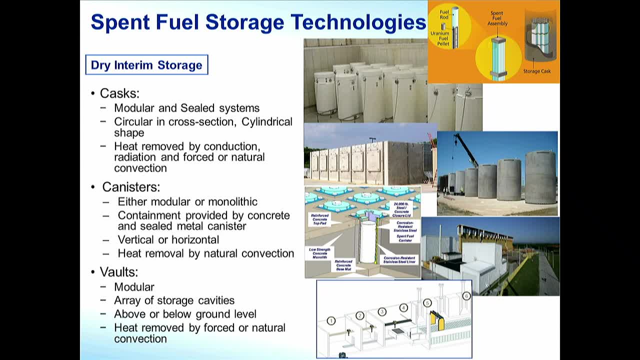 that are also modular, so can be added more and more or rise of cavities, and can be above or below ground level. Also, the canister can be both or below ground level 00.076. But in truth buildings has more and more. 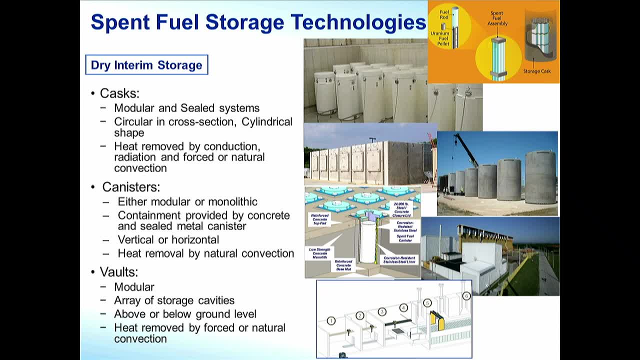 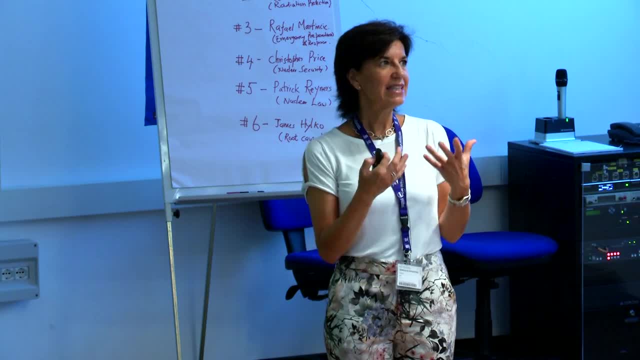 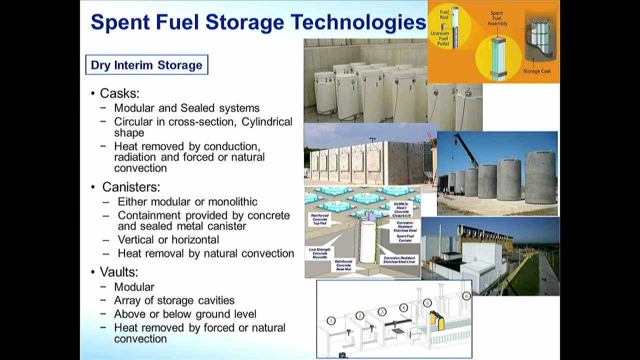 The main benefit of the dry storage is: this is a passive system, so it doesn't need any active systems, so the system is controlled by itself And in the case of the water of the pools, now there is a lot. after Fukushima, there is a lot of work done and performed trying to find solutions to make the pools more passive than they were before. 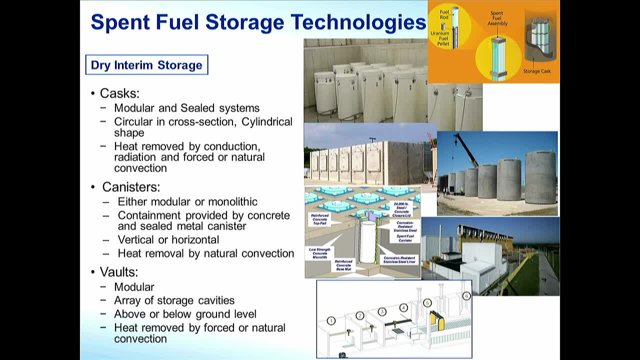 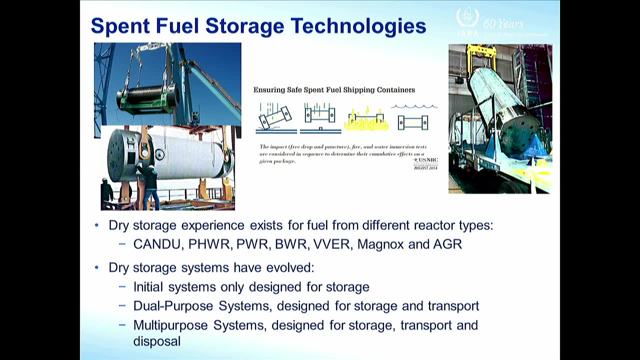 So the goal is to have the most passive systems for storage. So the dry storage options and technologies have been applied to all different types of spent fuels, And the dry storage technologies have evolved since their conception, And at the beginning they were only designed for storage. 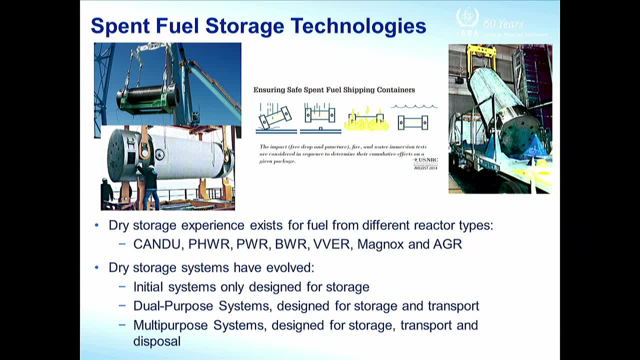 But today they are designed for storage and transportation and they are the so-called dual-pull-post casks And the idea is to design multiple systems to be licensed for storage, transportation and also for disposal. So the idea is not to Once the spent fuel is placed in the casks and the cask is licensed for all the stages, it's to avoid additional handling. 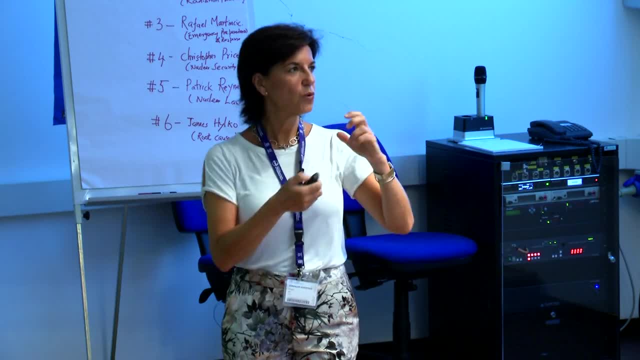 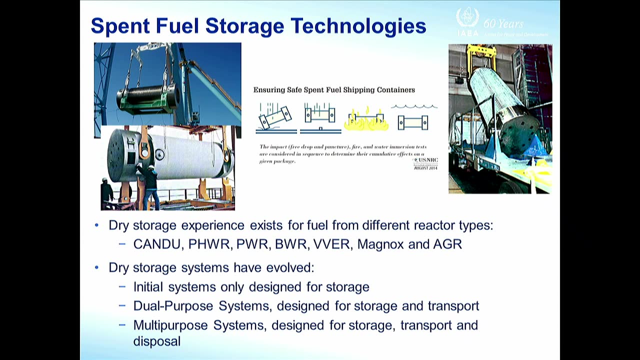 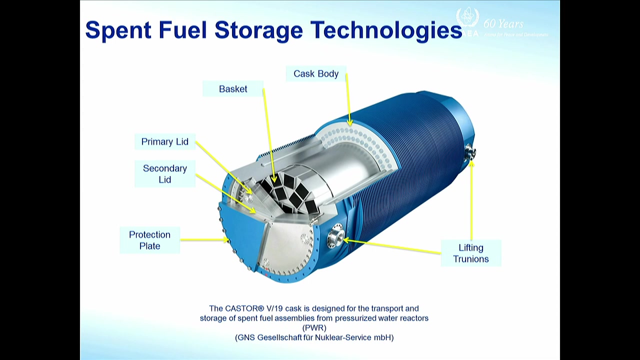 additional sillage to open the casks to handle the spent fuel from one cask to another cask. So the idea is to simplify the process, to avoid manipulating too much the fuel assemblies. So this is an example of a cask store, a cask designed in Germany. 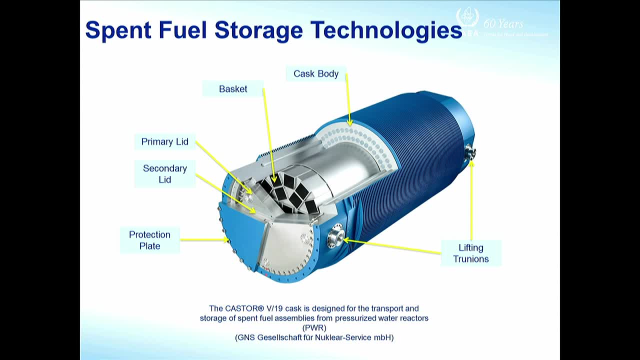 So you can see the fuel assemblies. this is the basket for the fuel assemblies And there are many layers outside with neutron absorbers to prevent the dose And the spent fuel inside the cask is around 300 Celsius degrees more or less. 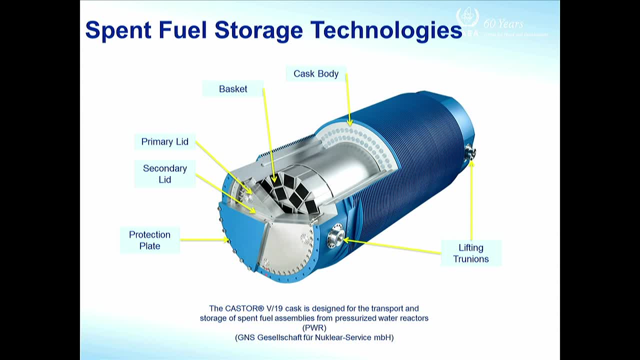 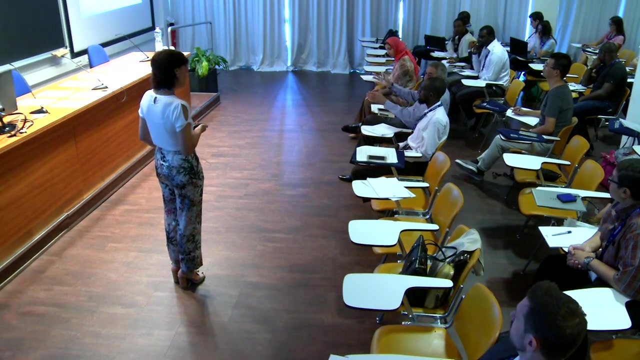 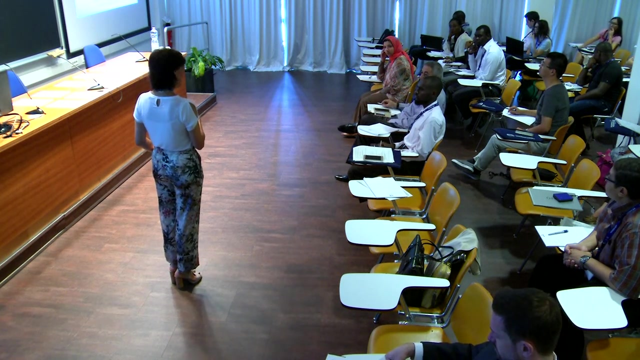 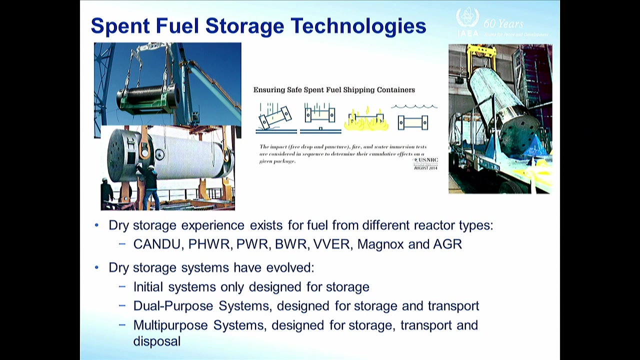 And the decay heat is eliminated by natural convention And there are some layers and lids to close the casks. Some are bolted and also welded. So this is the main issue now: To find a way to license the casks. The cask for the three stages is not that easy. 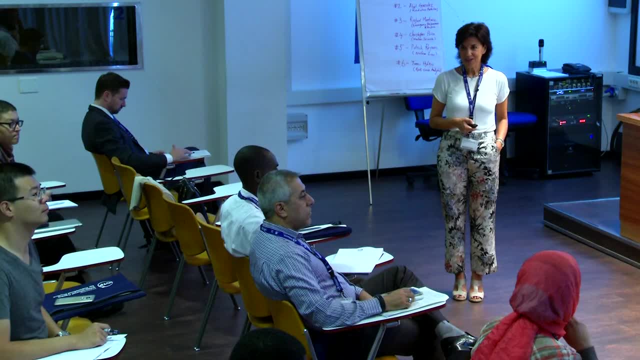 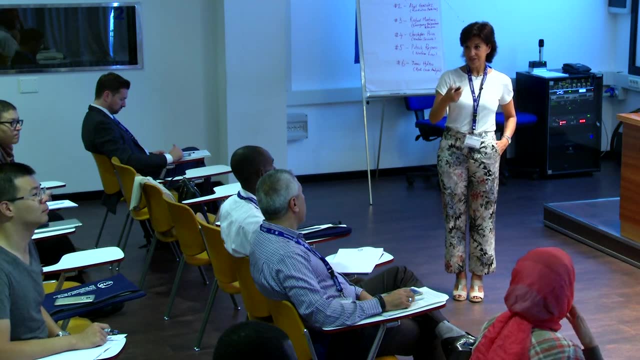 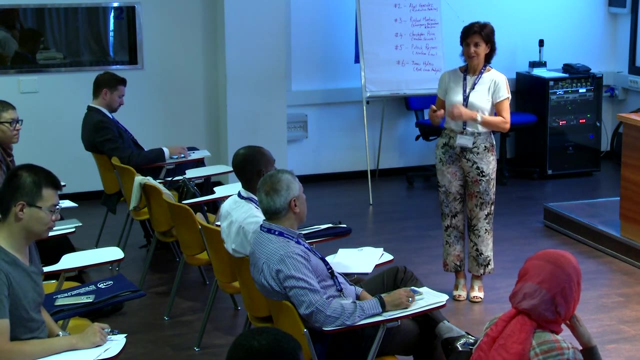 So this is the main issue, Because then you don't need to retrieve the spent fuel from the casks used for storage and transportation. So if it's licensed for disposal too, you can use it to be disposed. So you don't need to retrieve the spent fuel. 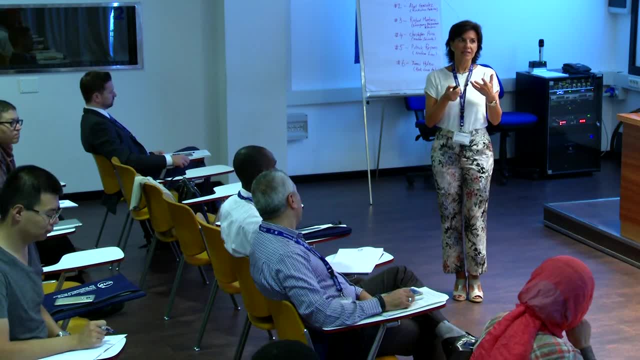 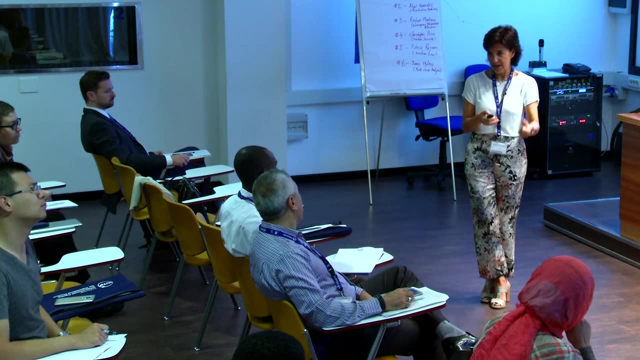 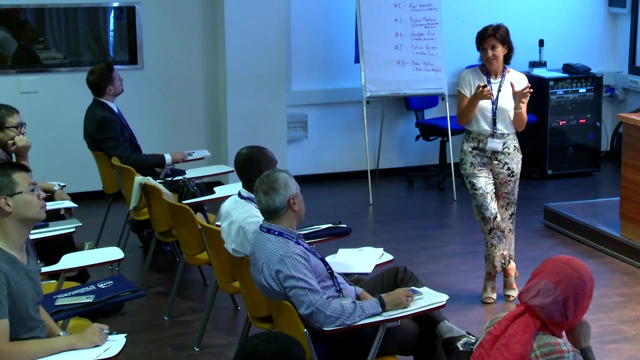 That is a very It's difficult, but also it's a source, A source of damage in the fuel assembly If you have to handle, after 30 years of storage or 60 years of storage, So you have the same cask licensed for disposal. 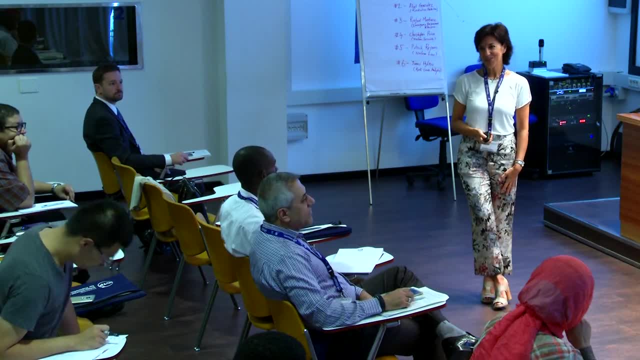 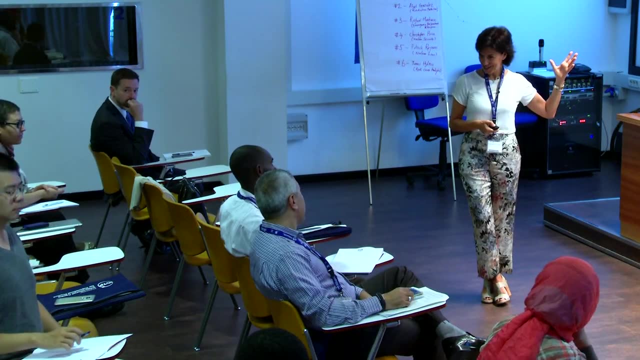 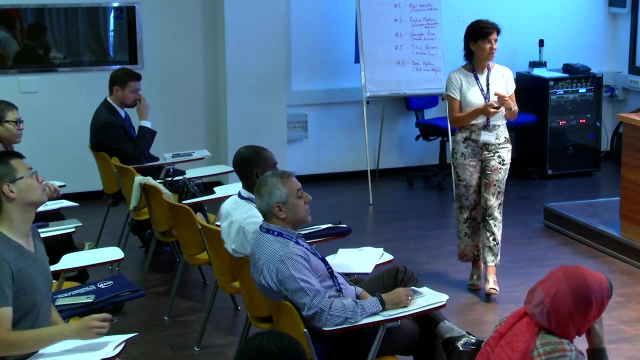 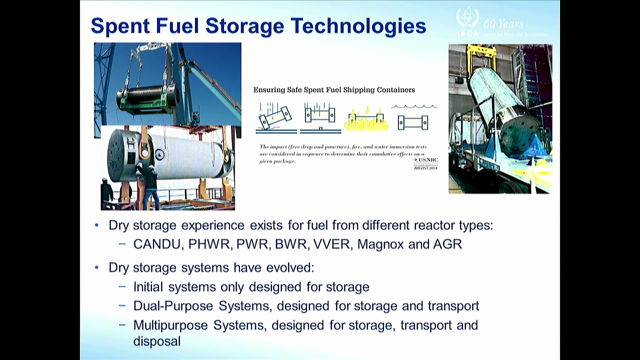 And this is the issue: how to get the license, How to ensure that a system that was licensed for storage 60 years ago is still valid to be disposed. So now we, for example, in our section, In my team, we are starting working in transportation issues for casks after a long period of storage. 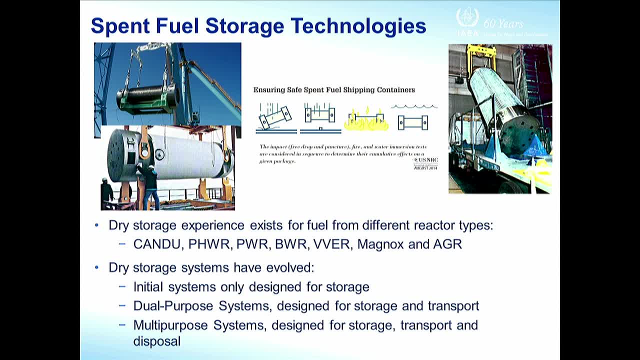 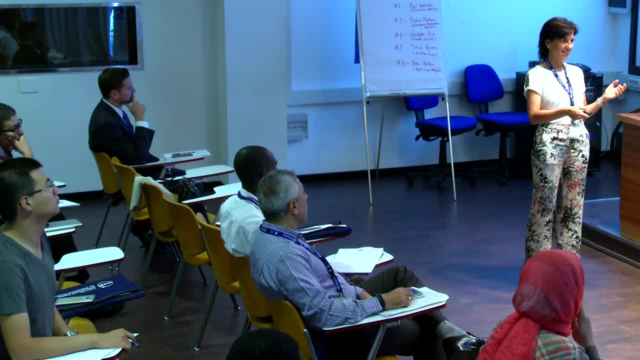 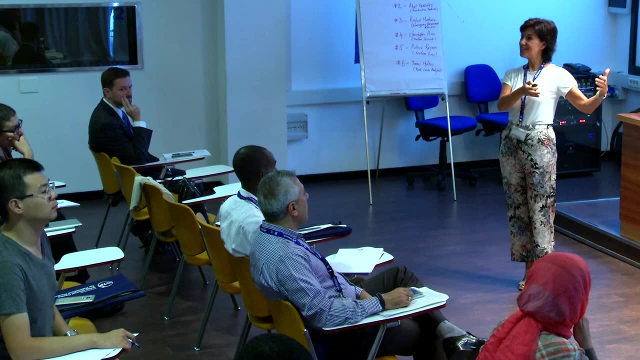 Because some of the casks- the dual-purpose casks, have been licensed for storage and transportation. But you store the casks in the nuclear power plant and you transport, But what's happened after 60 years of storage in the interim storage and you have to transport these casks to the disposal facility. 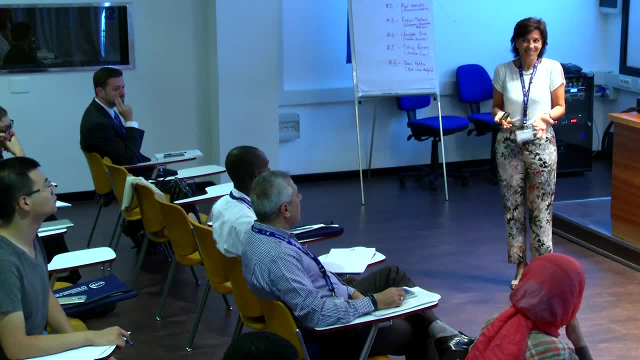 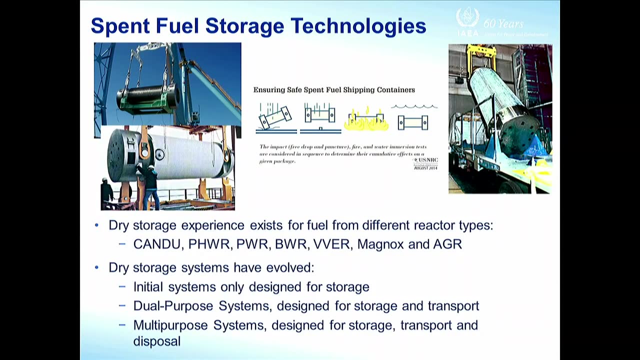 Even to retrieve, But what's happened after 60 years? So now we are working in this type of issues And there is an international group in safety dedicated to dual-purpose systems for the license To find the requirements and all the aspects and parameters to be taken into account for the license process. 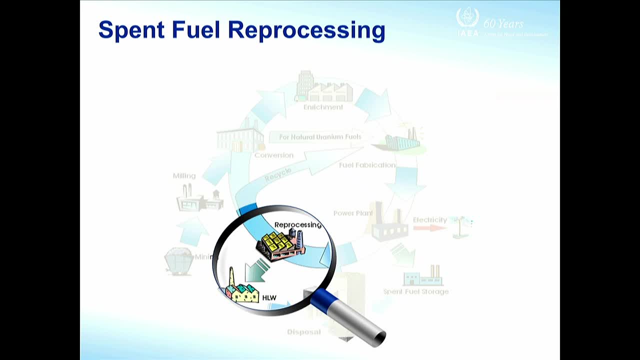 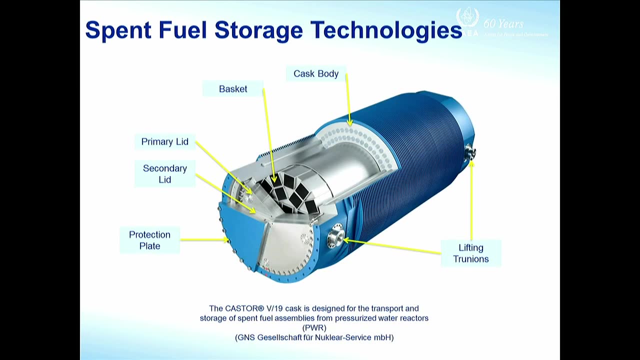 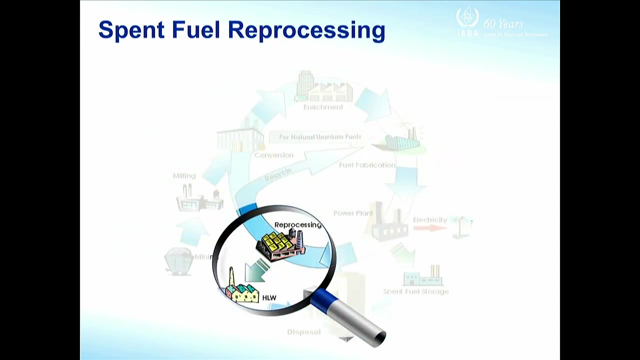 So so far it's when we consider. So once we store the spent fuel, we can dispose, eventually dispose of the spent fuel in the deep geological repository. But for those countries which don't consider the spent fuel as waste, They consider the spent fuel as an asset. 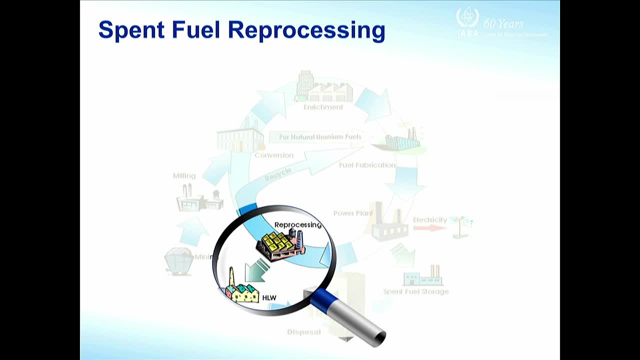 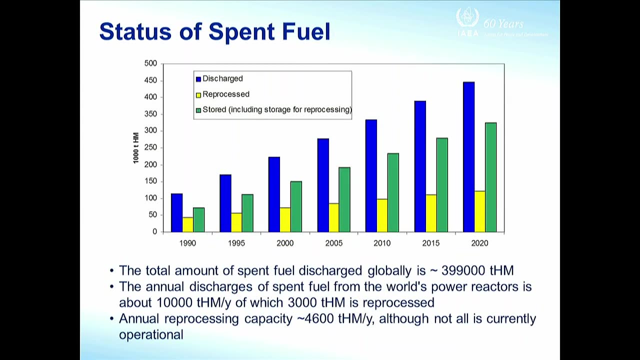 They reprocess the spent fuel to get the uranium and plutonium for recycling. So what is the status? So we talk about the storage, But the total amount of spent fuel discharged globally is around 400,000 tons of heavy metal so far. 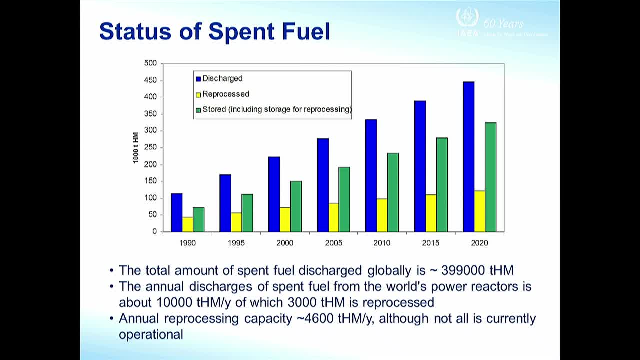 And one-third of this amount It has been or It's under reprocessing so far. So 1,000 tons of heavy metal is discharged every year. 7,000 tons- No, sorry, 10,000 tons are discharged. 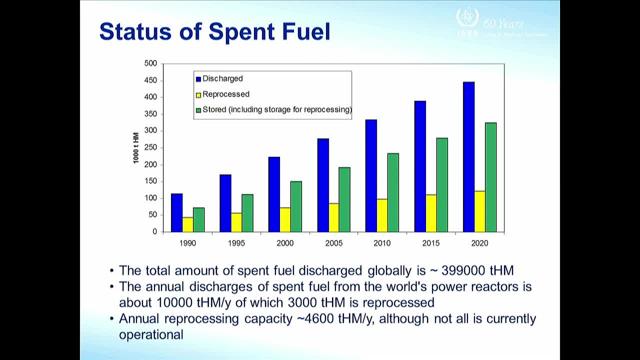 7,000 tons are stored And the remaining 3,000 tons- so one-third- is reprocessed. The annual reprocessing capacity in the world so far is 4,600 tons of heavy metal per year. Although now it's not all is currently used now. 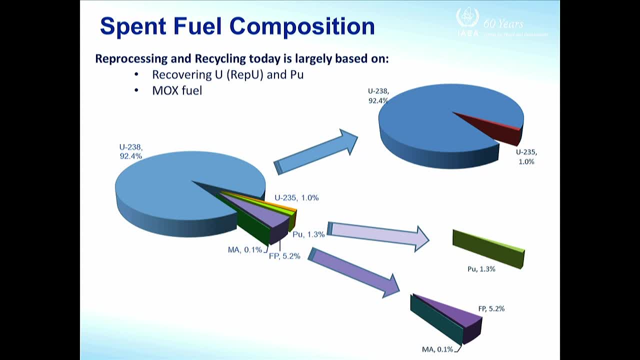 It's not operational. So in which consists the reprocess? Is to To get the plutonium and uranium to be used again as MOX fuel And it's produced a high-level waste. That means The composition is mainly the fission products and the minor actinides. 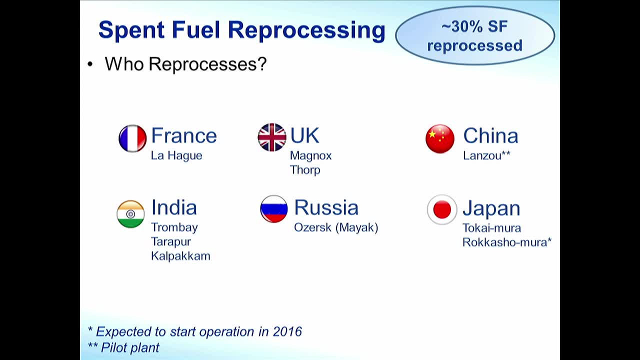 So So far, France, UK, India and Russian Federation are reprocessing. Japan now is. It was four. five months ago. The government clearly said that they will continue going for closing Closed cycle And the Rokashimura is under licensing process. 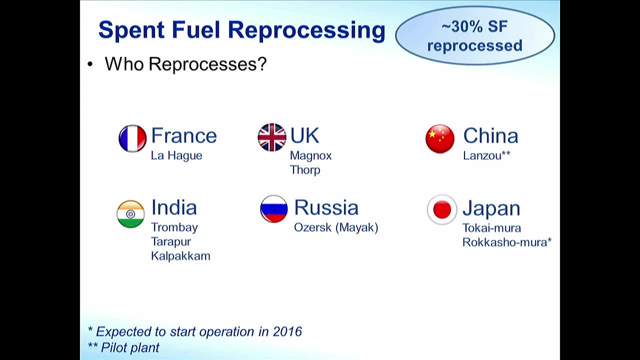 And China has a pilot plan And also it's building, or it's going to build, a new reprocessing plan. But they are facing some Built by Areva But they are facing some stakeholder issues to In the site Decided for. 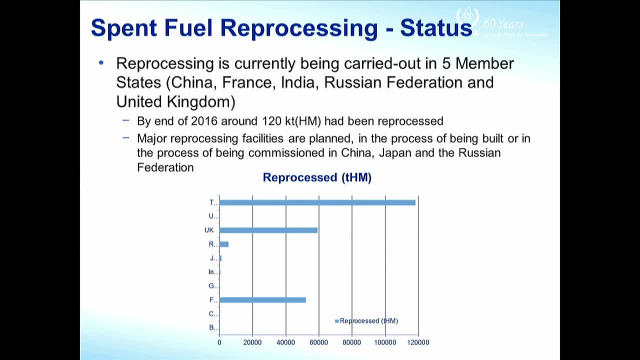 To build a reprocessing plan. So by the end of 2016,, around 120 kilotons of heavy metal had been reprocessed, And the major reprocessing facilities are planned to be commissioned in China, Japan and in the Russian Federation. 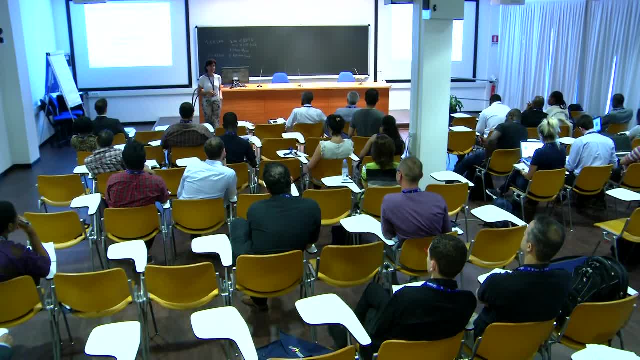 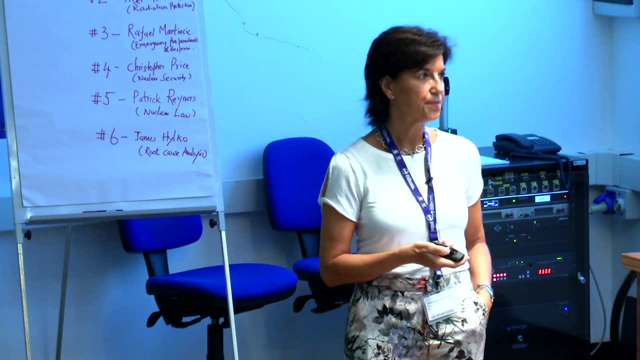 Since UK is going to shut down third plan And also they are going To open cycle, So they are changing the fuel cycle option And they are moving UK from closed cycle to open cycle. So this is the main process for reprocessing. 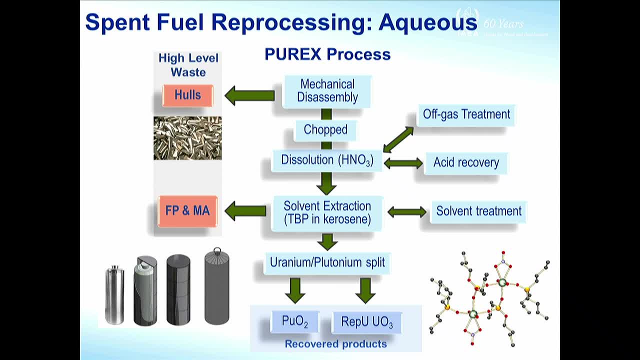 It's the PUDEX process, It's plutonium-uranium restriction And, after mechanical disassembly And the roads has to be shopped And And the spent fuel is dissolved in nitric acid, It's generating an off-gas stream that is treated by. 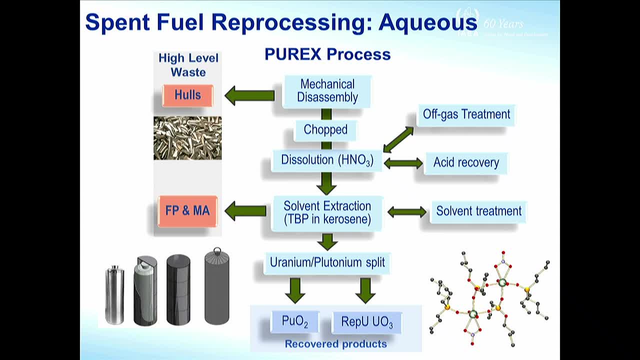 And it's filtered, And mainly iodine and the noble gases produced are trapped, in particular trapping absorbers And the nitric acid. once this is dissolved, It's a stream that has to be Treated, So The acid solution undergoes through solvent extraction. 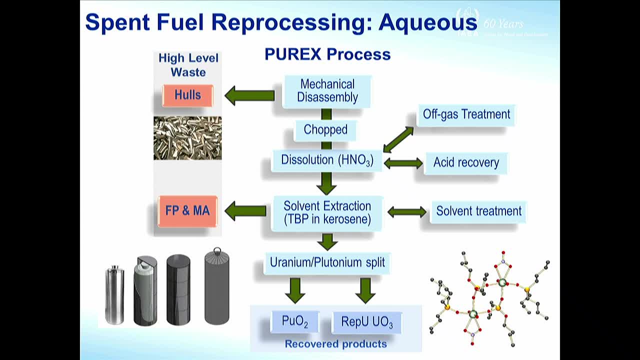 Using tributyl phosphate. This is the molecule In aliphatic diluent as kerosene or dodecane. So Under liquid-liquid extraction Uranium and plutonium are recovered And the rest of the fission products and minor actinides remain. 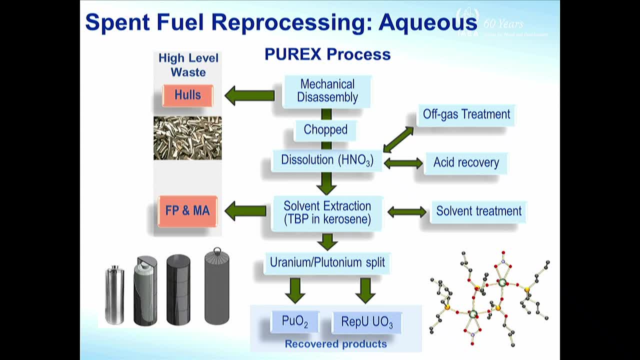 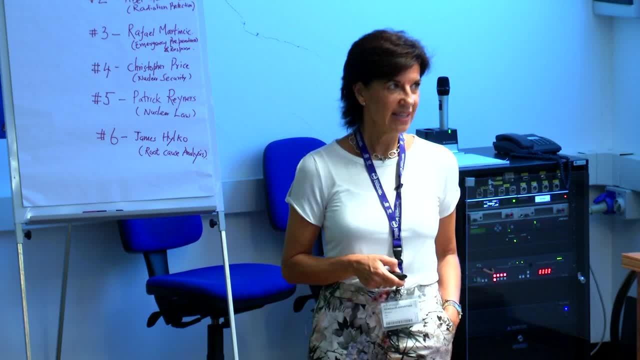 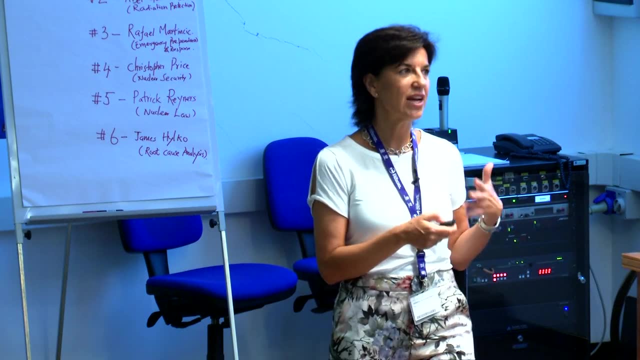 In the high-level waste stream. So the main of the minor actinides are in trivalent state. So that's why they are not extracted by TVP. That only extract uranium in. They only extract in Exavalent and four-valent state. 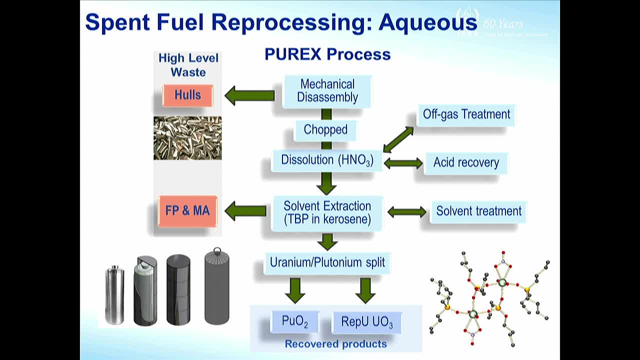 So once uranium and plutonium are recovered From the organic solution, The solvent is treated, Is cleaned And is reused Again In order to not produce a lot of organic spent solvent, Because the organic solutions are very difficult to manage As secondary waste. 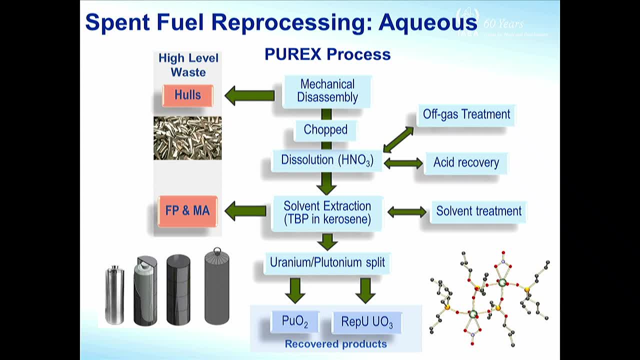 So the, The TVP in kerosene is treated and cleaned To be reused several times. So once uranium and plutonium are recovered, They are split in two streams In plutonium dioxide And the so-called repu uranium, And they are stored for. 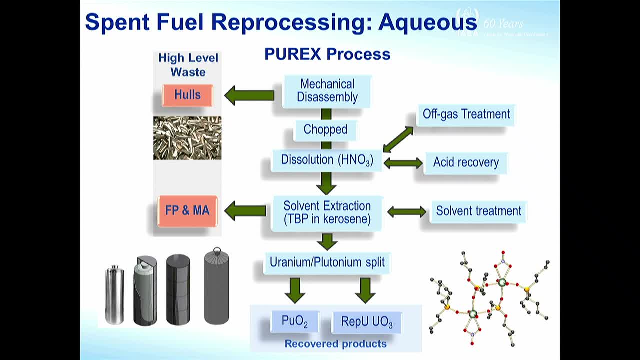 Further use. So plutonium is mixed with depleted uranium Or natural uranium To produce MOX fuel And so far repu is stored To be used In the futon. TVP is tributyl phosphate. It's a molecule. 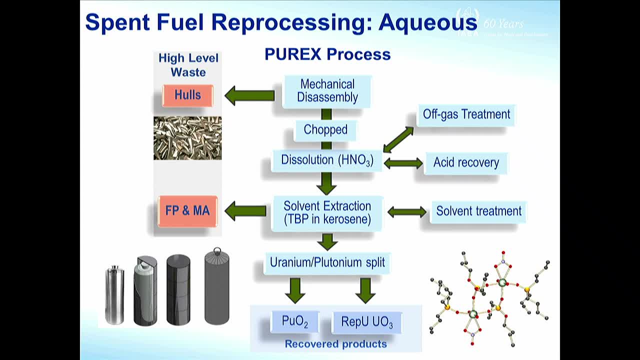 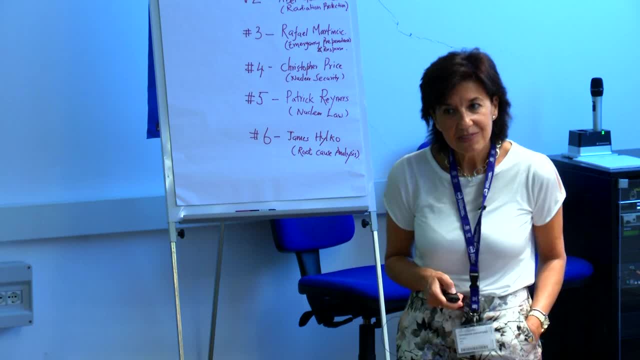 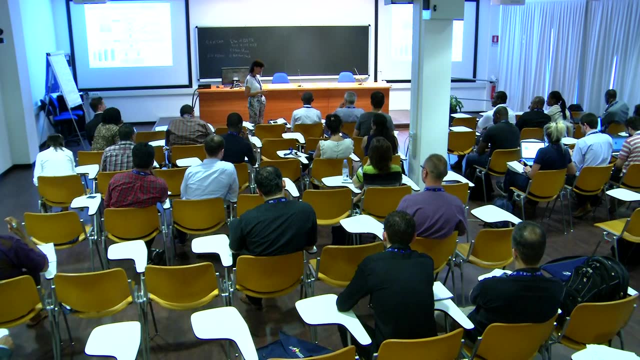 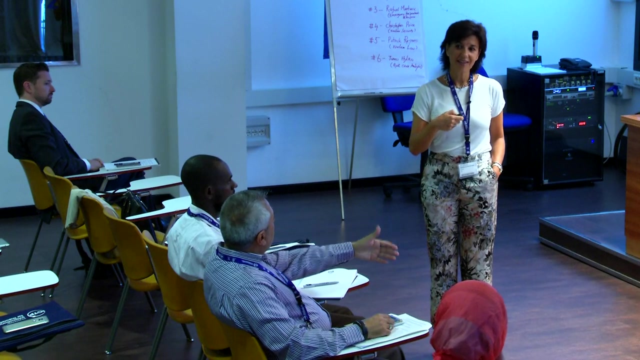 It's a phosphate With three butyl chains- Sorry, MOX fuel. So you mean it reprocesses the fuel. When you send your fuel, You will receive the radios If you run, And your record is designed for that. 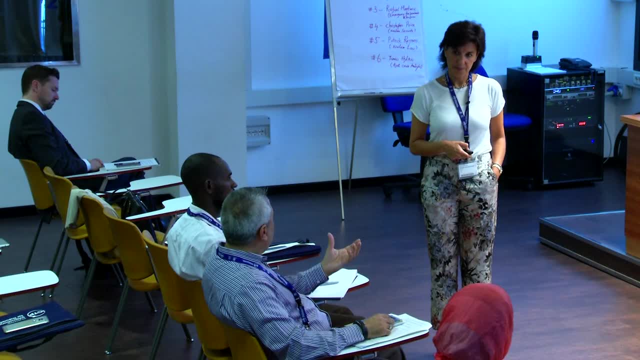 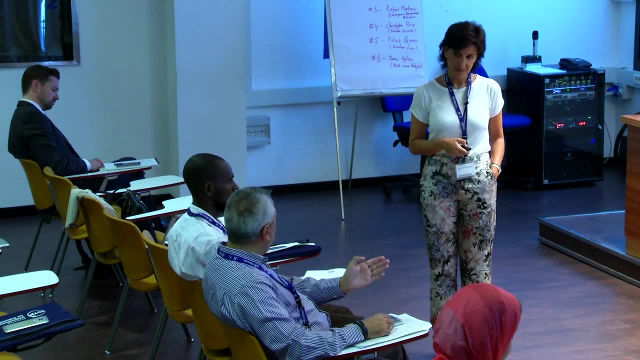 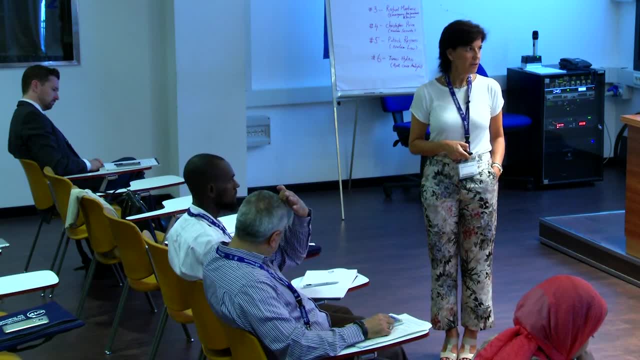 I'm not sure, I don't know, I'm not sure. And when you do that, When it's not enough, And then you have to. So the MOX fuel? As far as I know, The MOX fuel is produced with mixing. 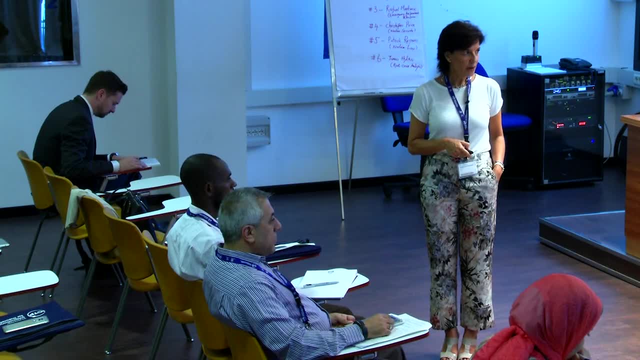 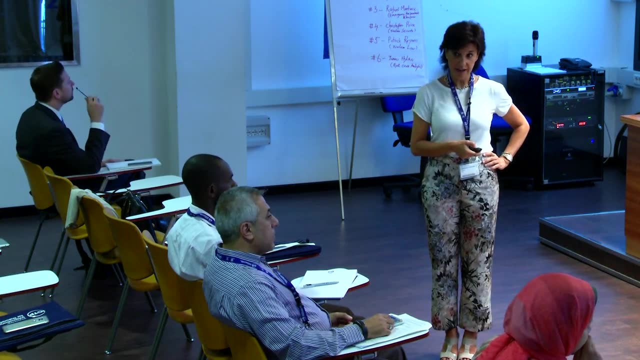 Plutonium And natural uranium Or depleted uranium. If you use repu, Repu has a different uranium composition Because it remains one per cent of uranium five In the repu And also there is other isotopes of uranium. 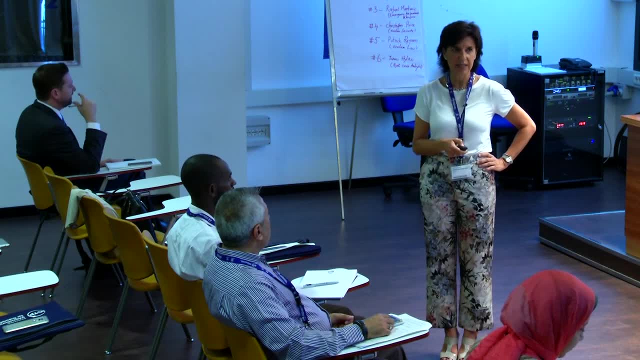 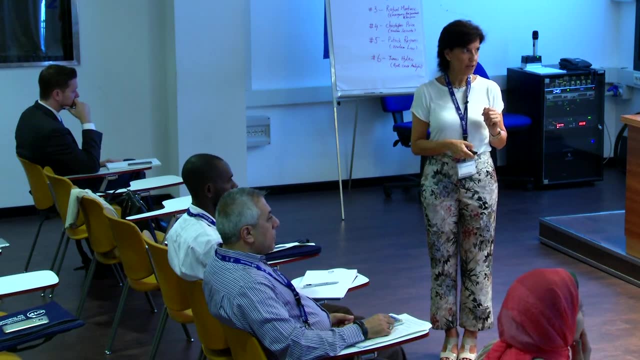 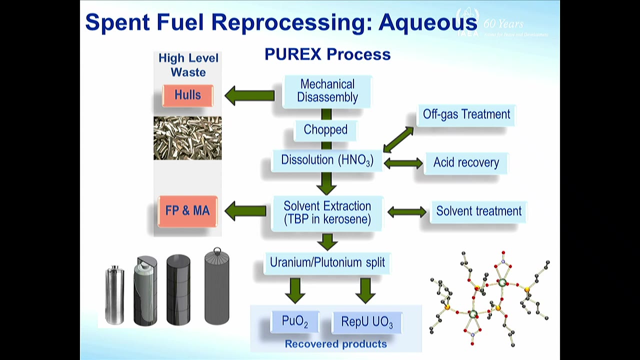 I think it's uranium two hundred thirty two. That is a very strong material. It's a very strong gamma emitter. So the isotopic composition of repul is different to the natural uranium or the depleted uranium. So I'm not engineering the core, but you have to have into consideration that the isotopic 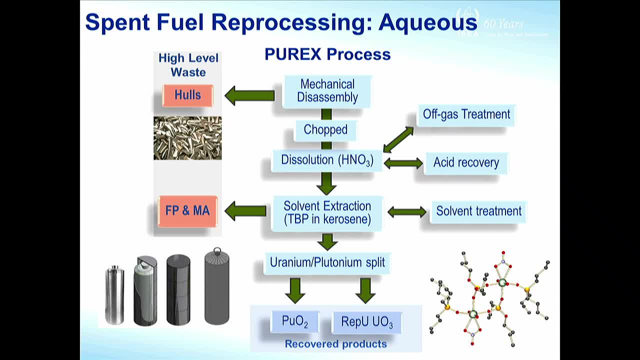 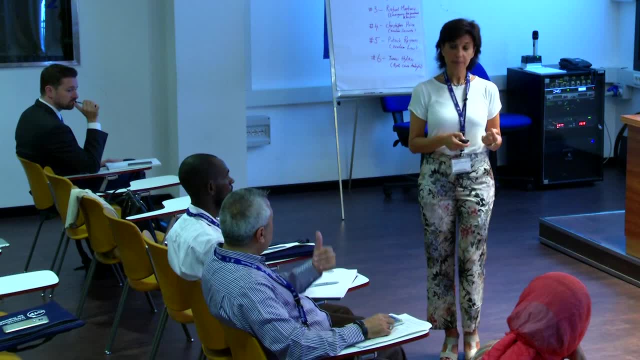 composition of repul is different. So what I will receive, I don't know. I think I will To reprocess: Yes, What I will receive. So it depends on the contract because, for example, some countries, when you sign the 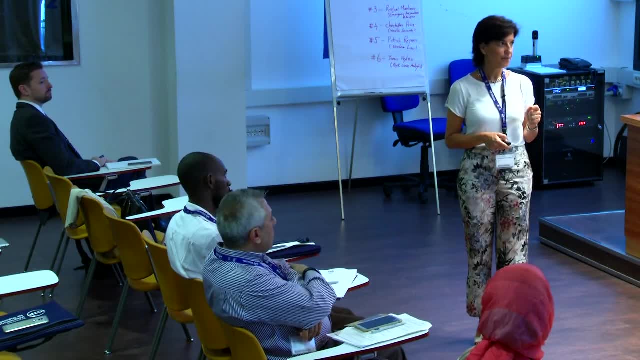 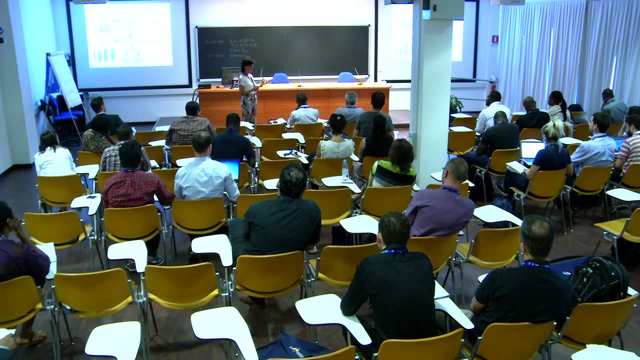 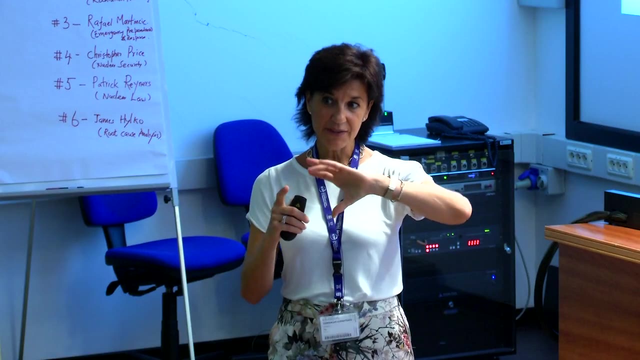 contract with a reprocess facility, you can receive MOX fuel. You can receive only the high-level waste. So you have to receive the high-level waste, because any country can get waste from other countries. So even if you send your spent fuel to reprocess, you will receive the high-level waste. 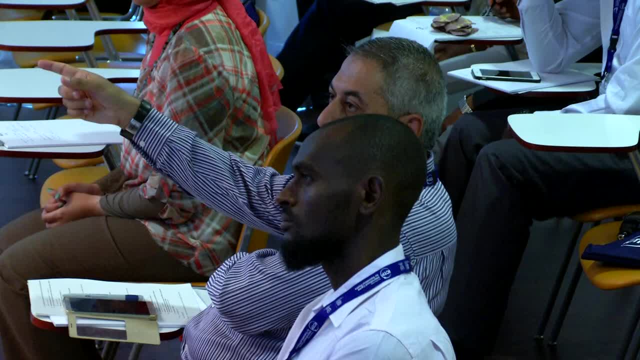 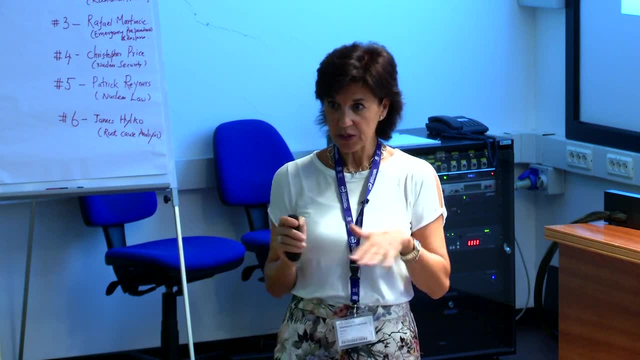 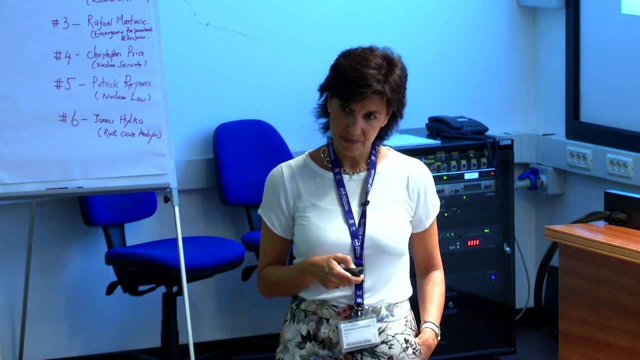 I will never receive the true fuel. I think you will. It depends on the contract, But you cannot. If you don't want to receive the repul, you don't need to receive the repul, I mean, which I will use as a fuel to receive the high-level waste from other countries. 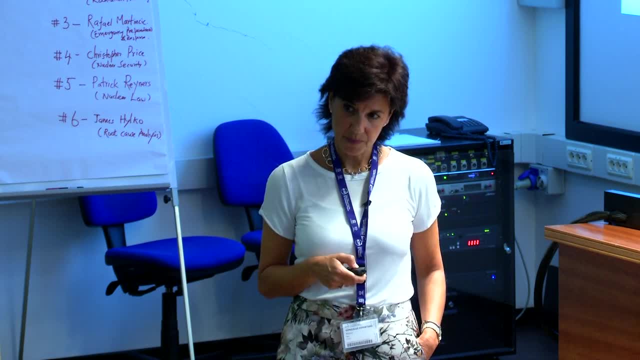 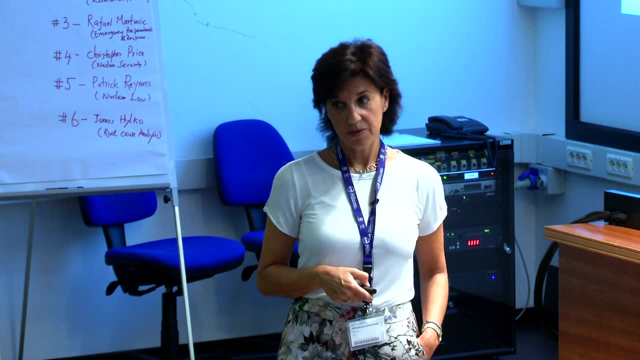 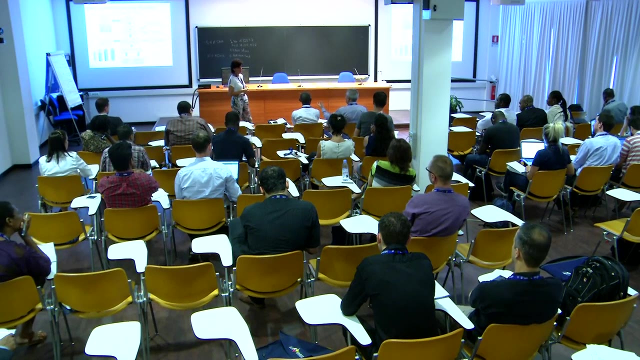 I mean as a fuel, Which is the fuel? I receive The fuel or the other one As a fuel. As a fuel, you will receive MOX. You will receive MOX fuel Because I understand You will never receive repul. 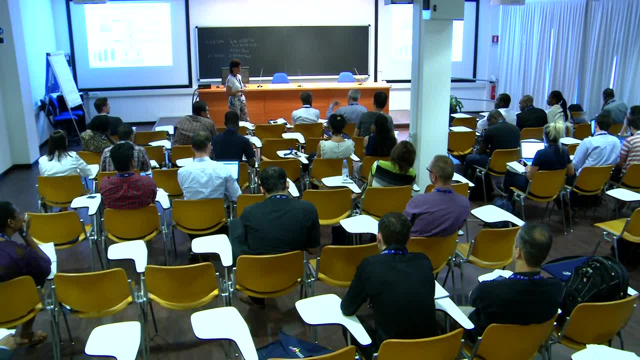 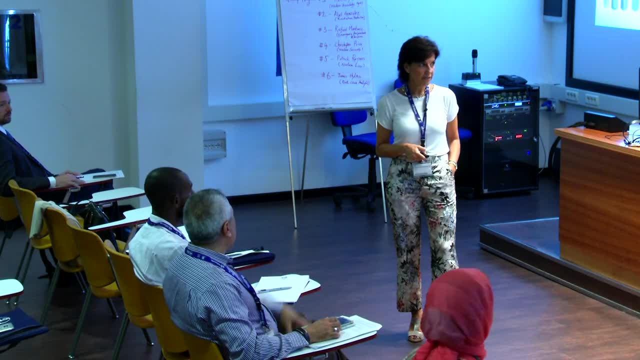 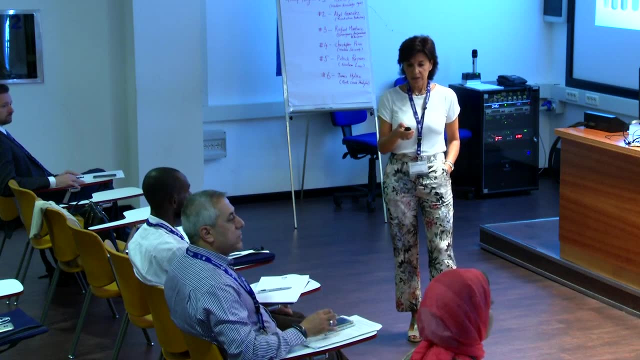 No MOX fuel. You will receive MOX fuel, which is your own fuel. Okay, so you will receive. Because the core is not designed for MOX, you need to modify it. Okay, So it depends on the contract you sign. 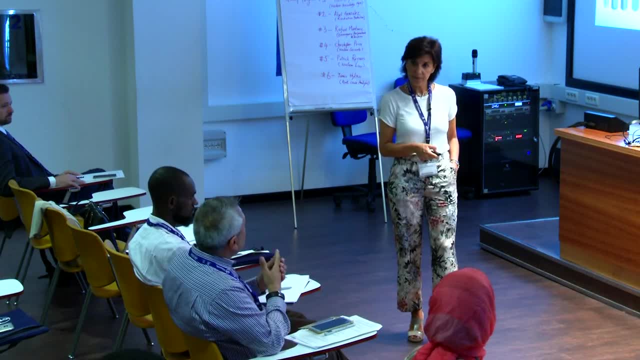 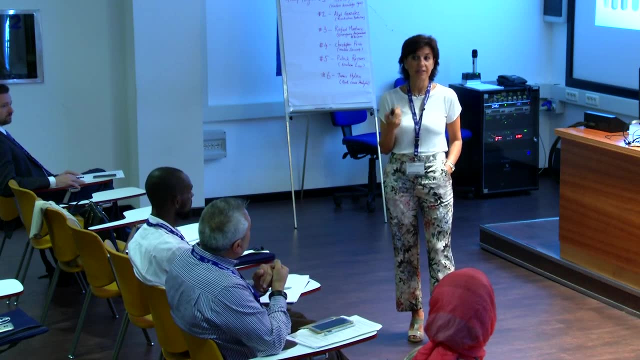 If your core allows you to use repul, you can. You can receive repul if your core allows you. For example, in the case of Spain, we send some of our spent fuel from Bandejos, for example, to France for reprocessing. 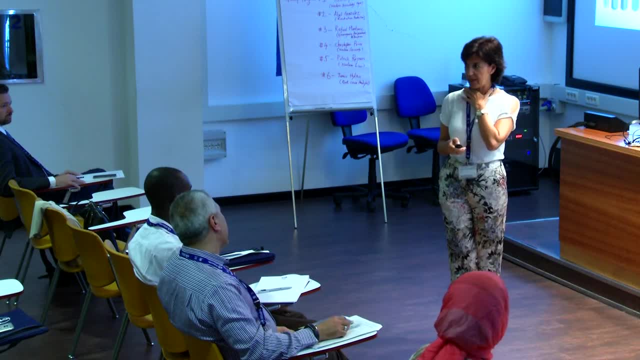 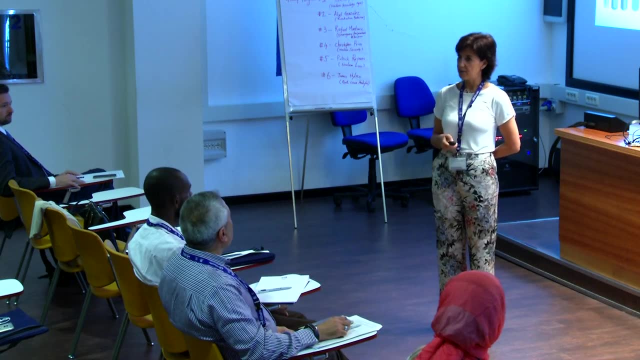 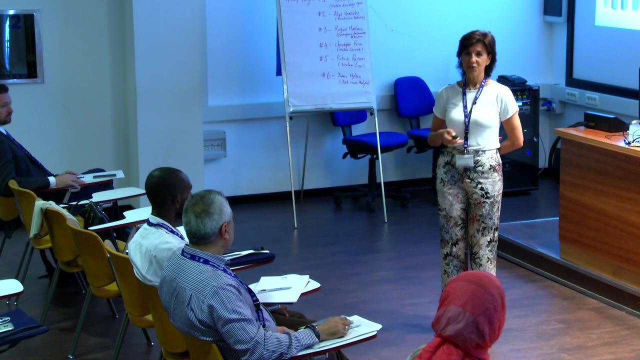 And we are not allowed to use MOX in our reactors And we are not allowed to use repul as well, So that we are going to receive is a high-level waste, But we don't have so far any storage to store high-level 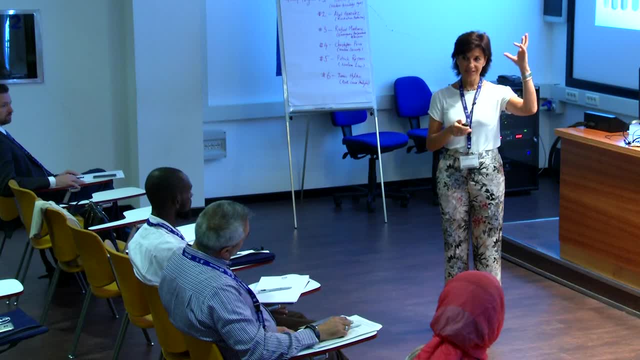 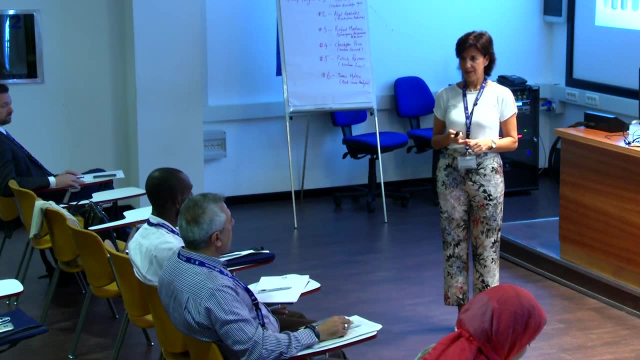 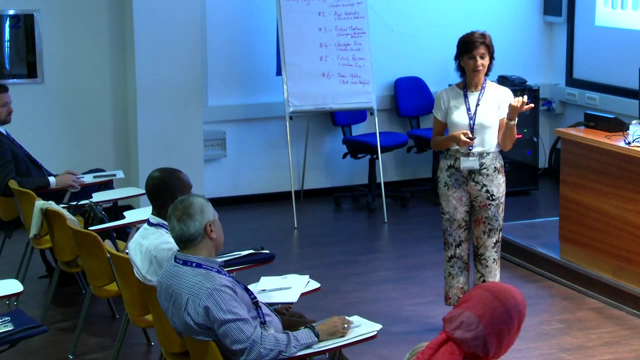 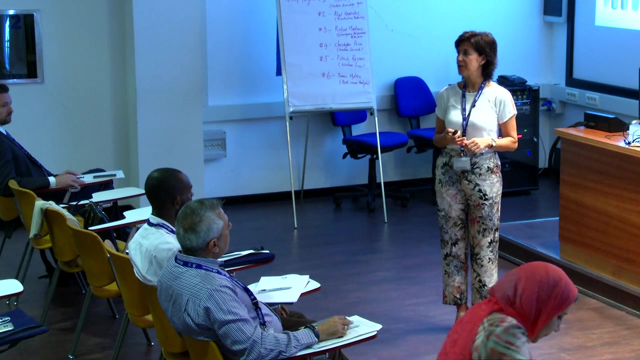 In Spain. So our waste remain in France waiting for our country to have a suitable storage facility. But we only will receive the waste because we are obliged to receive it. But we are not going to receive any additional fuel because we are not allowed in our nuclear power plants are not licensed to use MOX fuel. 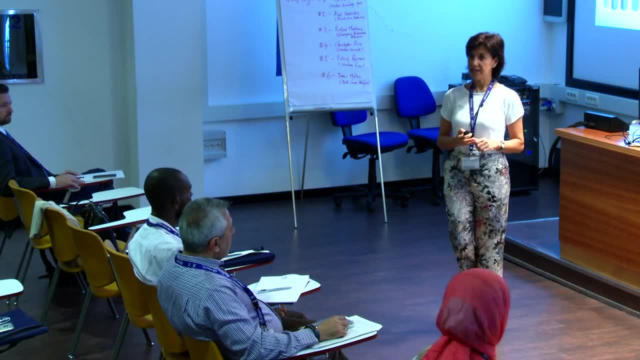 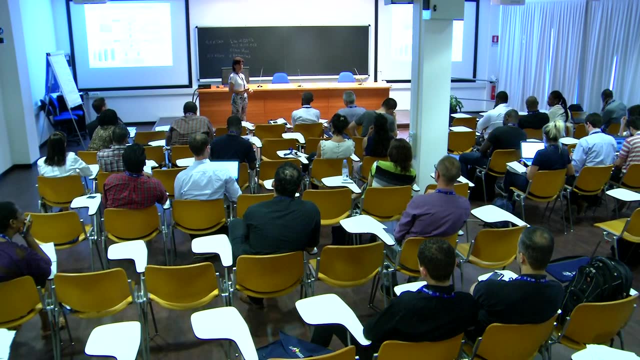 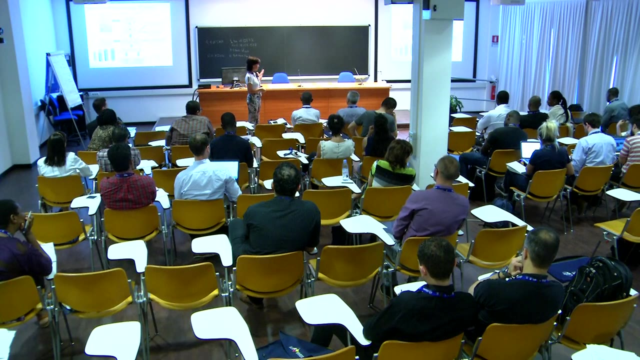 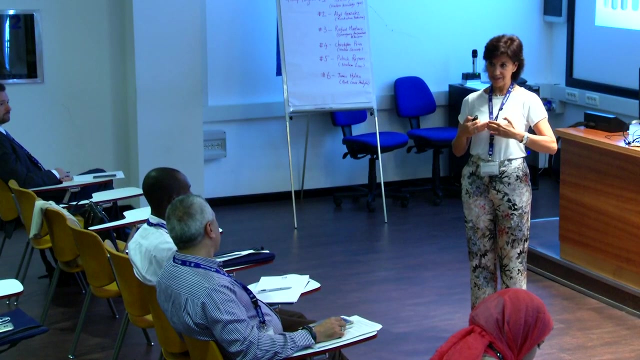 I love you. And this is contracted. This is not created in Spain, So it depends on the conditions of your license or your regulatory body and also your reactor, Because if you cannot use plutonium, you cannot use repul. the facility, the reprocess facility, can use it and can sell this material to another country. 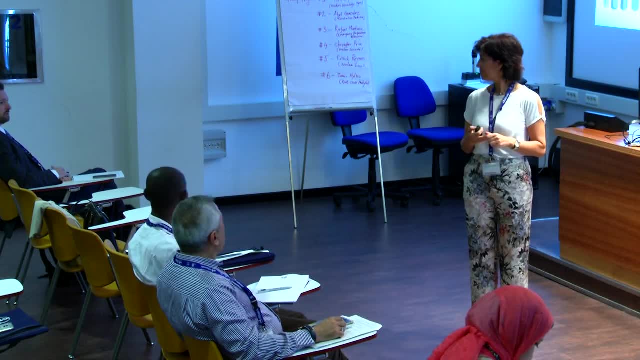 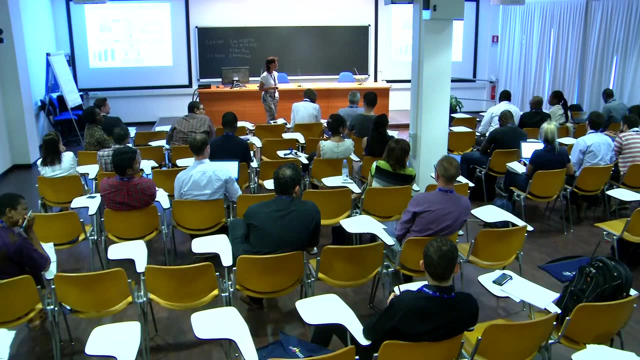 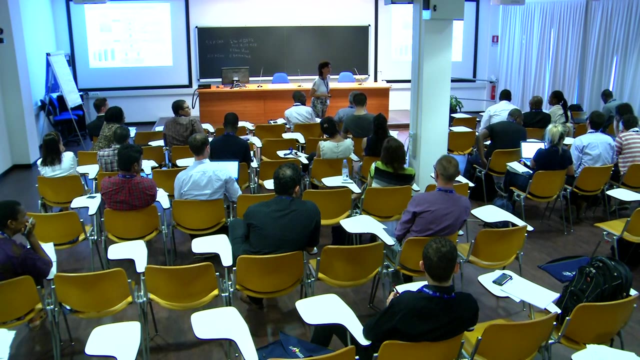 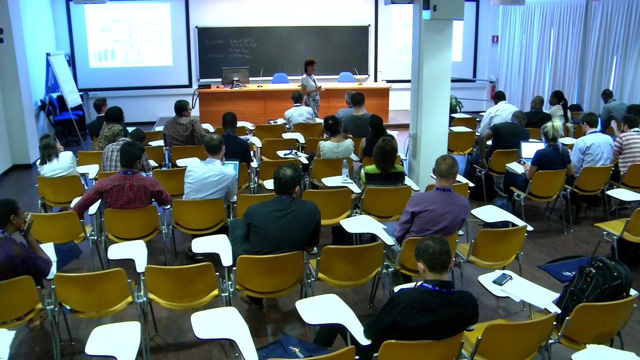 So it can be used for another country. Are you seeing this? Oh, it can be used as a fuel, but the core should be changed a little bit and the design of the core should change. And the problem with REPU is the composition of uranium after reprocessing the isotopic. composition change and now it needs additional safety requirements because there is one of the isotopes of uranium- is 232, and it's a very strong gamma emitter and you need a shield for the workers or to remote handling. But it can be used very rich again and can be used as a fuel. 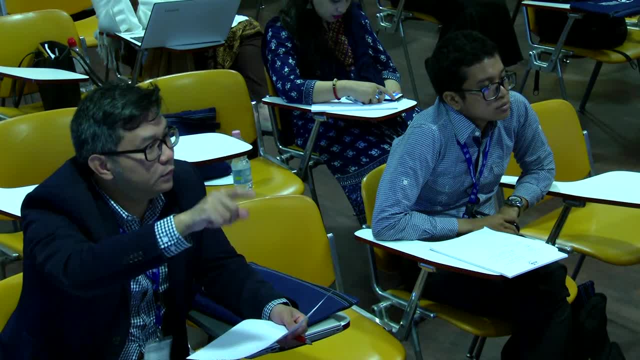 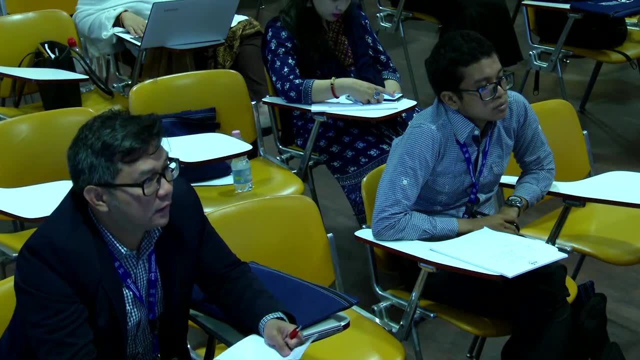 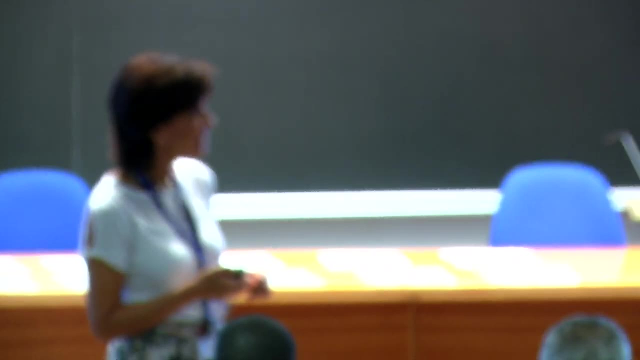 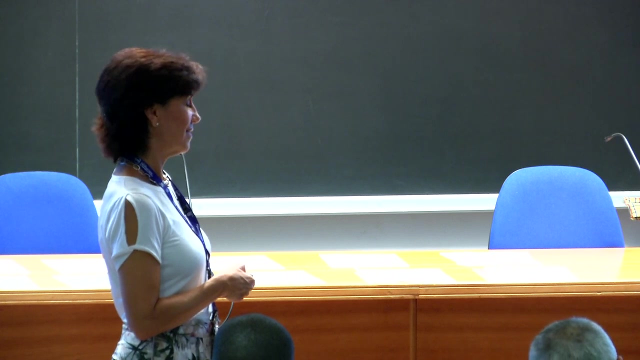 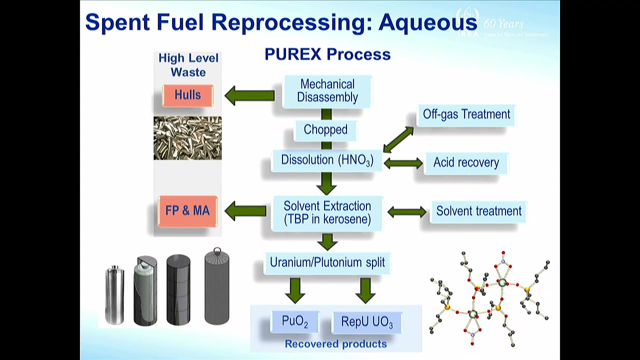 Of plutonium and REPU. Yes, Ah, because the REPU is the 95% of the spent fuel, is? Yeah, so if you consider, for example, one road and the final composition of the spent fuel is around 92% of uranium and around 1% of plutonium. and this is if we consider. 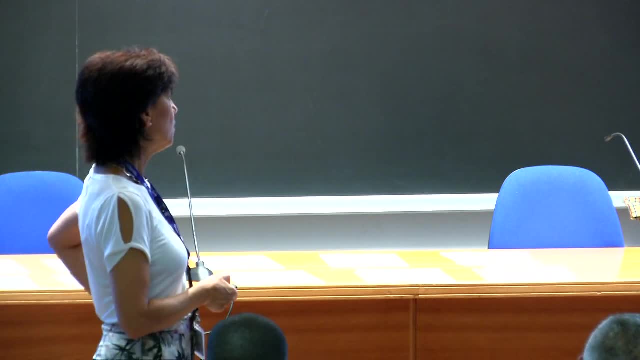 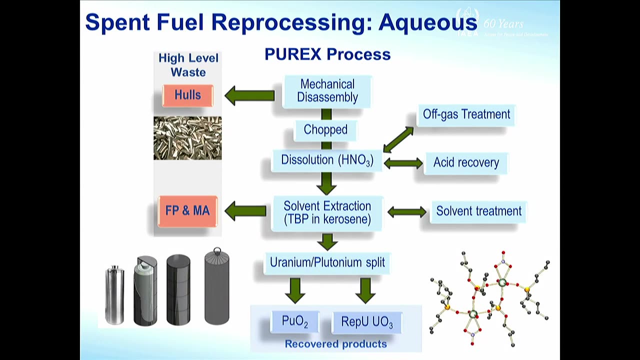 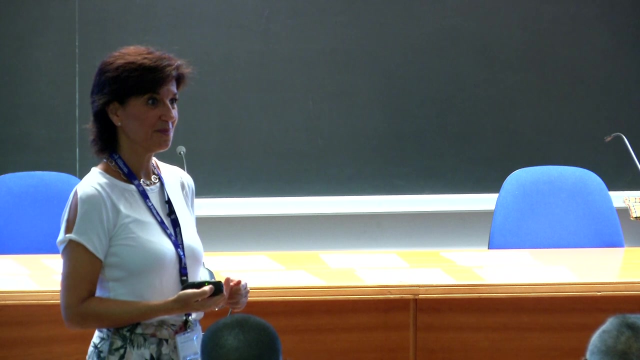 that the process is 100% efficient we will get at the end. the plutonium is 1% in the beginning and REPU it's 92%. it's 92% because the bulk of the spent fuel is uranium. That changed the composition. At the beginning the composition was 95% uranium-8 and 5% of uranium-5. But at the end in the core, the composition changed from 95% of uranium-8 is now 92,. because some of the uranium-8 has been consumed, producing plutonium-9, and uranium-5 has been fissioned And it's consumed from 5% from the beginning to around 1% at the end And during the fission process and the neutron capture process. there are also changes in the composition of uranium and there are new isotopes produced. But if we consider that we started with a population that was 50% of uranium-8,, at the end we will have 1% of plutonium and 92% of repul. 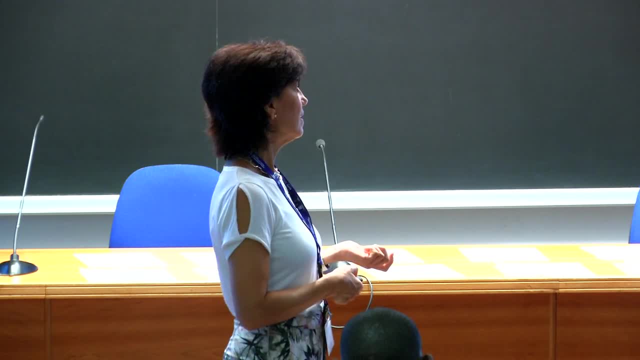 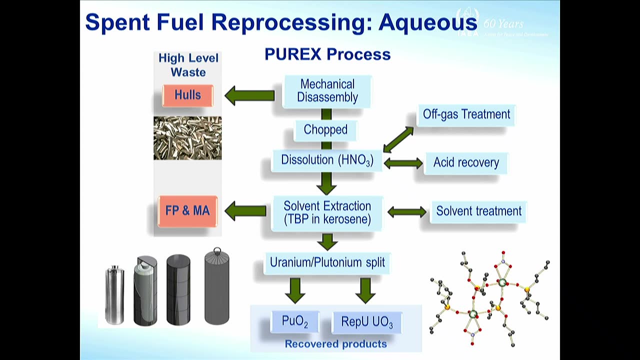 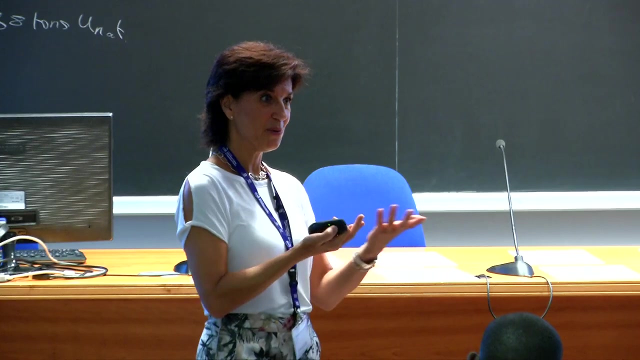 So, since in the enrichment process there is a lot of depleted uranium produced, it's easier to use the depleted uranium or natural uranium to fabricate MOX fuel, because you can handle this uranium without any shielding for the workers. But if you use repul, you need a facility, a modified facility, because the isotopic composition of uranium has changed And there are strong gamma emitters now I think uranium-2,3,2,. it's still noble, But if uranium-2,3,2 exports to neutrons, 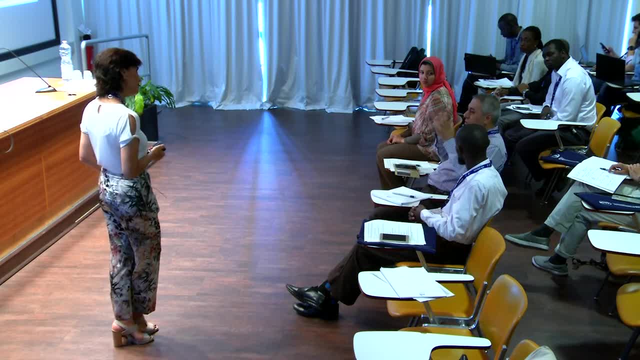 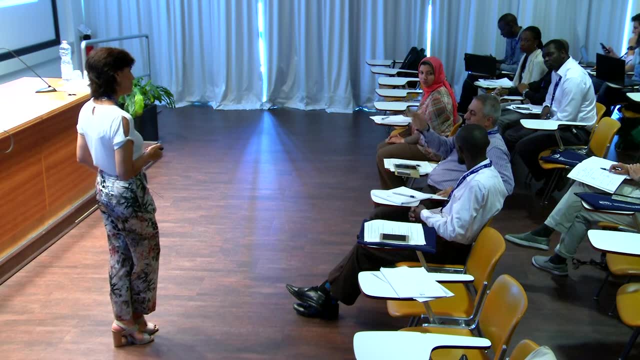 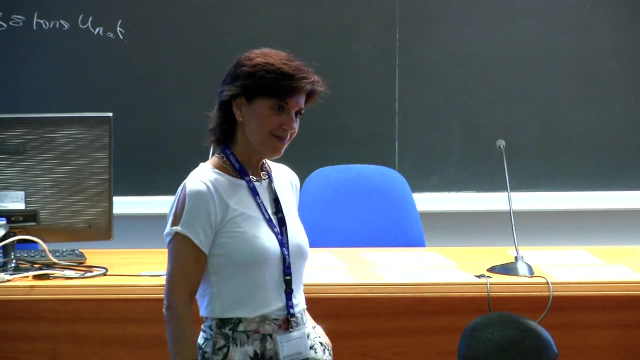 I think the altitude will be- I don't remember the name- But not uranium itself. This, this element, will give a high gamma rate, Gamma, high gamma emission. So even for just that, they we talked about the reparation of uranium-2,3,8,. 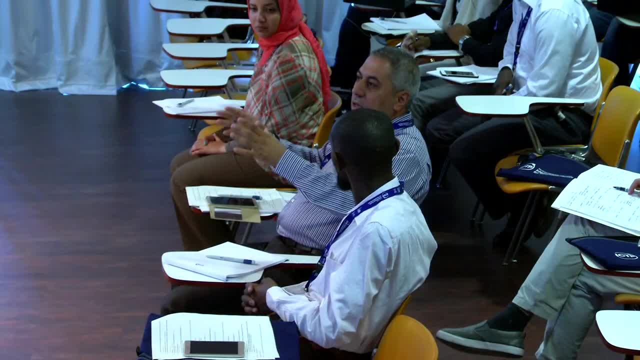 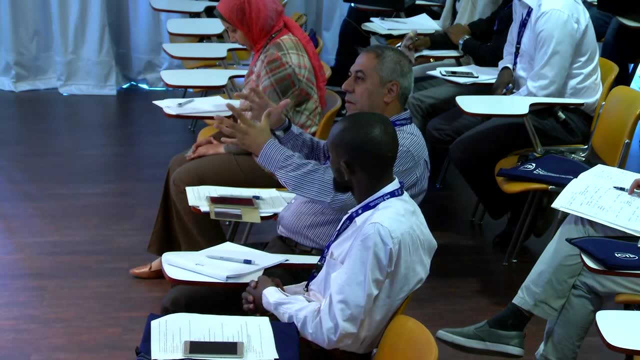 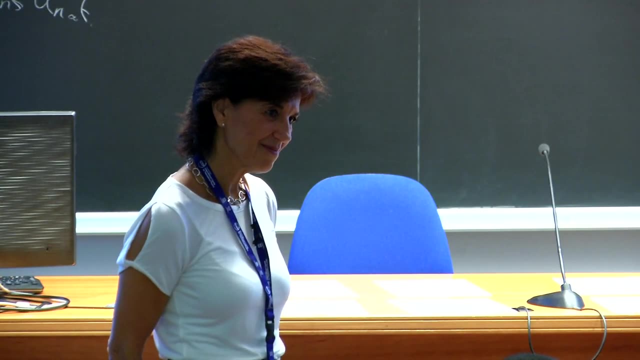 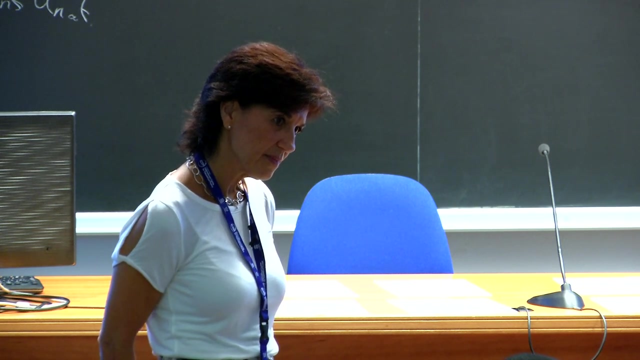 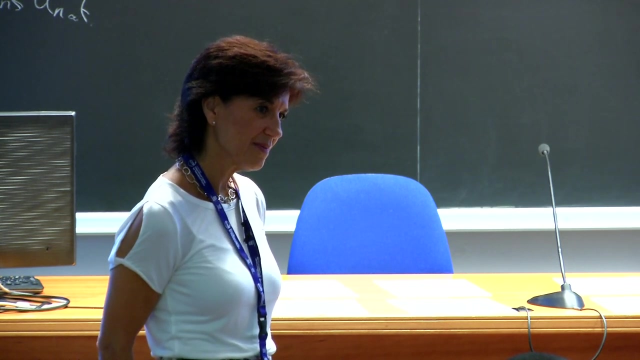 2,3,2.. By the way, a plutonium is from full cycle. You can. by the way, it's from full cycle, But if you have online refueling or you can remove 2, 3, 2- uranium, 2, 3,, 2, before it goes to the US. so it means online, you can. you have a problem with or challenge with that operation? okay? 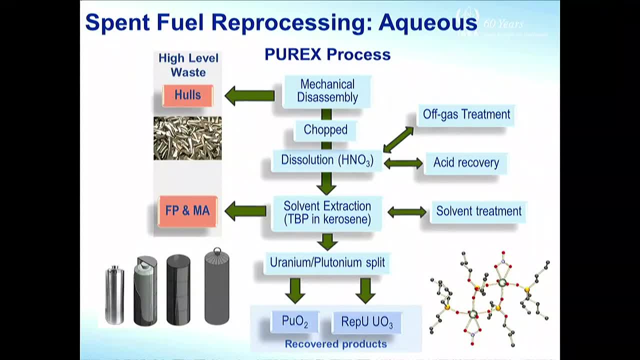 So uranium, as if it's normal for gamma, no problem. The problem with that it's for neutron, more neutron. in this case, you will have another element, maybe this one, I don't remember. Okay, Then you have the problem with again. 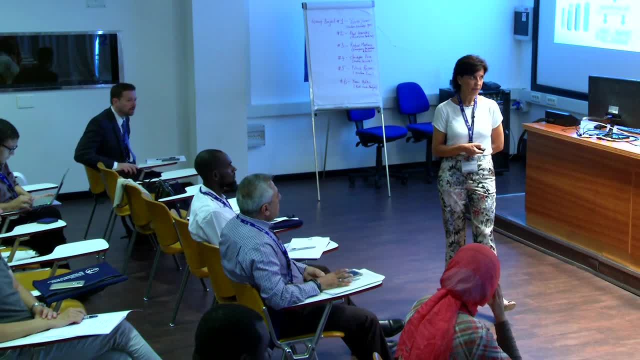 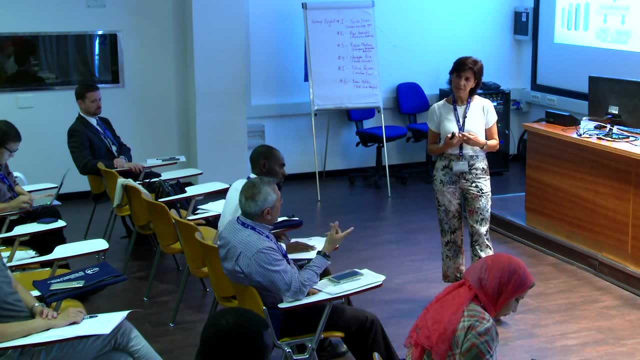 Ah, okay, But I mean it's not the same, because for the handling of this uranium, the facility Yes, As if no problem, You can have it, But the problem is you have to go to the US. 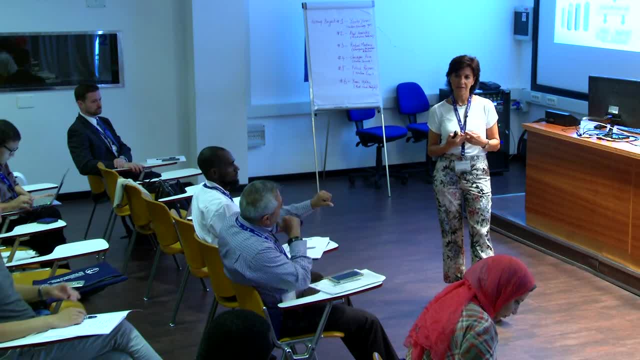 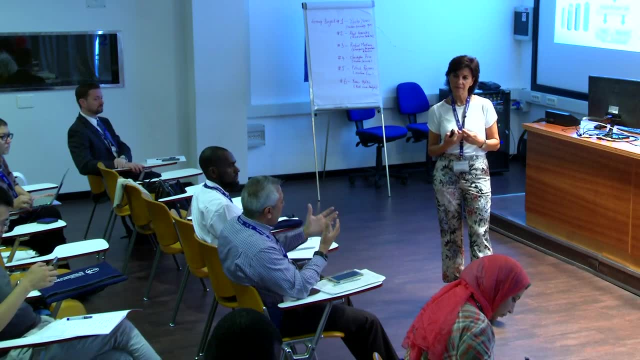 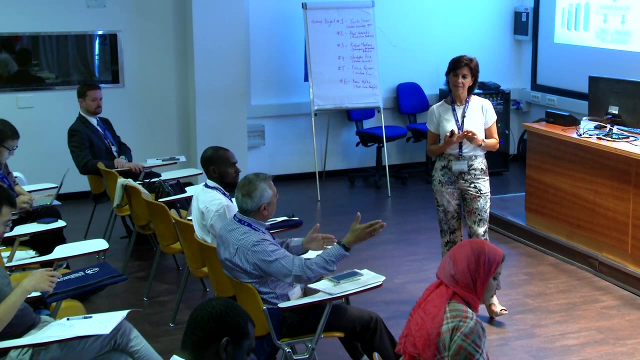 Ah, So in the spring to fuel for thorium, your cycle, you already have 2,, 3,, 2 in the core and a lot of our. they will report to US and in this case you will have that element which is, I think, plasma, and then you have the gamma. 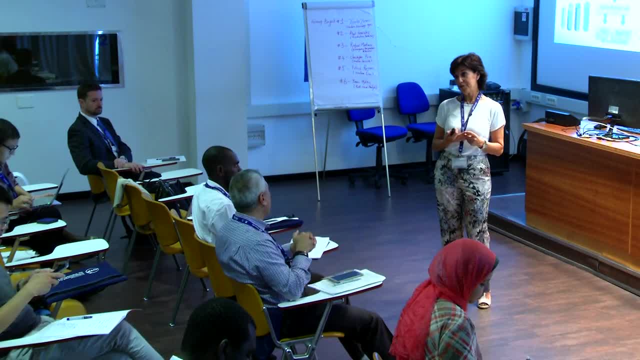 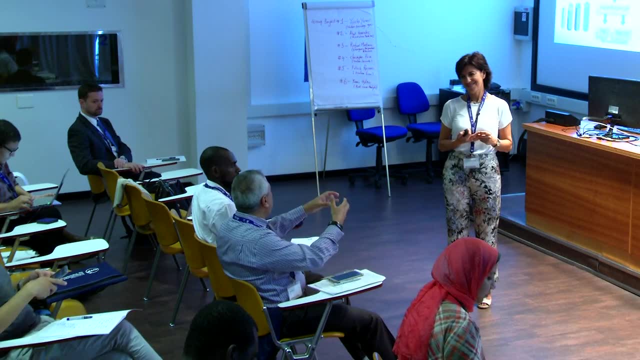 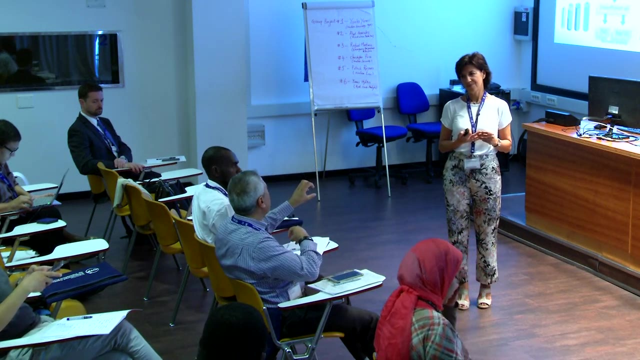 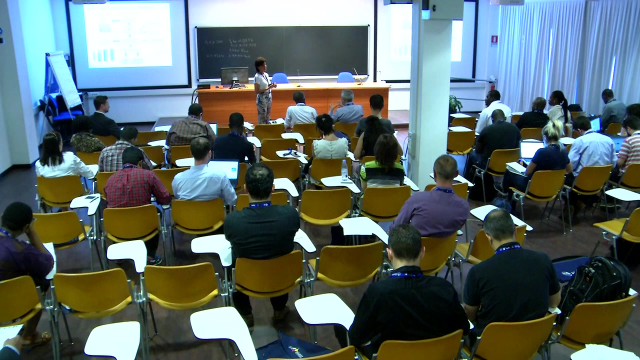 But the handling is very difficult. Mm-hmm, To do it from preparation? Yeah, from the preparation. you should, yeah, You can, one way to, to, to make something Uh-huh, Which is, by the way, have this, this help us. 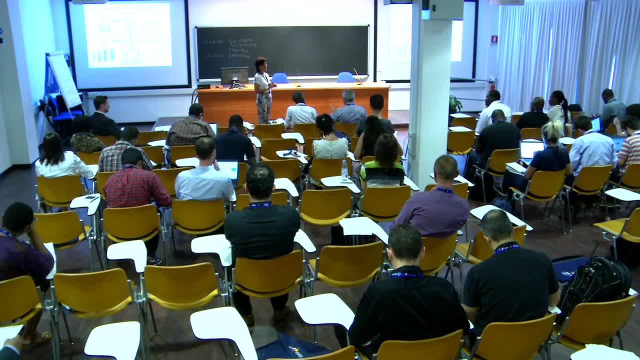 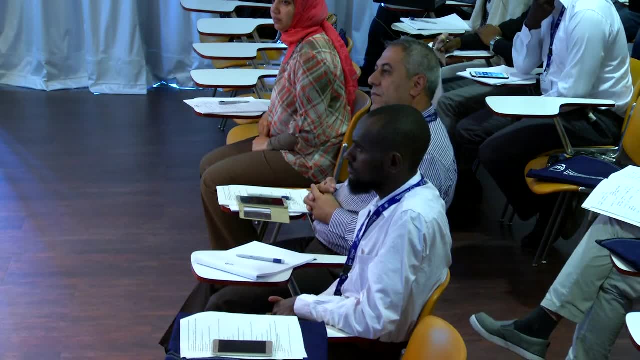 Ah, okay, Okay. So I will give you after the talk a reference, because there is a very interesting technical report dedicated to repul. Uh, it's a very interesting technical report. Uh, it's a very interesting technical report dedicated to repul. 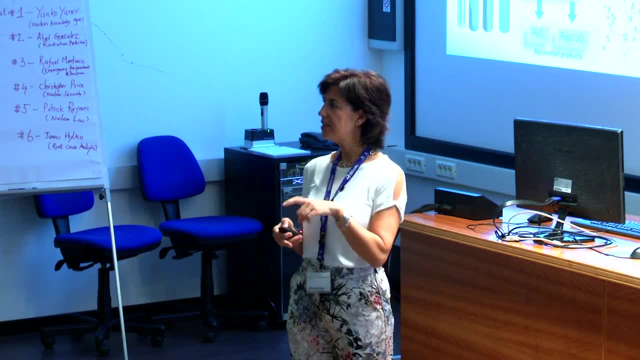 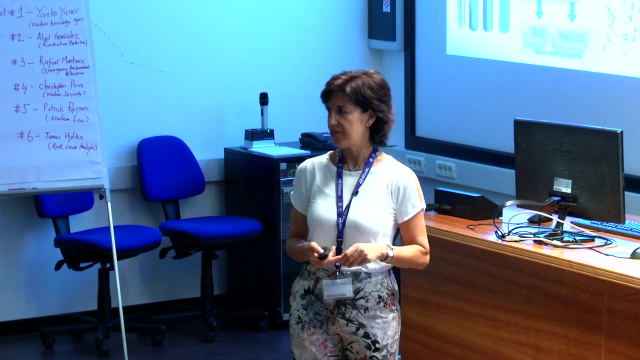 Uh, it's a nuclear energy series. So- and in this report there is a lot of- there are all options for to manage repul and to use repul so far. So I will give you the the reference after the talk. 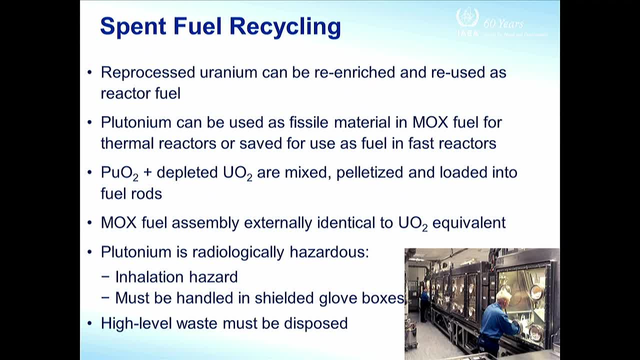 So the red processed uranium, as we talked, can be enriched again and reused in the reactor fuel, and plutonium is used to produce MOX fuel, Uh-huh. And the second fuel is mixed oxide fuel. So to produce MOX fuel, plutonium and depleted uranium are mixed and pelletized and loaded in the rods to fabricate new fuels. 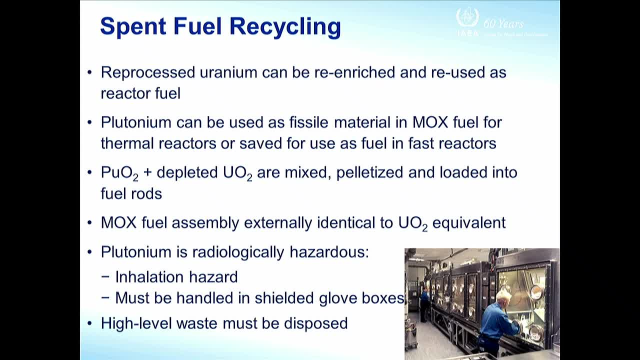 And for example, in France, most of the of the of their reactors are licensed to use MOX fuel And certainly the fuel and the fuel assembly are identical to The oxide uranium fuel. But in this case for the fuel fabrication it's necessary to make it under glove box due to the plutonium is uh has uh problems with inhalation as hard as because of it's a very strong alpha emitter. 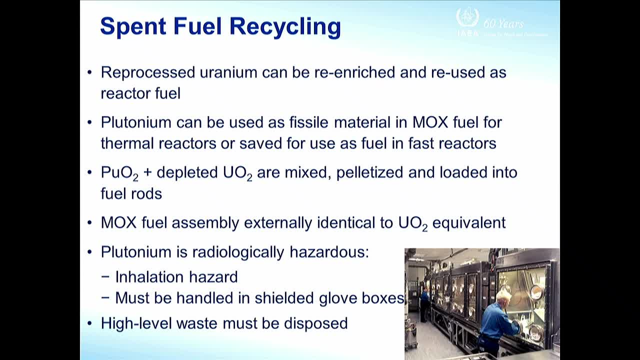 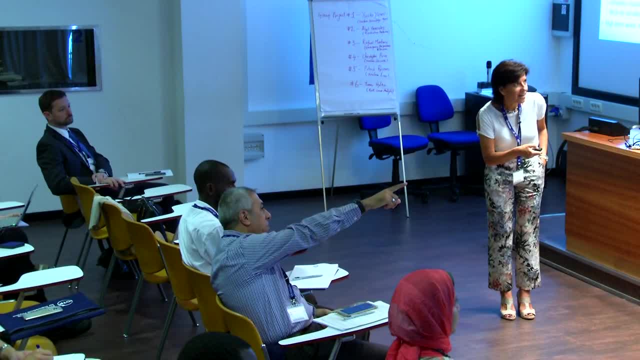 So it should be handled in glove boxes? Yes, sure, Uh-huh. So I took a report. There's two different things: Epoch uranium, Our fuel, which you can reuse as a reactor fuel, Uh-huh. 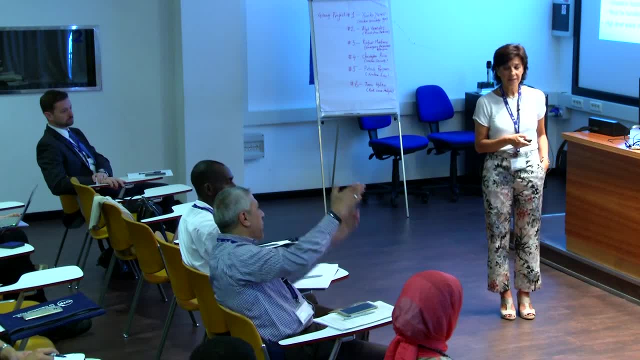 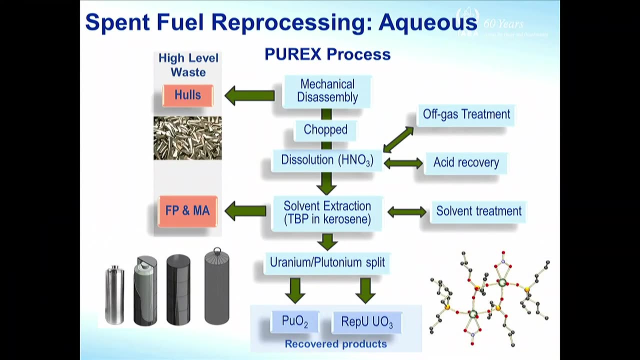 And then you have the MOX fuel, which is not plutonium, Yeah, So if you have the two, you have, I think, the MOX fuel and the other one, the reprocessed fuel from the radio fuel. 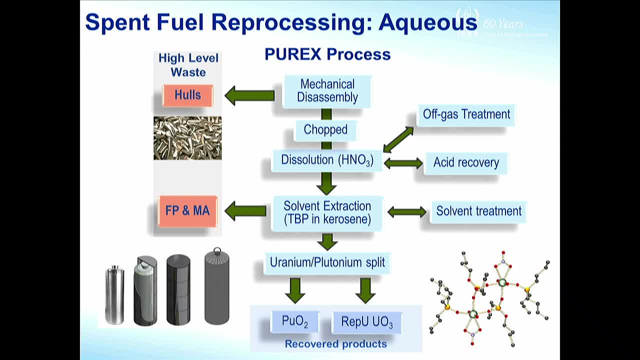 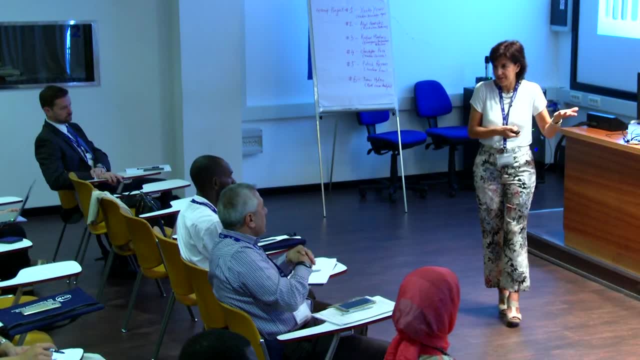 Yeah, because in this case, if you are very rich again- because the enrichment is around 100%- if you are very rich, you have to use the plutonium. So if you are very rich again, you don't need any other fissionable. you have the uranium as a fission: uranium-fired. 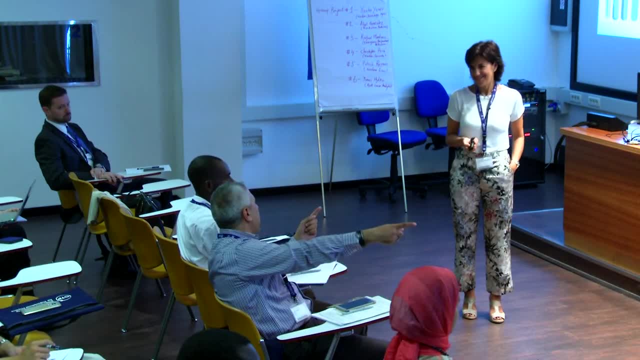 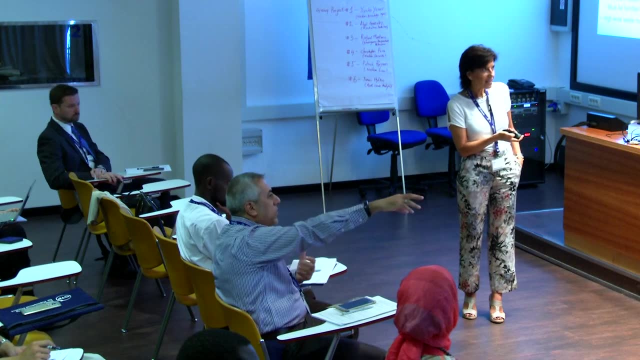 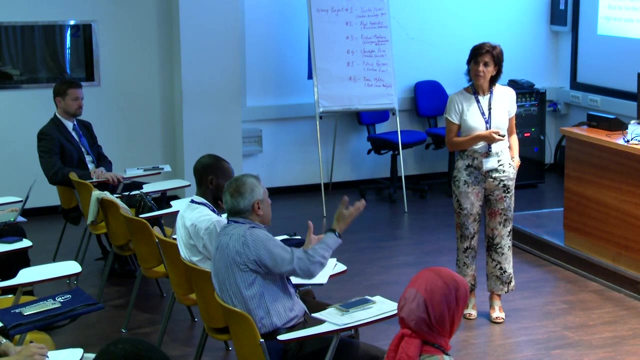 You have already, but you need to be rich. Yes, you are rich, And this is what happens. by the way, I don't know, according to the fact, even what we receive. we will receive the reprocessed uranium and the design of the core is really, from the beginning, for reprocessed uranium, but it's not really for MOX. 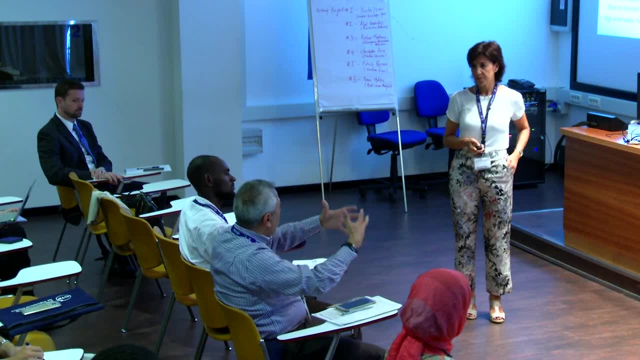 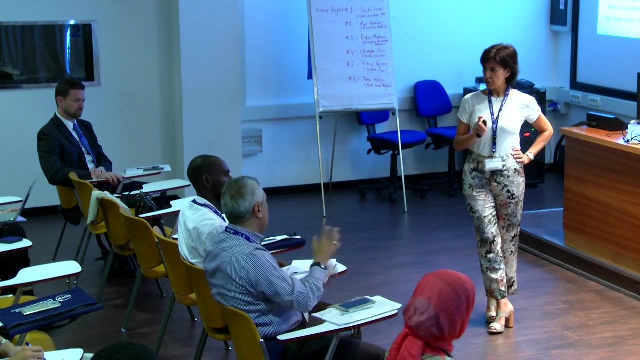 MOX? Ah, okay. So if you have, if you have, if you receive the reprocessed uranium, not the MOX, So you will never receive the plutonium because you are not? okay, yeah, but it depends on your contract. 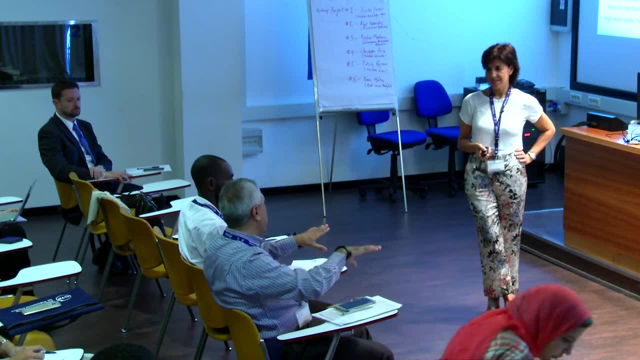 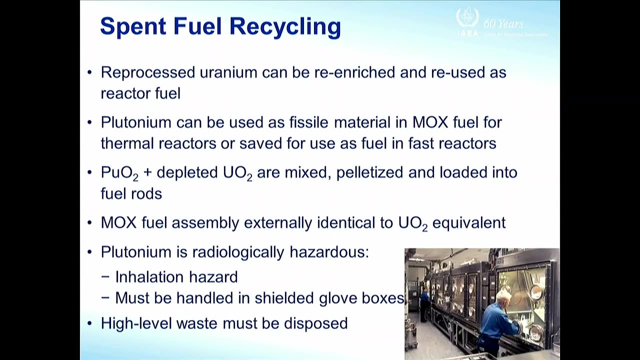 In the case- Yes, I mean, yes, I mean, that's a- you need to modify your core. Yeah, So you can. yeah, if you. even you need a license to use reprocessed uranium, For example. in our case we don't, we cannot use it in Spain, but if you are allowed to use, you will receive the reprocessed uranium re-enriched or you can re-enrich and reuse again. and the plutonium, as I mentioned before, is mixed with depleted uranium, because the fission material is plutonium and the depleted uranium act as a matrix and as a protein material. 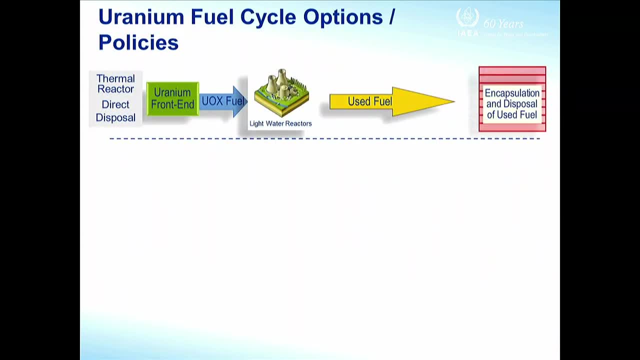 Yeah, So as a summary, We have talked about the open cycle. One of the fuel cycle options is the open cycle, so it's considered they use fuel as a waste. The one-through cycle or the closed cycle is not fully closed, because plutonium is used once as a MOX fuel and then is stored or is considered waste. 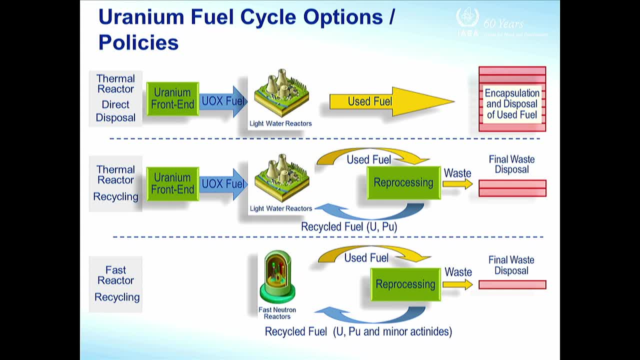 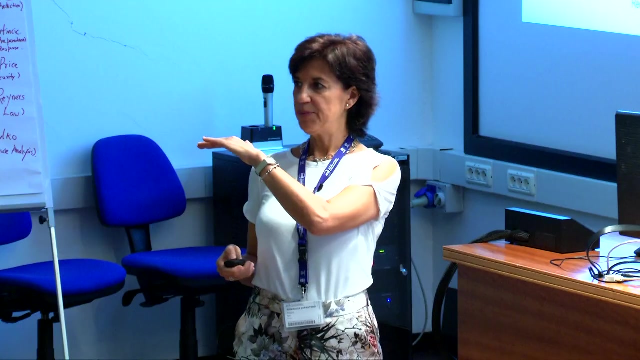 And now for the future and for the sustainable Sustainability of the nuclear energy. There is a lot of effort applied to use and to develop as a commercial scale fast neutron reactors to fully close the cycle and to reuse all the time plutonium and to get the equilibrium in the plutonium. 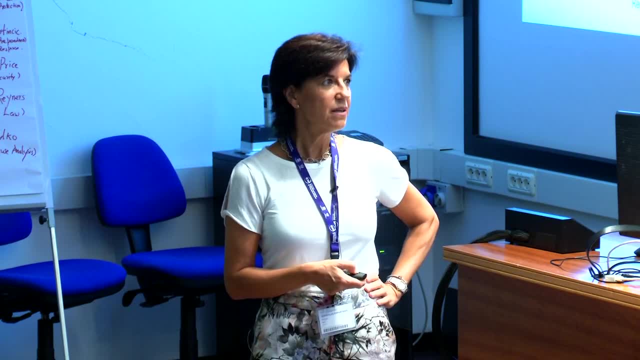 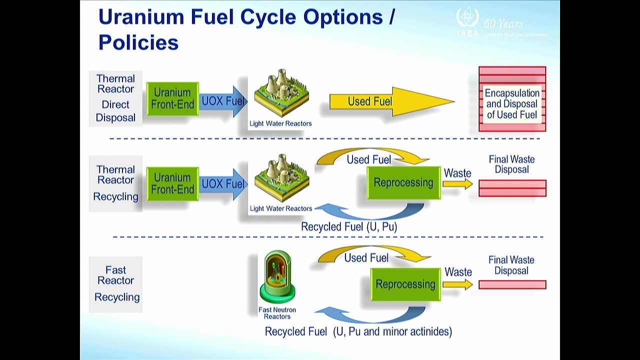 So in the ideal world it will. it won't be necessary to have more uranium And with plutonium we can sustainable and we have the stable inventory of plutonium. So it's reduced in a huge amount the waste produced and the burden of the waste. 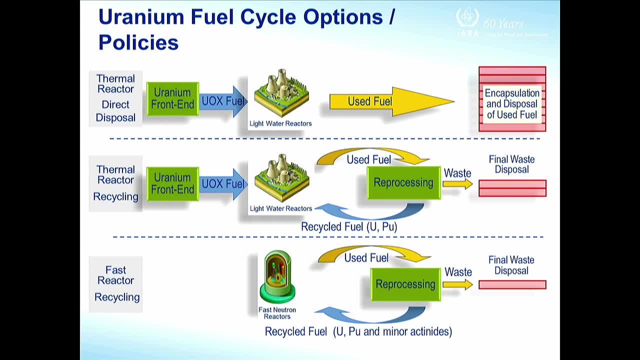 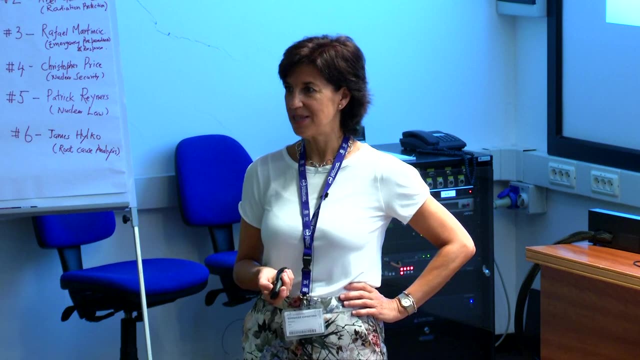 So this is the A&D so far- is dedicated to have this fuel cycle option, And there are countries, as Russia, that has the only operating fast reactor In the world. it's the BN-800, and it was connected to the grid in 2016, 15.. 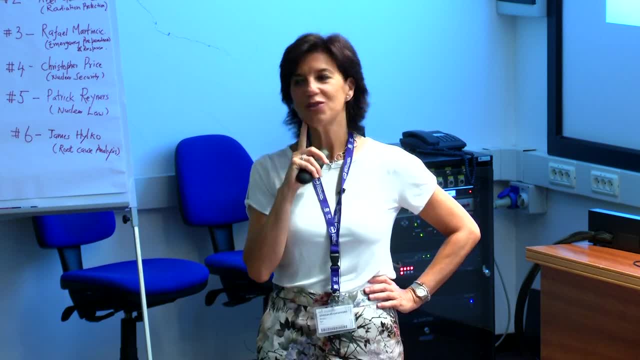 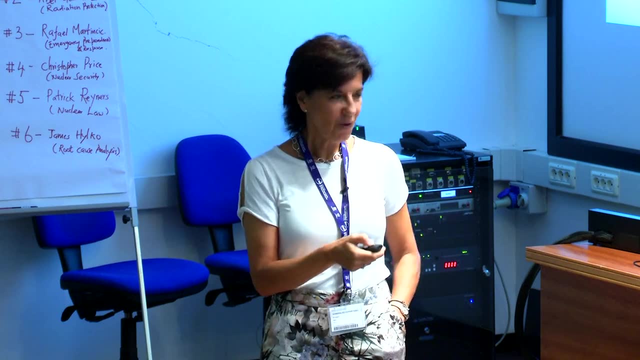 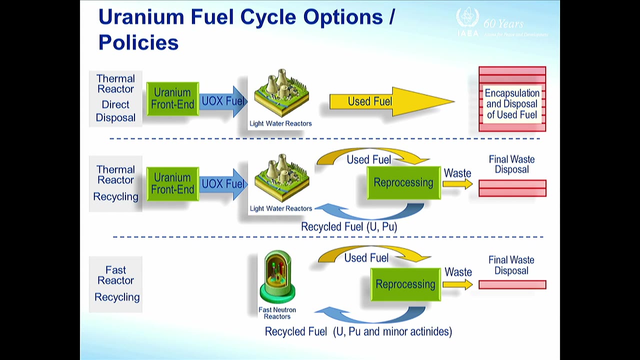 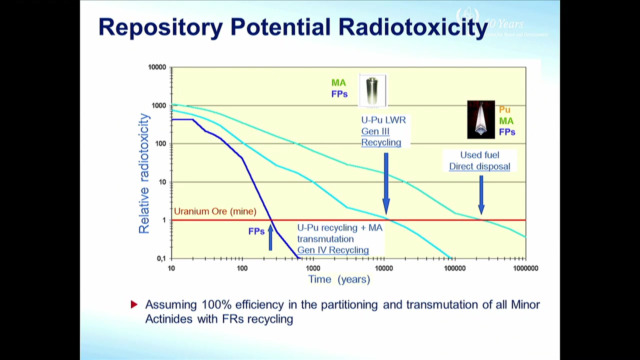 And we had last June the fast reactor conference there in Yekaterinburg with 800 attendees and with all the community of fast reactor and associated fuel cycles. So this slide, it means it represents the radiotoxicity and so we can see this is a radiotoxicity evolution of the open cycle. 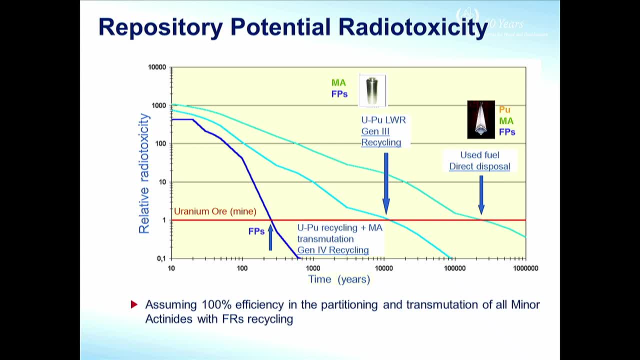 And it's due to plutonium, mainly to plutonium. If we avoid plutonium in the high level waste, the radiotoxicity decrease and it's due to minor actinides. But in the case of plutonium, the radiotoxicity is in the same and it's due to radioactinides. 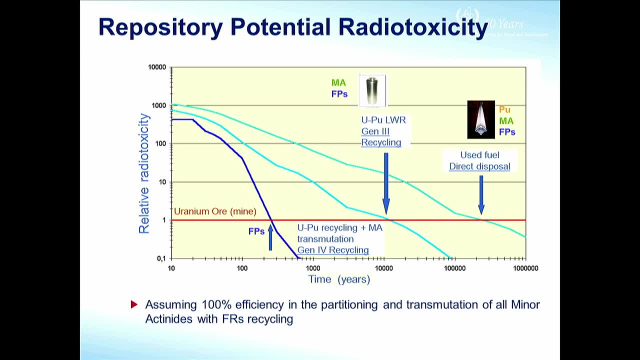 All right of fully use the fast reactors and the advanced fuel cycles and the fully use of uranium-plutonium recycling plus the minor actinide recycling. Only fission products remain in the high-level waste and due to the half-lives of the radionuclides. 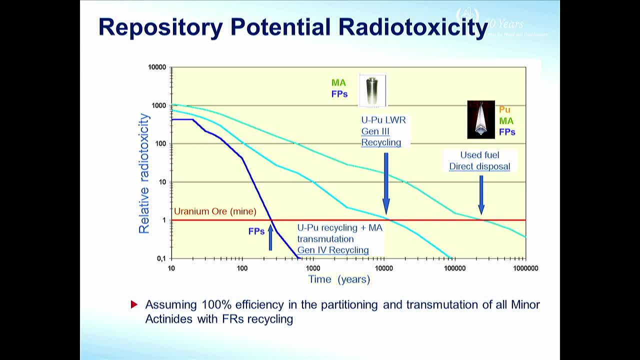 of the fission products. the radiotoxicity gets the radiotoxicity of the uranium in around 100 years, So 300, 400 years. So compared to millions of years, is an increase in the reduction, an improvement in the reduction of the burden of the radiotoxicity. 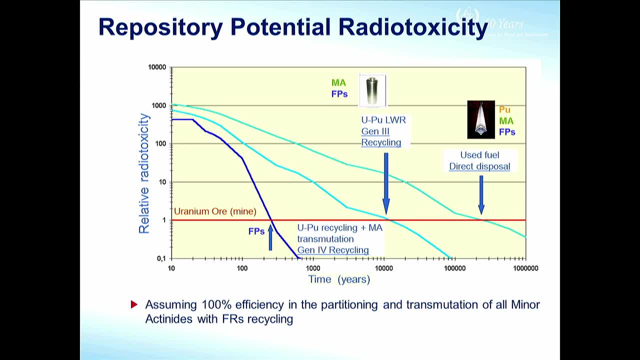 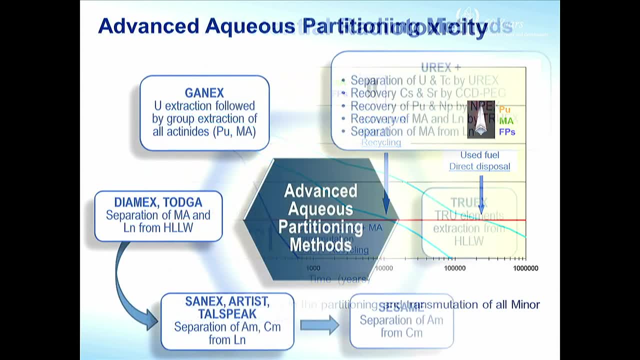 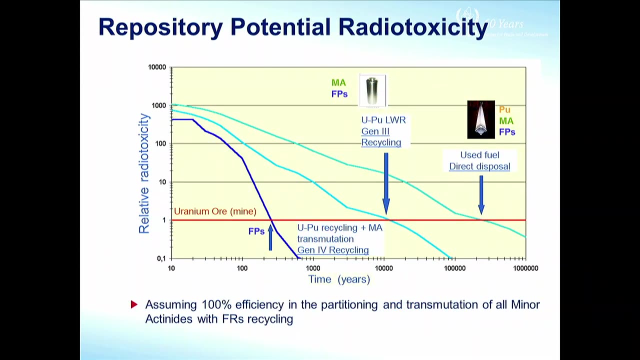 in the high-level waste, And this is the future. that is the future that is foreseen in nuclear energy technology. So let me give you some examples of the So to apply these scenarios, we need to have So uranium-plutonium recycling. 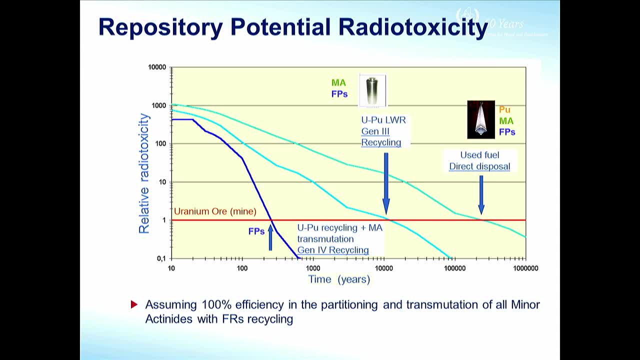 from the chemistry point of view has been already proved with PUREX process. but to get minor actinides is not that easy task because the minor actinides and some of the fission products have the same chemistry, So they are trivalent elements. 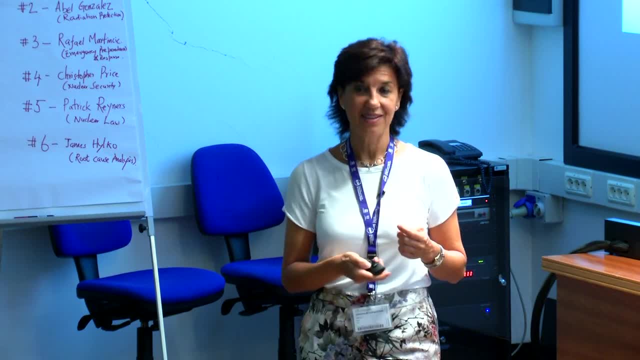 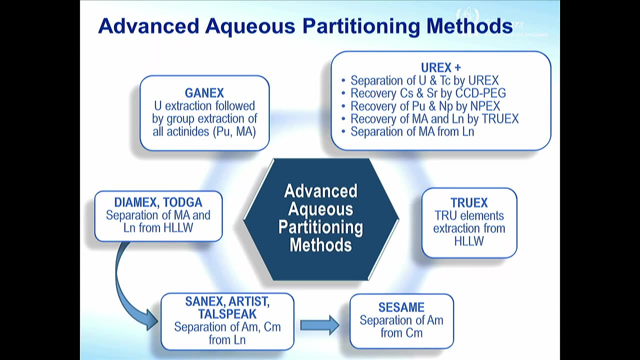 and it's not that easy to separate them. So there are international efforts applied to this and there are some European projects and also American projects And we try now in the INC to coordinate all these R&D efforts in the world. So we try to set a project. 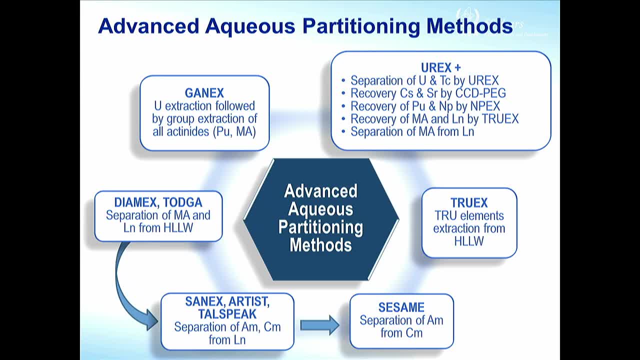 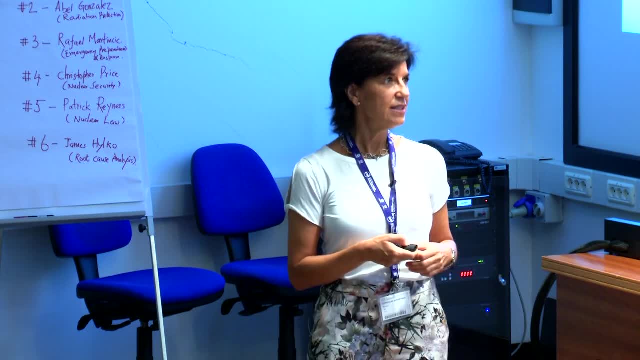 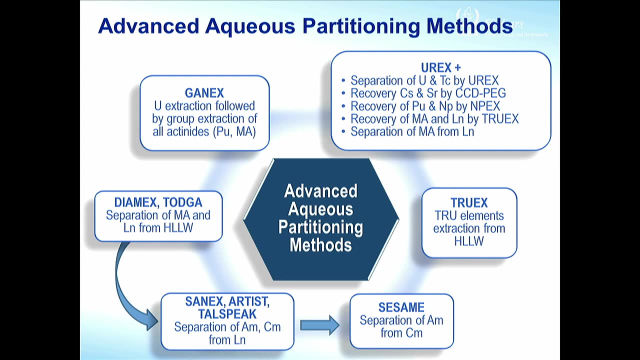 with the European community, with America, Japan, Korea, China. We are working on that. So, for example, this is the American process, it's Eurex Plus and it's a modification of the PUREX process, And the P disappeared from PUREX. 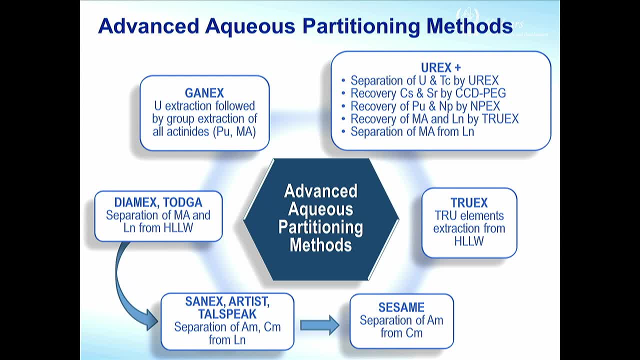 and now it's Eurex, because they work not to have plutonium separated for the proliferation issues. So they separate uranium, they separate plutonium with the rest of minor actinides, basically with neptunium, and they conduct the process in steps. 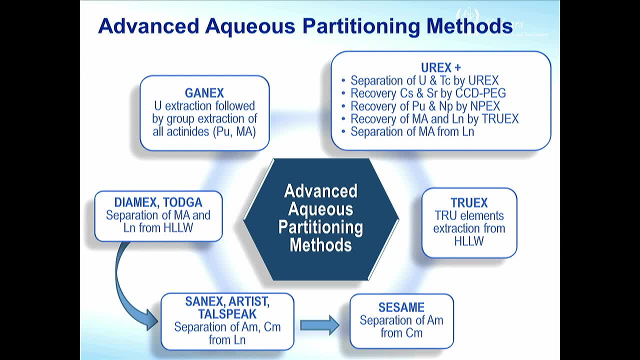 So they separate uranium and also they separate those elements that produce heat decay, like cesium and strontium, and they separate plutonium with neptunium, The minor actinides with the lactanides that are the main fission products. 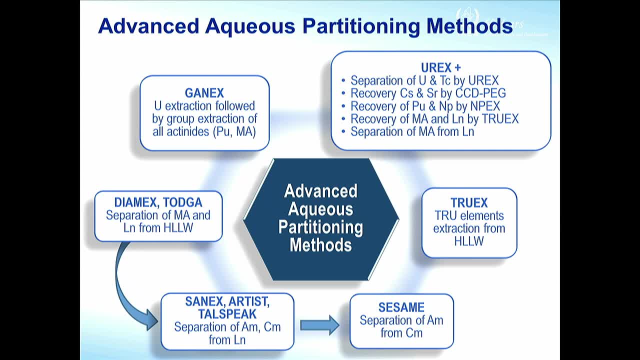 and they are very difficult to separate among them. And finally, there is a process dedicated to separate minor actinides from lactanides. This is the American approach. The American approach is to separate. once the bulk of uranium is separated, the plutonium is extracted. 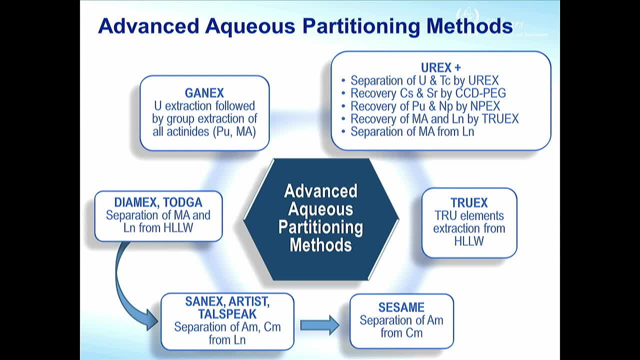 with the rest of minor actinides, and the process is called GANIX. it's the group actinide extraction. There is another approach, and it's the American approach in steps, So it's the so-called DIAMEX process. 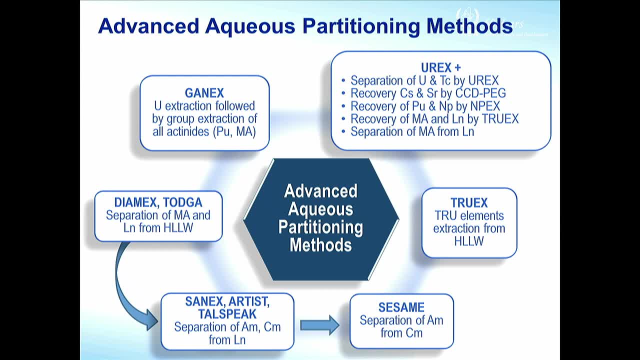 It's called DIAMEX because it's using bigly collamide and it's dedicated to separate minor actinides with lactanides from the high-level weights as the American process, And then, once we have minor actinides with the lactanides, 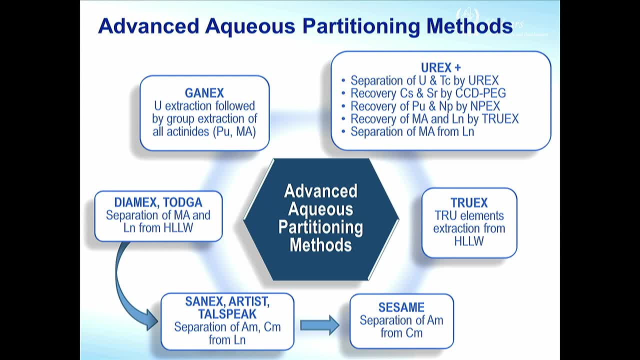 the separation between minor actinides and lactanides is done by using the SANEX process, the selective actinide extraction, using a dedicated molecule that is selective for actinides and not for lactanides. And then there is another process. 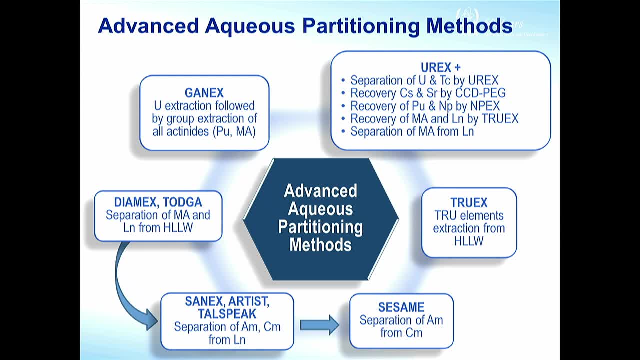 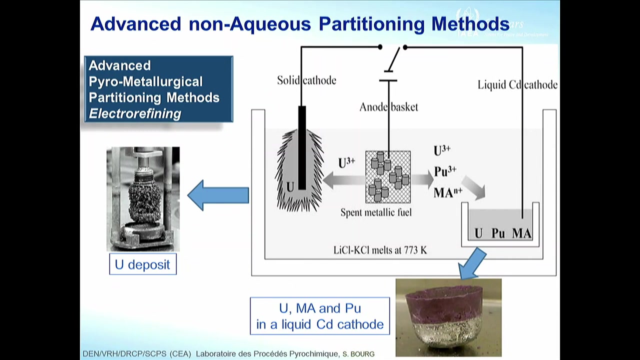 it's called SESAME to separate americium and corium to produce the blankets for transmutation. So all these processes have been tested at a pilot plant scale, but none of them have been already demonstrated at a commercial scale. This is the weight. 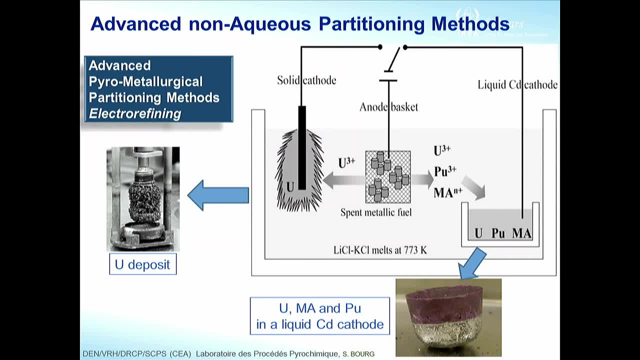 the weight methods and also there are understudied the dry methods that consist in dissolving the spent fuel in a molten salt bath, and it's called the electrorefining process, and using the difference between electroactivity between the elements, we can get a cathode. 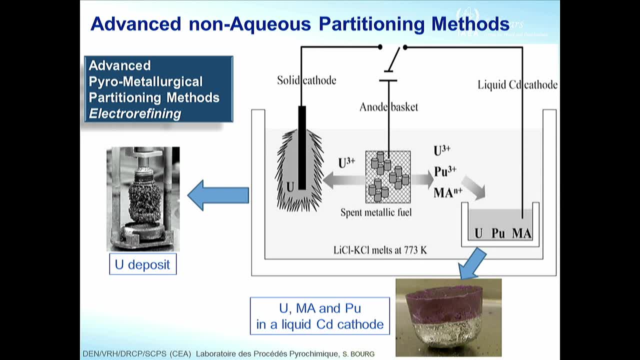 with the bulk of uranium and we can have a cathode, a liquid cathode with the rest of the minor actinides and plutonium and with some of uranium, And this is the real liquid cathode after the separation and this is the real uranium deposit. 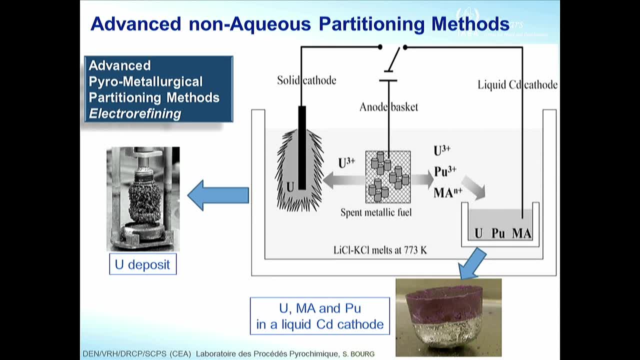 cathode with the uranium deposit. So these processes have been also tested at a pilot scale, but it's not commercially available. And in Korea they are working hard and they built a pilot plant to test the process in a cold test, not using radioactive material. 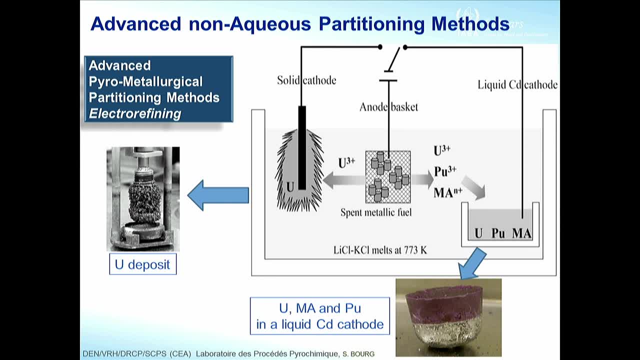 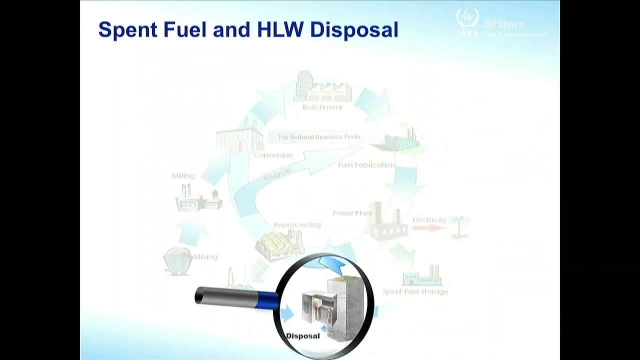 but using cold simulators to demonstrate the capability of this process to be at commercial scale. So this is the future And in any case, we need, at the end, a deep geological repository to dispose of the spent fuel or the high-level waste produced. 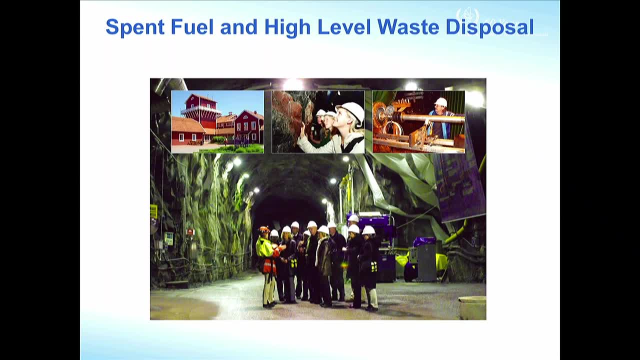 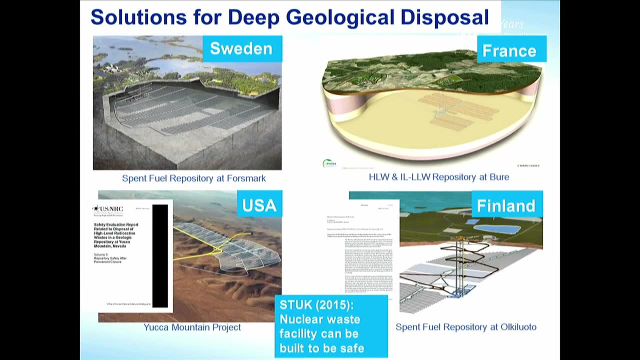 during the reprocessing activities. So this is a picture of a deep geological repository. And so far there are four countries in the development of the license step. So France has made a lot of effort to implement the industrialization of the industrial implementation. 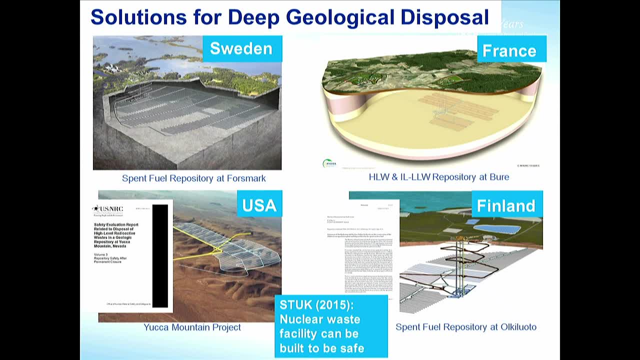 of the deep geological repository for high-level waste And they have an underground laboratory, and it's called CGO in the northeast part of France. Finland has submitted the license for the deep geological repository And they received in 2015 the positive feedback from the regulatory body. 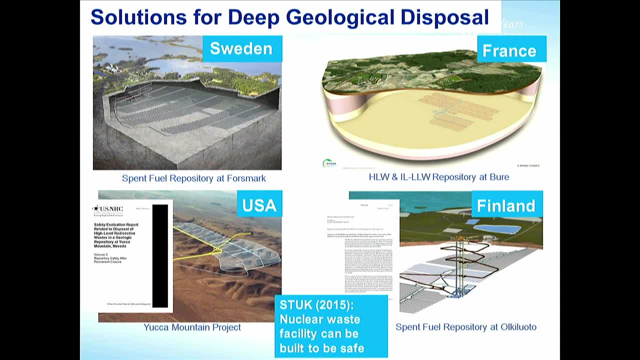 which says in a letter to the government, And they recommend to start the building of the facility under certain circumstances. So they are now building the deep geological repository And also Sweden has submitted the license, is in the licensing process And they don't have received. 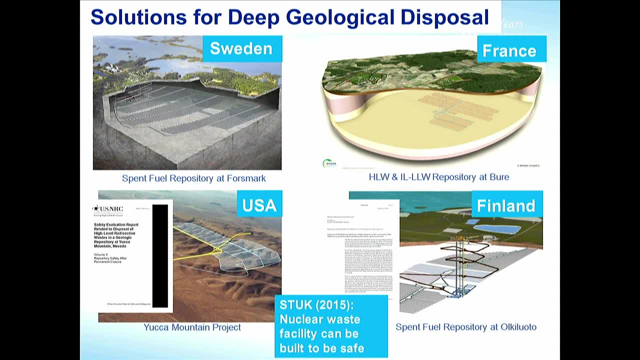 so far the final approval by the regulatory body. but they have some positive feedback and formal positive feedback And the unique ever-submitted license was in United States in 2008.. And the NRC, the staff, the regulatory body staff- shows their positive feedback. 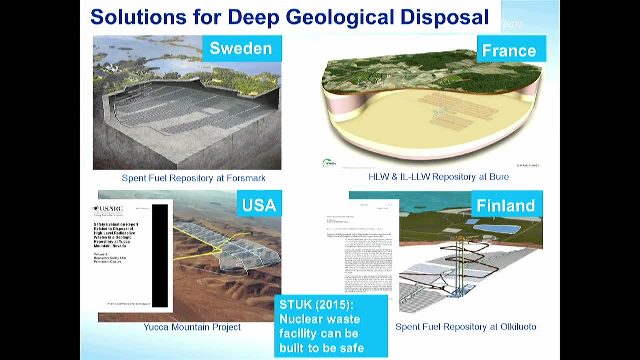 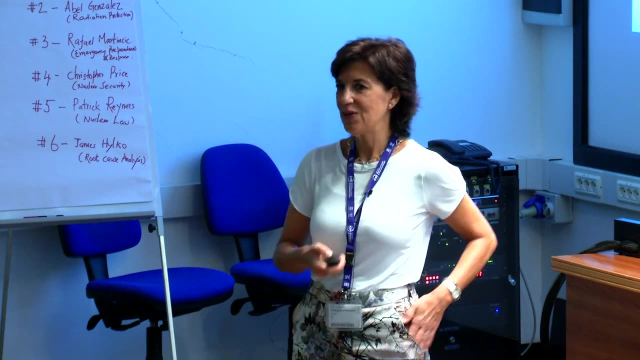 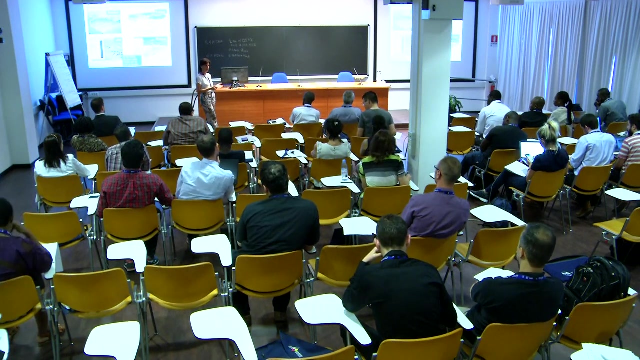 for the repository. But they found at the end some issues with the rights, the owner rights for the land and for the water. that stopped the project. And so it happened: the change of administrative administration. so Obama administration decided to stop the project. 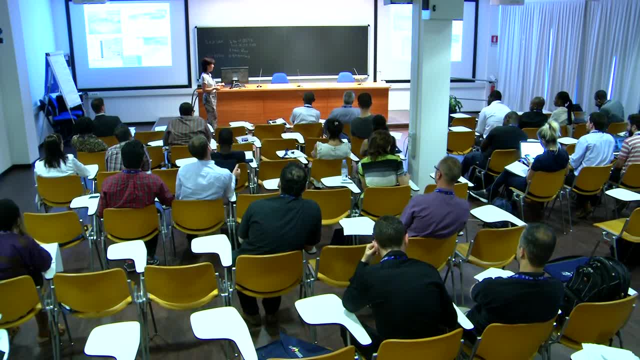 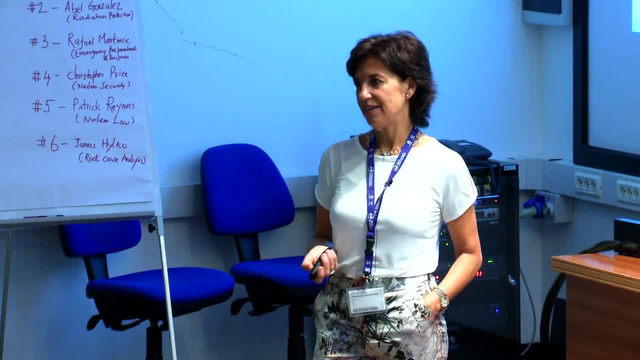 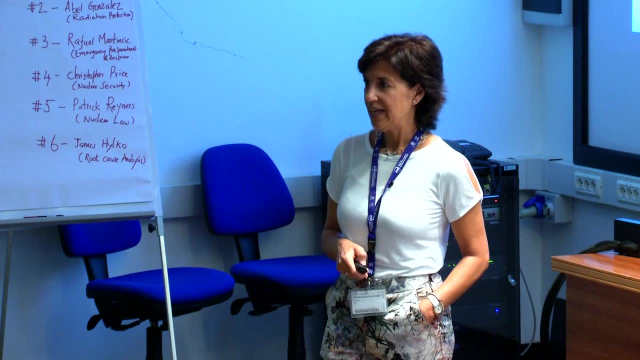 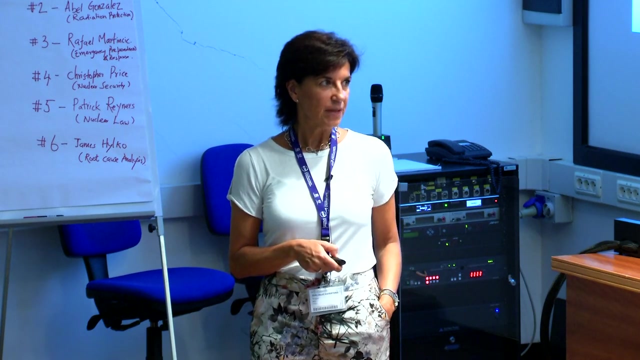 but not for the technical issues because the project was approved by the NRC, but was political and societal issues. So it shows that it's very important that stakeholder involvement from the beginning in this in all the nuclear energy development stages, but specifically in the sites.